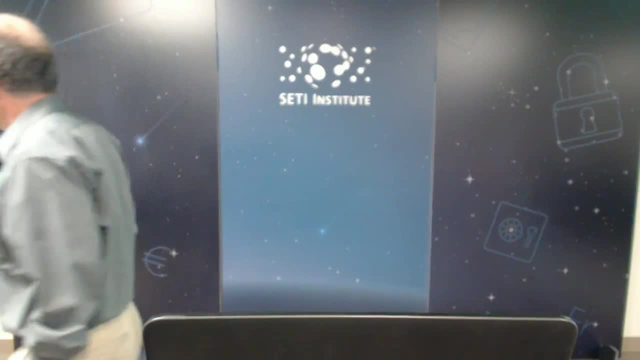 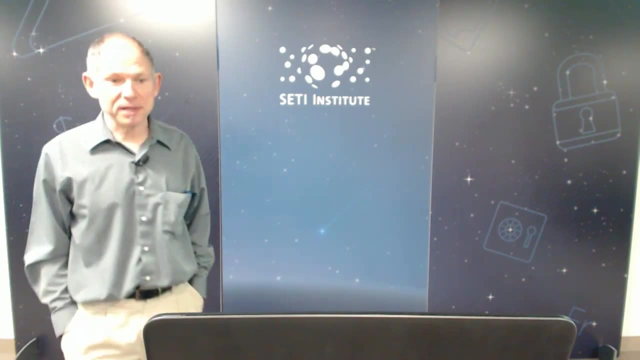 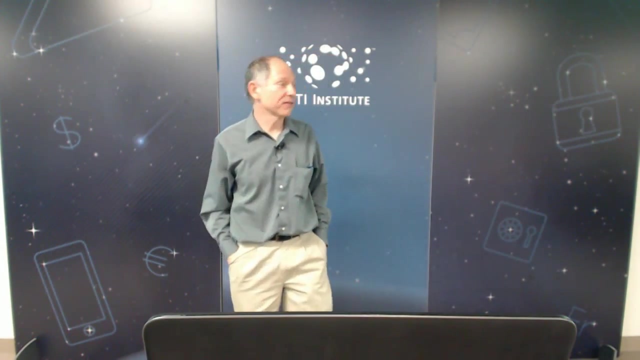 WFIRST is certainly in that category. You may have heard some of that. I'll give history in the next slide- but it's been changed recently and it's always been a mission focused on dark energy and also microlensing for finding planets. 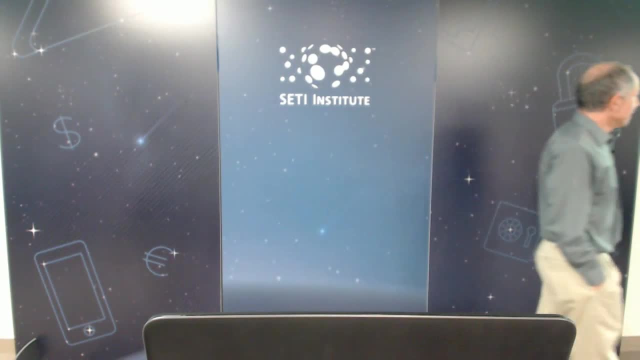 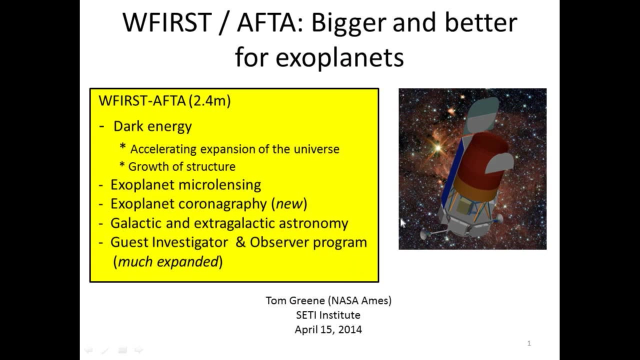 It's been complementary to Kepler, which I'll try to show. And this aspect about coronography is new. There's a new instrument for exoplanet coronography and also it has a much larger guest observer program. So larger than what? 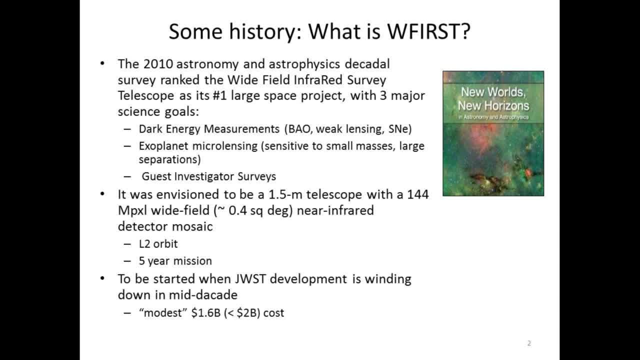 A lot of you probably haven't ever heard of this thing- So we didn't either when I was on the decadal committee- that every 10 years a bunch of people get together and decide what's best for astronomy and astrophysics. It's both ground and space. 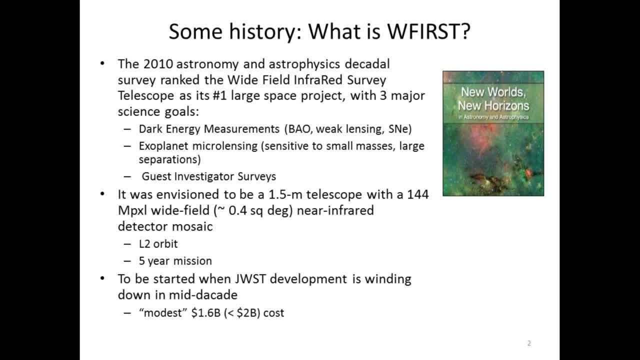 And I was on the panel that looked at space missions And we saw a number of proposals come in that looked quite compelling. There are people that wanted to use a moderate-sized space telescope for a number of different things: several different dark energy measurements. 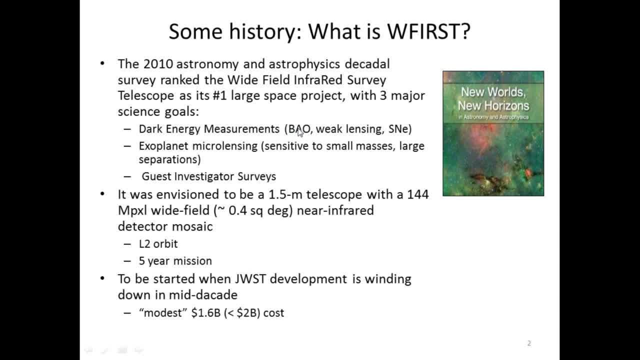 I'll get into these different ones. I hear you're going to have a talk on these baryonic acoustic oscillations later this month here Also weak lensing Supernovae. Supernova won the Nobel Prize, I think in 2011, with dark energy. 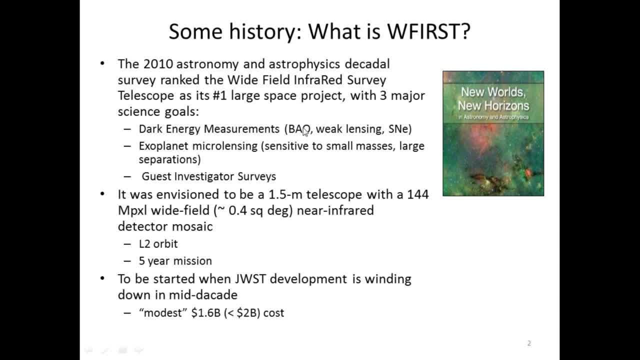 Then exoplanet microlensing, a new way of – there have been some detections with microlensing on Earth. Space could really open this up, similarly to what Kepler did for transit detections, And also a wide-field telescope would be great for a lot of surveys of the Milky Way, other galaxies. 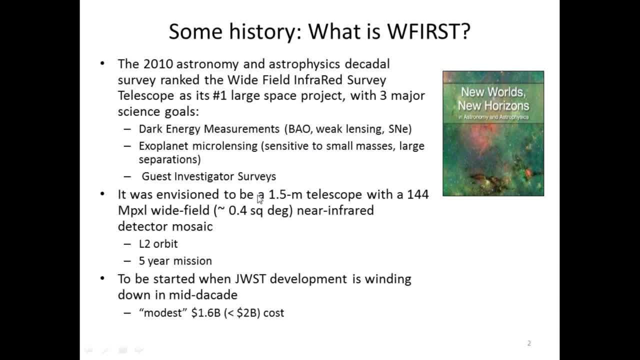 Then we thought about this. We thought that this could be pretty modest, like a 1.5-meter telescope, so about 5 feet in diameter, And much smaller than – like the James Webb we're building now, smaller than the Hubble Space Telescope. 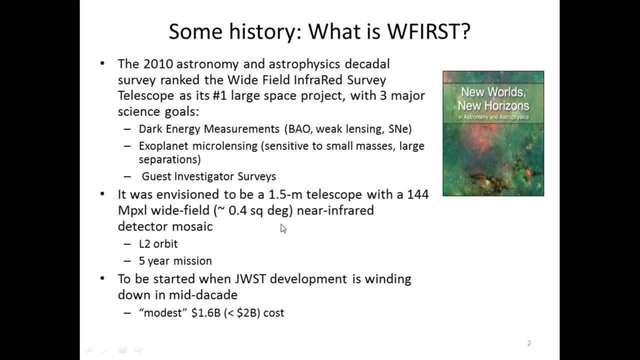 But have a lot of pixels over a very wide field, a couple tenths of a square degree. I'll show you how big that is in a bit. Then wanted to work in the near-infrared. Throw it out where there – it's a very popular spot these days, not in Earth orbit, but orbiting this point in the Earth-Sun system. 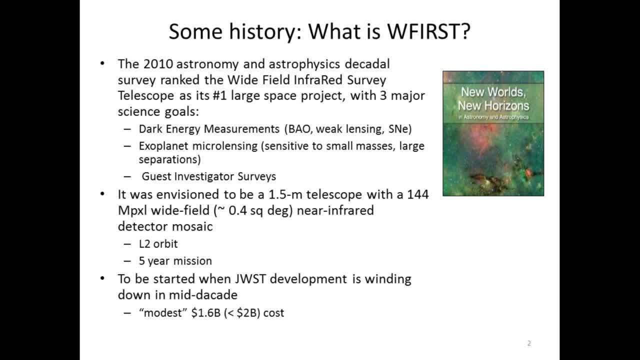 called L2.. It's about three or four times further than the Moon. It's a million miles away from here. A five-year mission, And the idea was is it should be affordable, where we'd have some of the funds that would be hopefully left over. 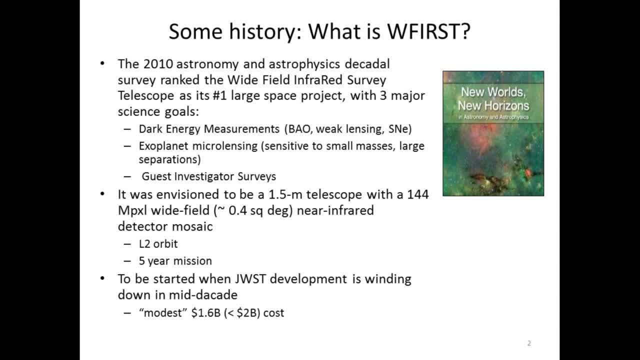 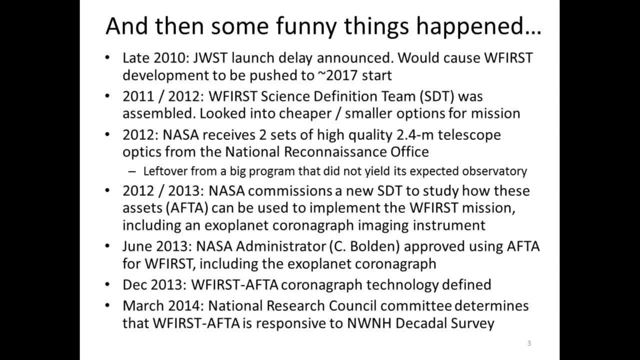 after the James Webb Space Telescope is winding down, And the whole thing would be maybe $2 million – $2 billion in cost. Well, a few things happened since then, Before we even issued our report, or about the time we issued our report. 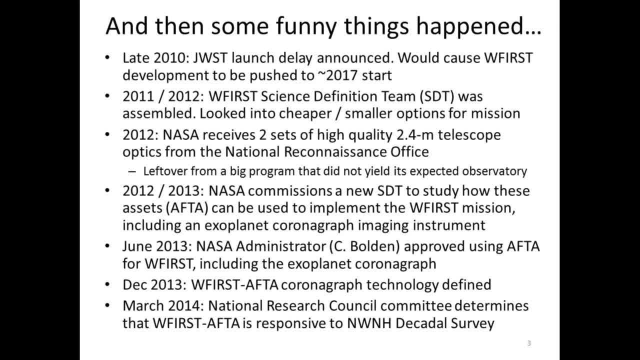 we got news that the James Webb wasn't in good shape programmatically. It needed more money and its launch was going to be delayed, which would delay any future observatory like this, like WFIRST. So a few science definition teams were formed to figure out what to do. 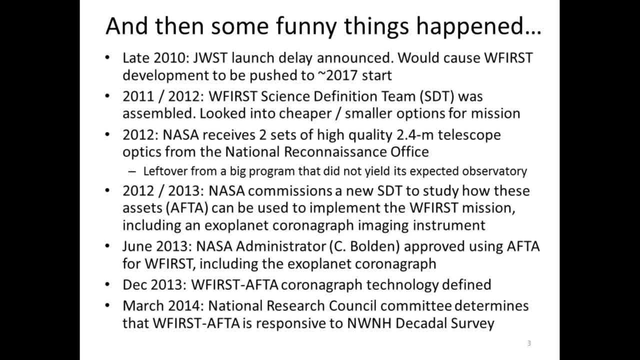 The first one formed to study what to do with the original WFIRST, and then another one looked into a cheaper and smaller version to see what could be done, scoped down and could still capture much of the science. And so everybody's kind of like mulling over, you know. 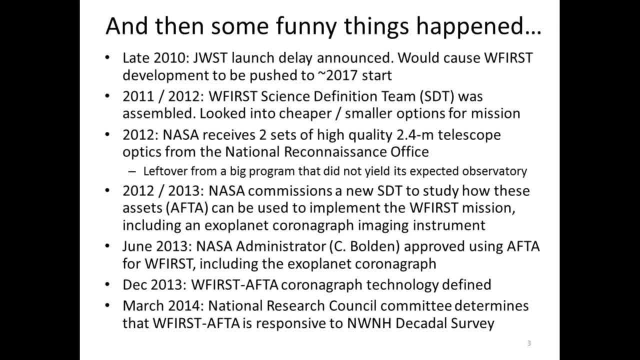 we're sort of like pretty glum about this. And then you may have heard, in the summer of 2012,, NASA was given some leftovers from another agency that just happened to be building a 2.4-meter space telescope the same size as the Hubble Space Telescope. 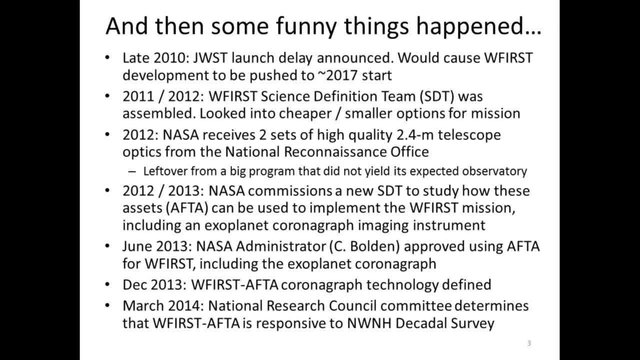 And no coincidence, the Hubble Space Telescope came sort of from the SPIE program. The National Reconnaissance Office builds them. NASA even operates these. We know that now. We didn't know that at the time Hubble was launched, Its existence was declassified in 1993.. 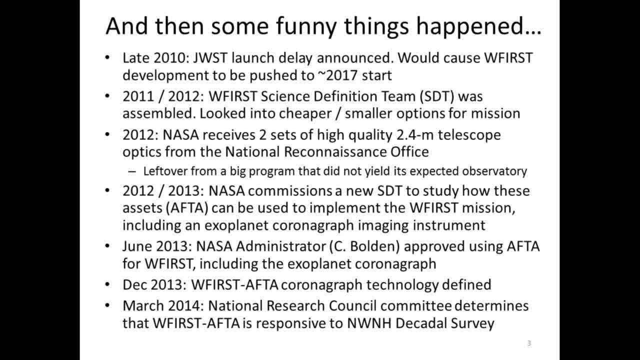 So we got two telescopes and then a new science team was put together to study whether these things are going to be useful for this WFIRST mission, And we put together a report. We found that, yeah, it turns out, you give us a bigger telescope. 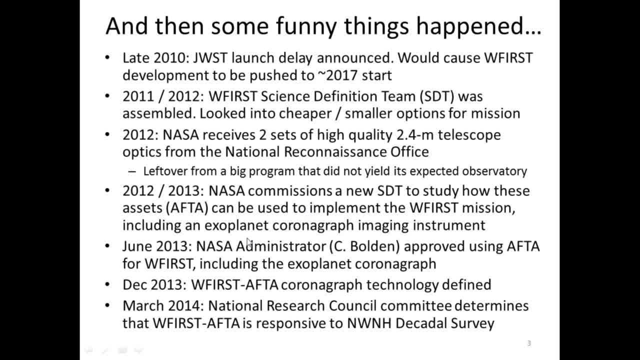 we can do more science with it, And the administrator of NASA got pretty excited about it and he approved using these telescopes for this purpose. By the way, when they were given to NASA, they were given to us for use in space science, but not looking down. 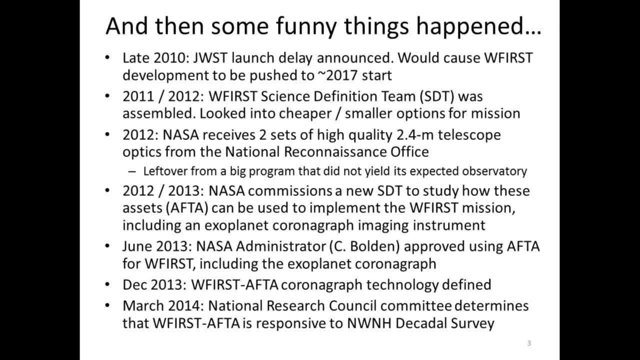 So it works for this application just fine. And then one part of this new formulation of it is that a new instrument was added to have a coronagraph to be able to blot out the light of nearby stars, to look for planets nearby. So we've been studying that too. 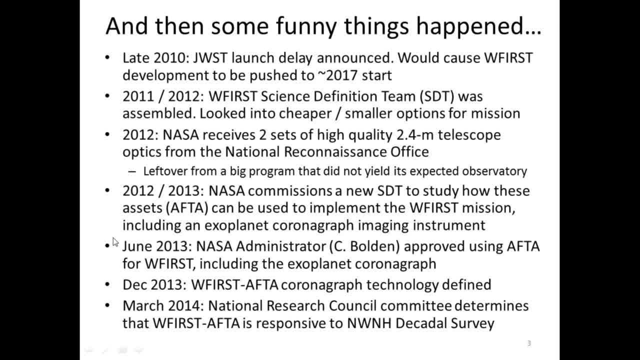 And it's not the ideal telescope for that, but we can do some pretty interesting stuff. So after we got approved to use this telescope, we went into a pretty mad technical program led by JPL where they defined the particular coronagraph technology. There were about six competing technologies. 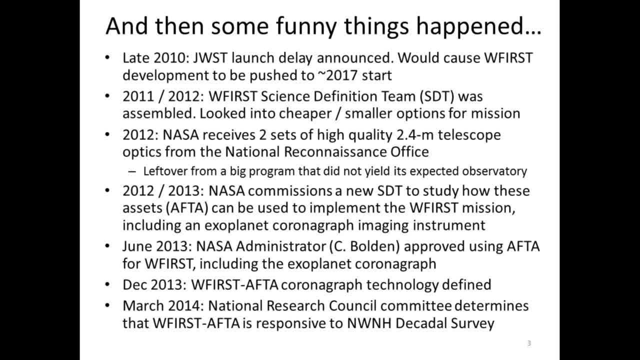 and we did a lot of studies and simulations to figure out which ones would actually have a reasonable chance of working well with this telescope, and narrowed it down to two or three, depending on how you look at it, And then also reviewed recently by the National Research Council. 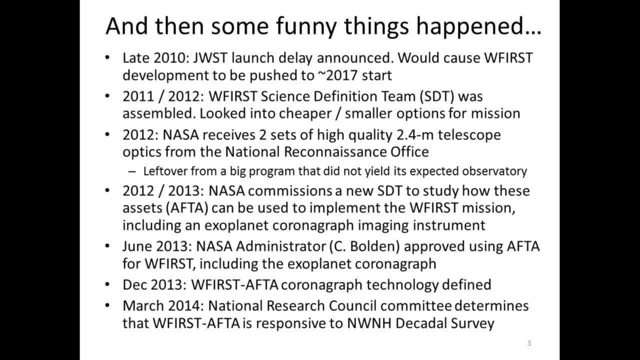 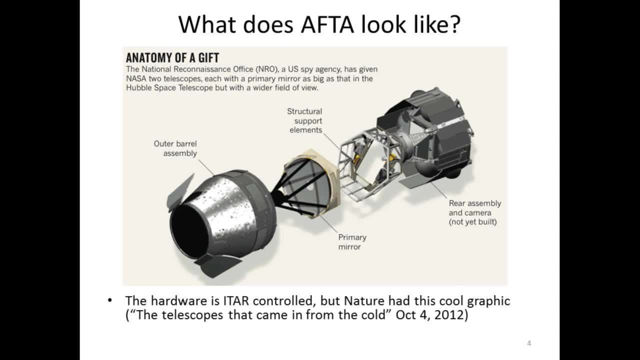 they had a committee to see whether this new thing stays true to what the Decadal Survey wanted the mission to do. And we got an endorsement from them, but also a warning saying: keep the cost within the box. So what does this new telescope look like? 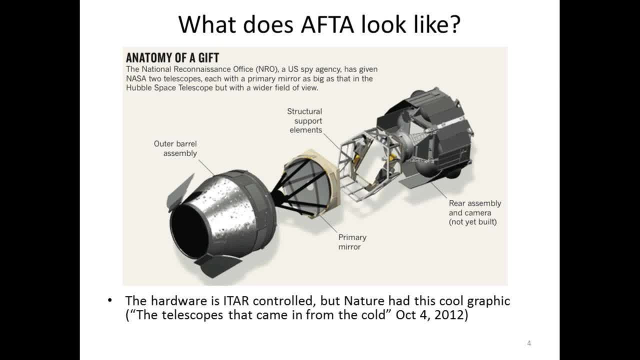 Well, I think I've only seen one real part of it. I saw a picture of it, and then that was restricted to US persons because of its genealogy. It's a controlled item, But this was a picture of it from Nature magazine. 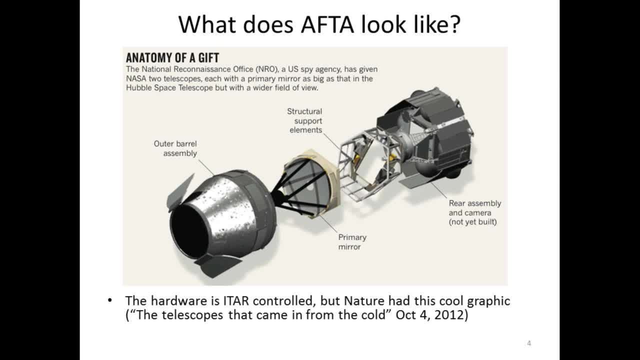 sort of showing how these things work. So I would say, this mirror here is 2.4 meters, like about 100 inches, the same size as the Hubble, and came with this baffle- The baffle we'll probably not use. 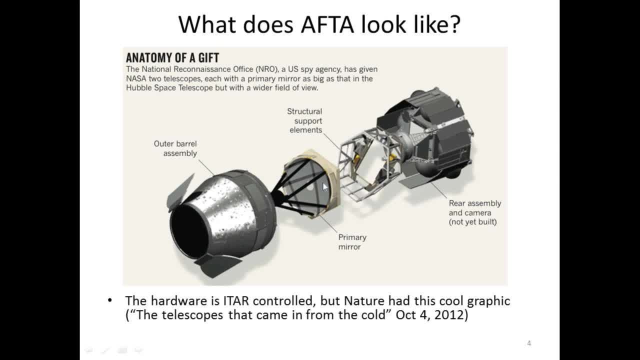 but we will use the secondary supports and the secondary mirror there and we'll put some other stuff on the back of it. The question is, why is the baffle there? And I assume something like that, but there's also got to be like a scan mirror to point down at the Earth. 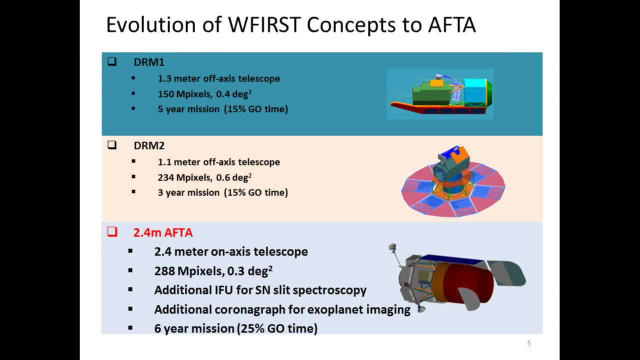 We have different baffling because it's going to be in a different orbit. These are sort of the cartoon versions of a few of the different versions of this observatory. This first one was the one DRM-1, is sort of DRM stands for Design Reference Mission. 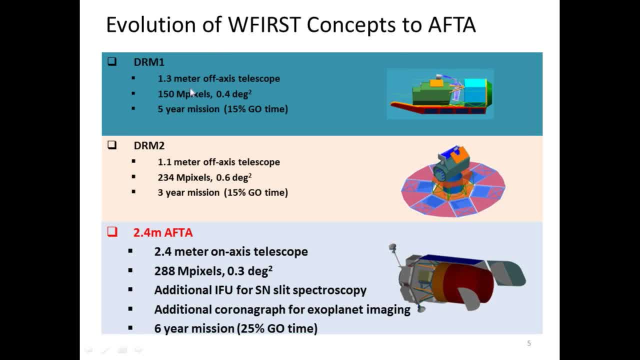 put together to pretty much follow what we had recommended in the decadal survey. They made the telescope a little smaller because they didn't have a hole in the middle, so they're able to get better images. And then, once we found out how the James Webb was going to be late and cost more. 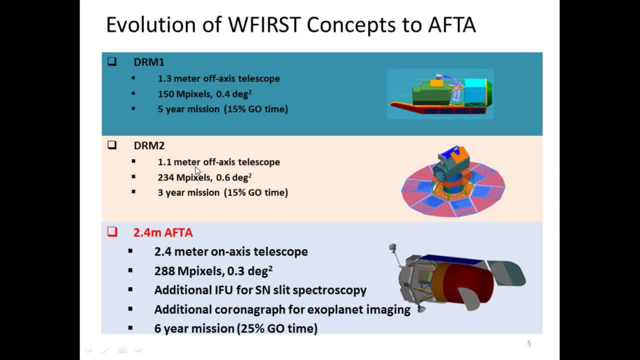 we tried to do something cheaper, so we made the telescope smaller still And then had more pixels in the detectors, but actually fewer detectors by making the pixels smaller Then now this is what we have: a 2.4 meter telescope and a lot of pixels. 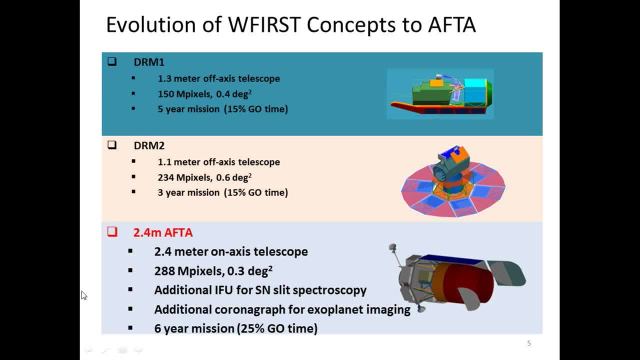 They have 18 detectors in the wide field camera. Each one is 4,000 by 4,000 pixels, so you end up with 300 million pixels. It's a big camera. There's a little integral field spectrograph for supernovae. 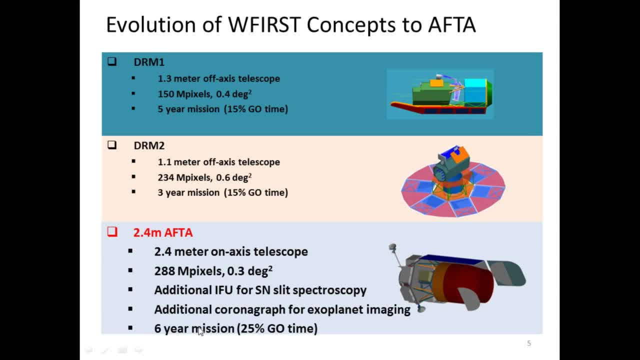 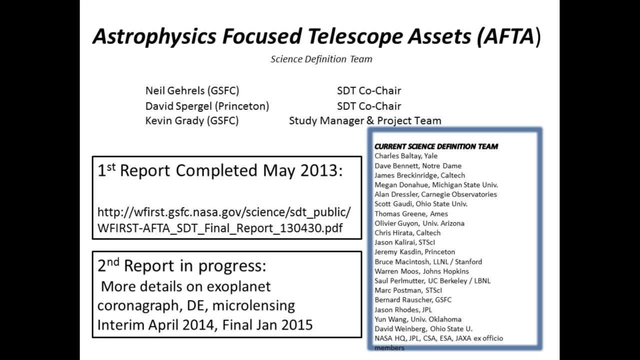 and we've got the chronograph instrument and looking at a six-year mission. So it has gotten bigger. This is what the science definition team is doing. We do have a report on this. first, look at this 2.4 meter. It's on the web on this NASA Goddard site here. 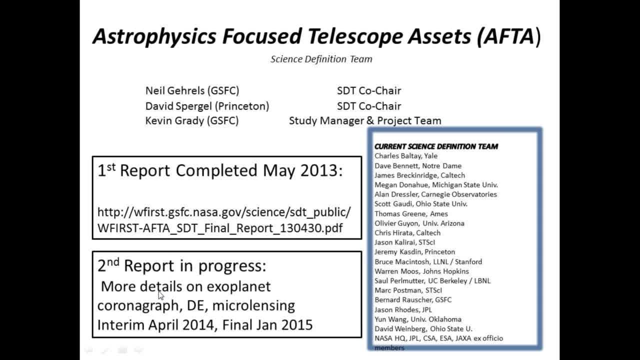 And we're working on a second one. We have an interim report this month and a final one in January of next year. We're really looking at a lot more details, More work being done on the project. We've refined the chronograph technology. 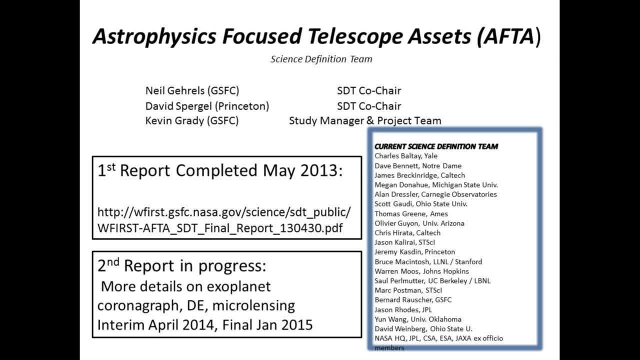 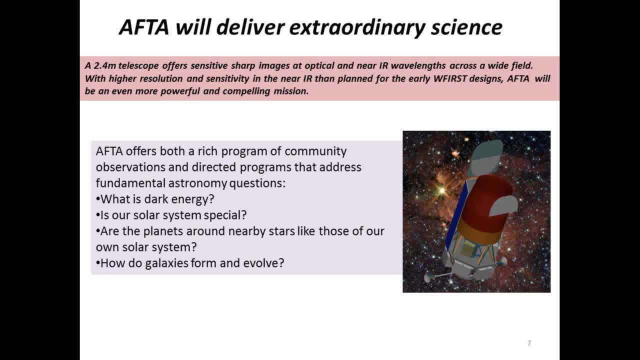 We're getting much more specific about what science this thing is likely to do, So we think it's going to do great science. That's what kind of science it's going to do And I'll get into it a little bit. It's going to stay true to the decadal surveys charge. 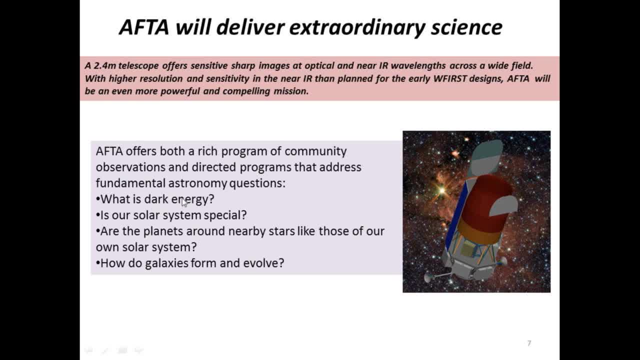 to figure out what is dark energy. It has three different programs for that. Demographics of planets. Kepler has shown that most planets that it's seen are nothing like what we have in the solar system. It's like there's this huge population of planets. 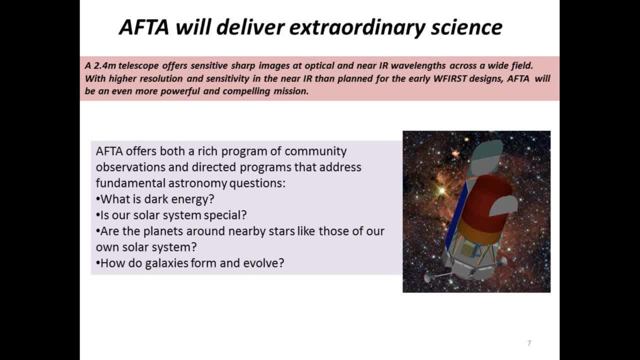 between the size of Earth and Neptune that Kepler has found, that we just don't have here. So let's see what else is out there, And also studying really nearby planets and what their planetary systems are like, what their distances are like, and also galactic structure and evolution. 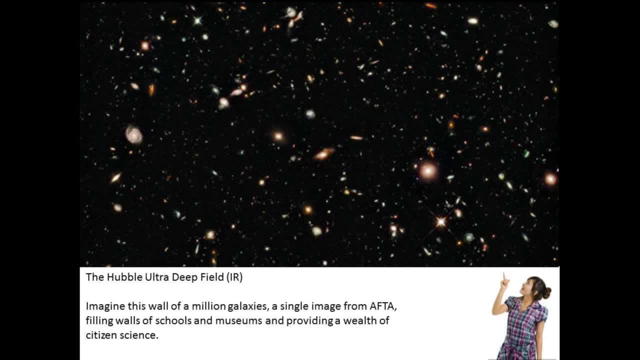 So how is it going to do all this? Well, this wide field stuff is pretty interesting. You may have heard- you're going to hear- talk about it. this really wide field camera called BOSS And Kepler was a pretty wide field instrument. 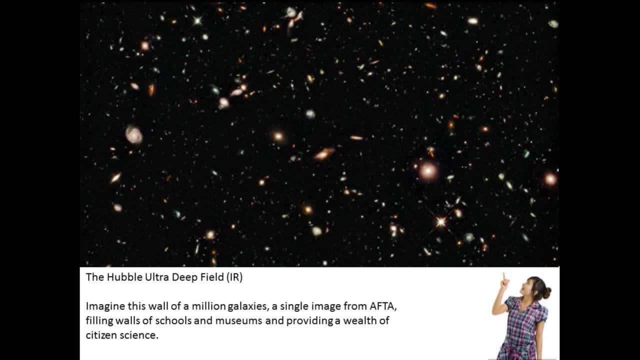 It was like 100 square degrees, which is huge to stare at all the time. So if you look at more parts of space, you'll learn more things. This is an image of the ultra deep field taken with the Hubble Space Telescope. about 10 days of integration time put together there. 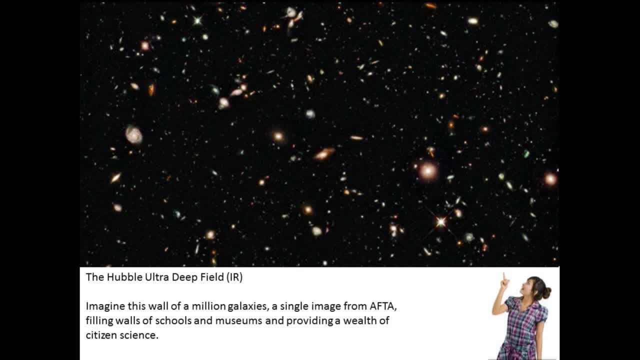 That's about the field that the Hubble Space Telescope and Hubble sees, And you can see galaxies going quite far back to only like a few hundred million years after the Big Bang. So to get statistics on these you want to look at a lot. 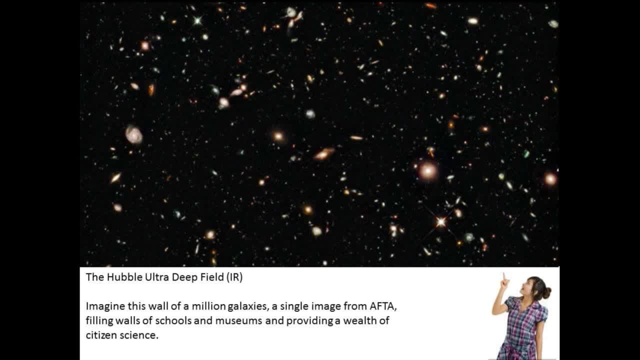 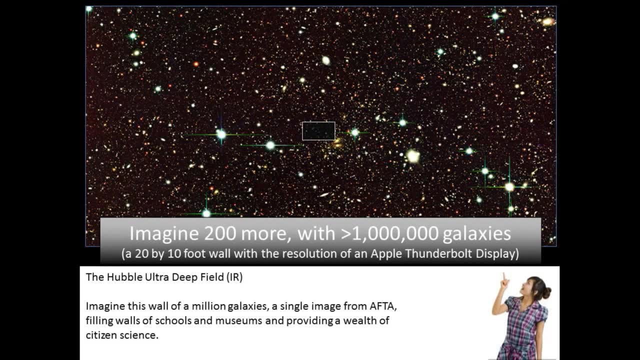 However, if it takes 10 days for single pointing, you're not going to be able to look at many fields. So what if you had a field that was bigger than that, Like maybe 200 times bigger? So that's what AFTA is going to do. 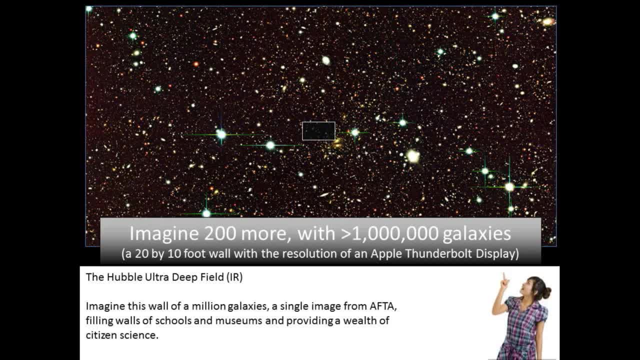 It's going to deliver Hubble Space Telescope sensitivity and spatial resolution over a field that's over 200 times bigger. That's the increment that the wide field camera does, And this has pretty much been enabled by detector technology that has been developed for the ground and also for the James Webb Space Telescope. 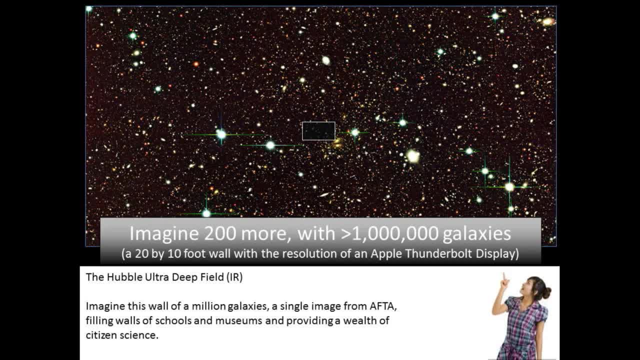 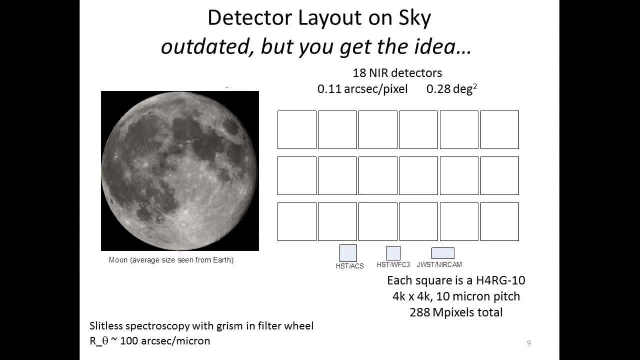 Oh, these are near infrared: 1 to 2 microns. primarily That was the question. what was the wavelength? So this is just another picture. A lot of people don't like this one, but I like it. It sort of shows the field of view. 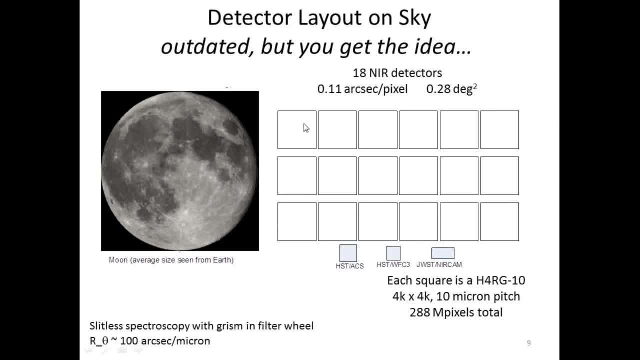 These are the focal plane. It's been changed a little bit to be a little more curved to take advantage of the best image quality. This is the size of the moon, So if you saw the lunar eclipse last night, it would only take maybe a couple fields. 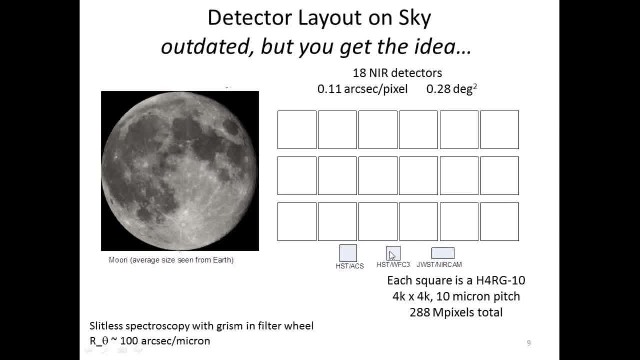 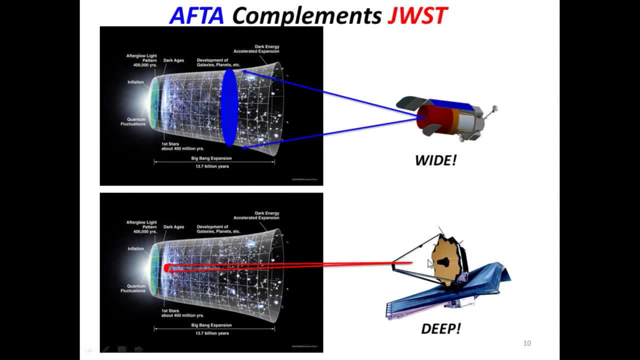 to get the whole full moon. And then this is the size of the equivalent camera on Hubble and this is the size of the equivalent camera on James Webb. No, no, this has grisms and it has prisms. I'll talk a little bit about the instrumentation in a bit. 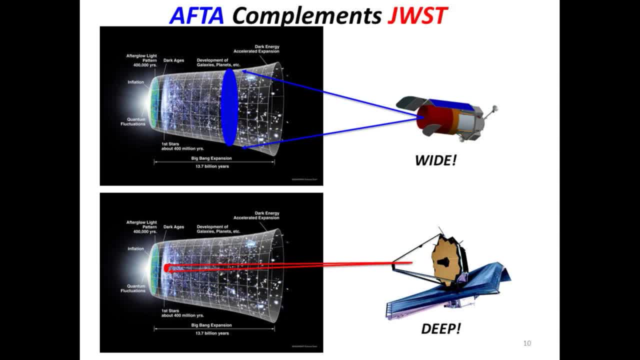 This shows complementarity with James Webb. James Webb is something that we're building now and we're going to launch this in 2018.. It's a huge telescope: 6.5 meters in diameter, 25 square meters of area. 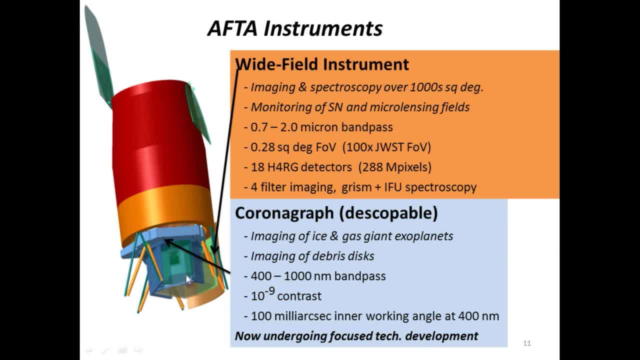 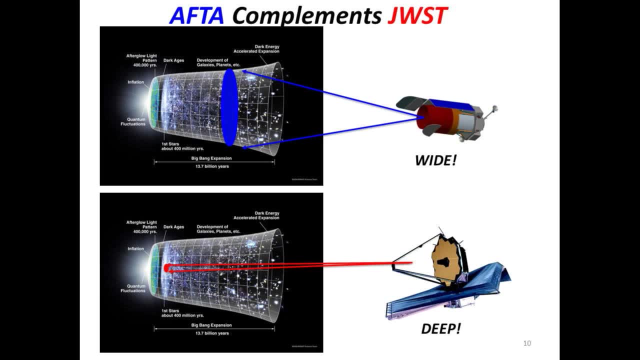 It's going to see the very first objects that lit up the universe after the Big Bang, But it's not going to see. it's not going to see a big field. We didn't have a lot of detectors at the time and we had to make this advance. 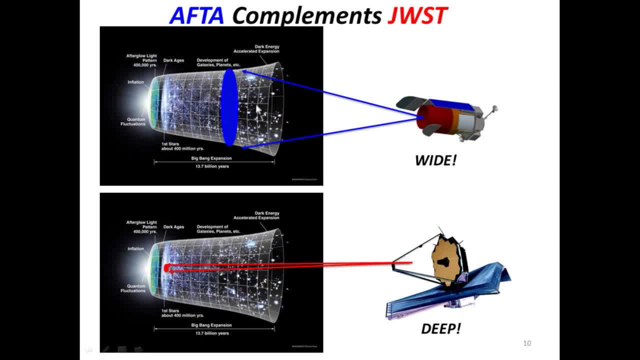 So now, what AFTA is going to see, though, is going to be a much bigger area of closer things. We will probably find a bunch of stuff that's of interest to James Webb. They should be flying at the same time, So it'll be able to survey a much larger fraction of the sky. 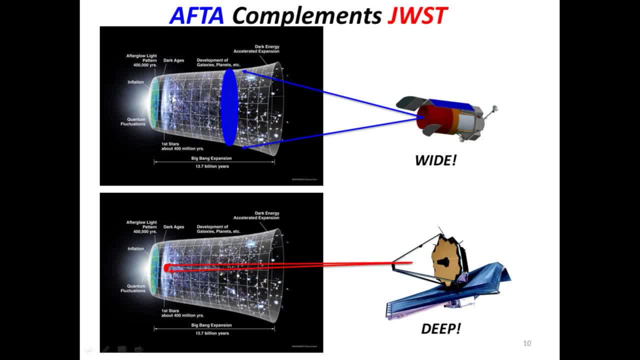 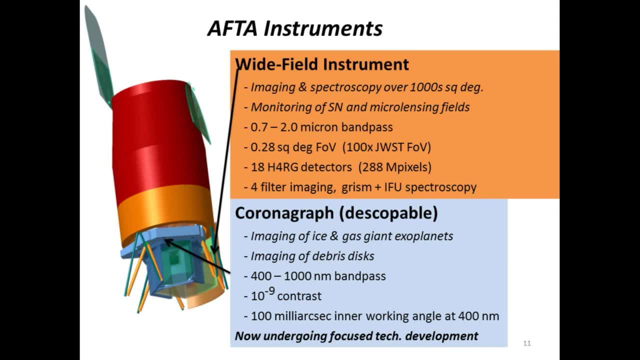 not as deep, not as far back towards the Big Bang, which is over on this side, but be able to see things down to about 10% of the age of the universe. So, in addition to having this really big field instrument, that's, this 288 millions of pixels, 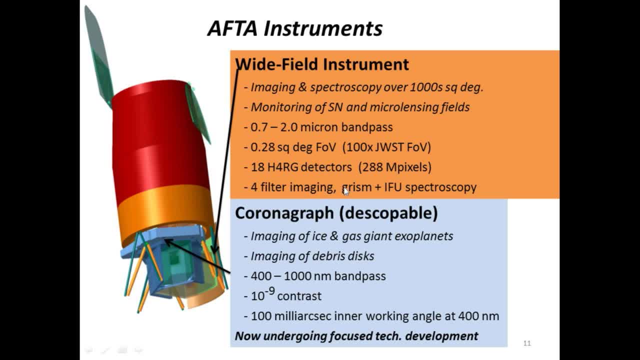 there's also going to be a grism which does spectroscopy. You'll be able to get to a spectrum of every point in the field And a separate spectrograph. you can put individuals like supernovae, to figure out their velocities. 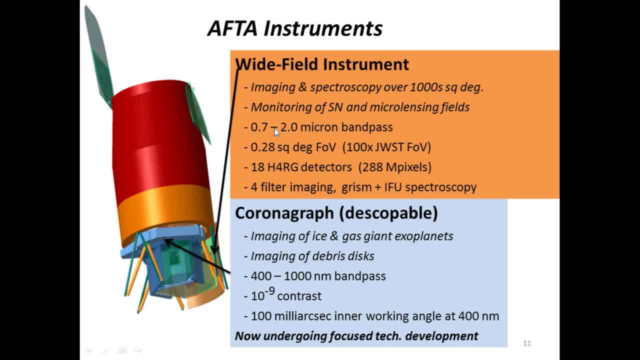 This is the wavelength range over which it'll work: from very red- just as red as the eye can see out- to a few times that wavelength. Then there's a coronagraph instrument here. It's a very different beast from the one above. 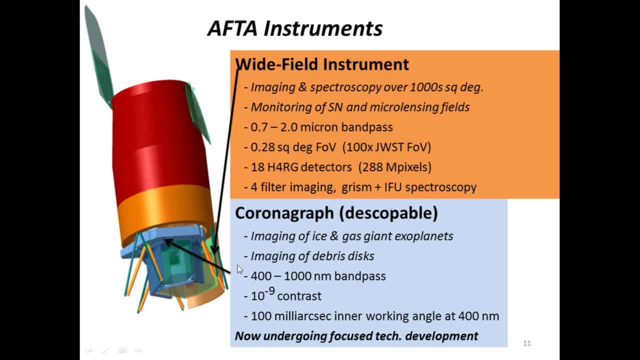 It looks at a very small area with very good spatial sampling and we try to blot out the star. So we'll look at the very closest stars to the sun- things within 10 parsecs or 30-some light years- and we'll try to blot the stars out. 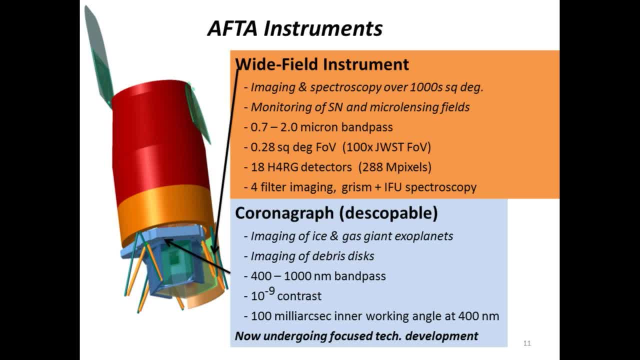 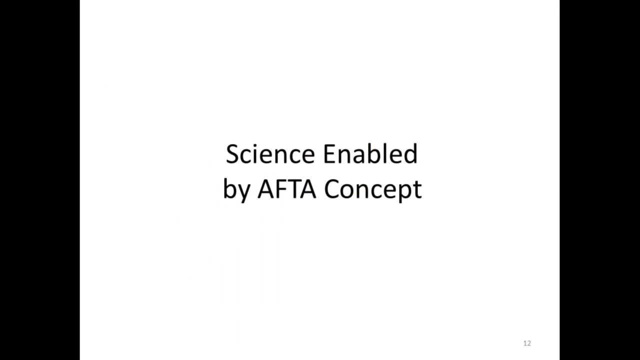 look for their planetary systems very nearby And we'll try to show some examples of what we think that will do. And this is really undergoing some focused technology development. now Science. I kind of like this picture. It sort of sums up what we think. 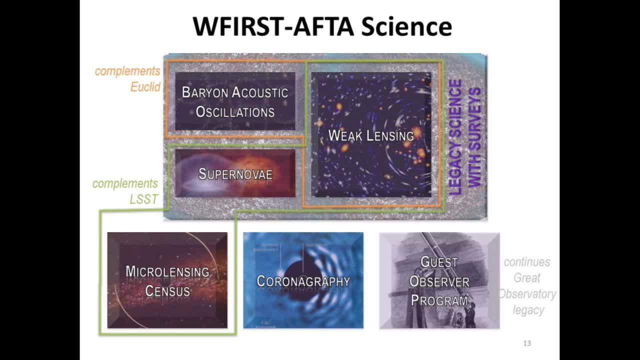 the big science pillars are. This whole top rectangle is all the dark energy. It's going to be these three different surveys that we're going to try to get after. this question is: what is dark energy in different ways? Baryon: acoustic oscillations were around. 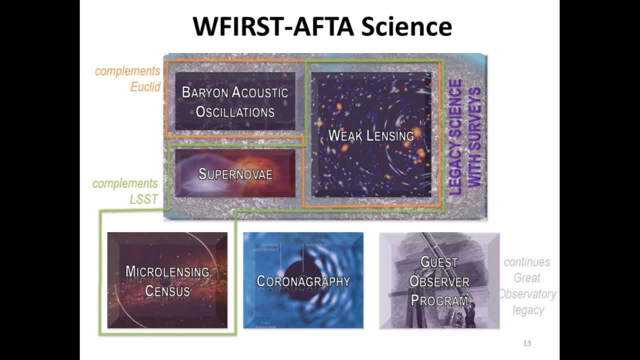 probably right after the Big Bang, and these are just sort of compressions in matter that have propagated from the Big Bang into clusters of galaxies. today It gives a size scale of the universe. We're going to look at how that changes in time. 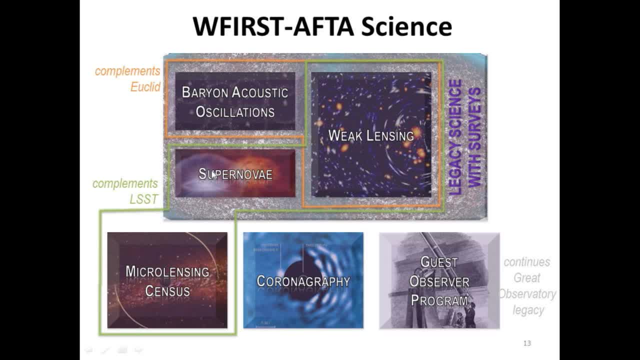 Then supernovae again is what won the Nobel Prize. So by looking they're all about the same brightness, or people think they are. So by measuring the brightness you know how far away they are, and then you measure the velocity of the spectrograph. 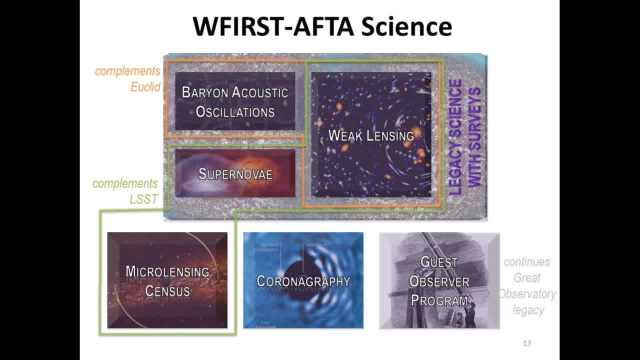 and then you see how the universe is changing its expansion rate And weak lensing probes matter. So I don't know if I've got another slide of that, but we see an example of strong lensing right here on the SETI sign. 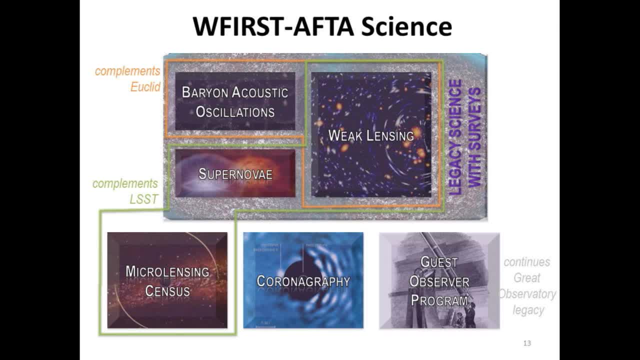 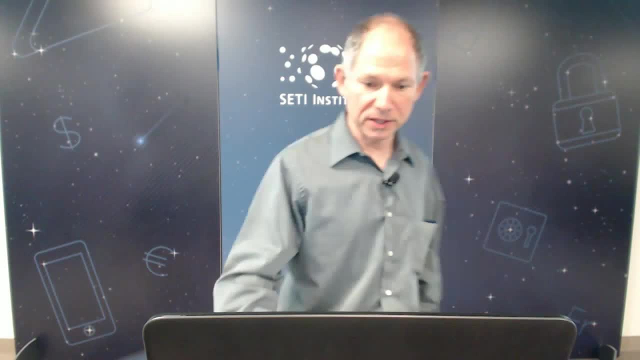 These galaxies in the background are being magnified by some mass in front of them, So it's very sensitive to both dark and luminous matter. Then we'll be doing planetary microlensing. I'll give an example of that: This coronography that I told you about in the middle. 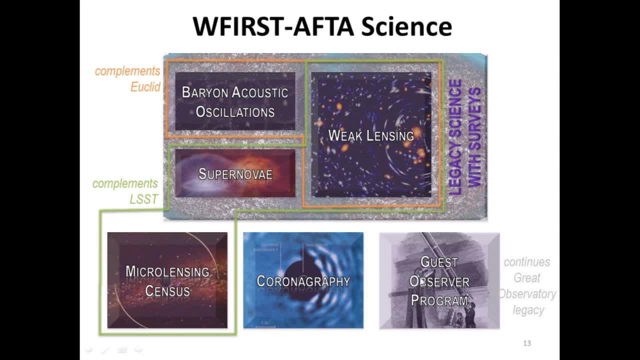 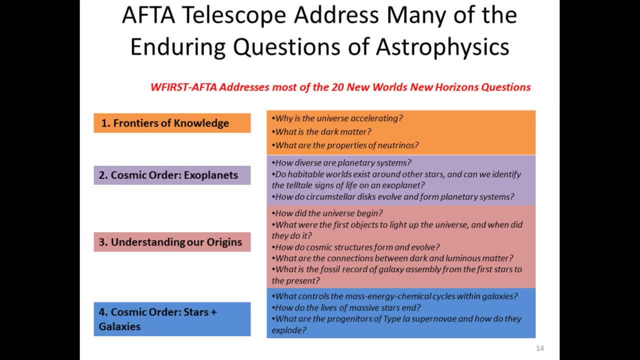 is where the star is blotted out, and these are, so we can see planets nearby. And there are a lot of smart people that will want to use this thing for a lot of different programs, just because of the field. I'll give a few examples. 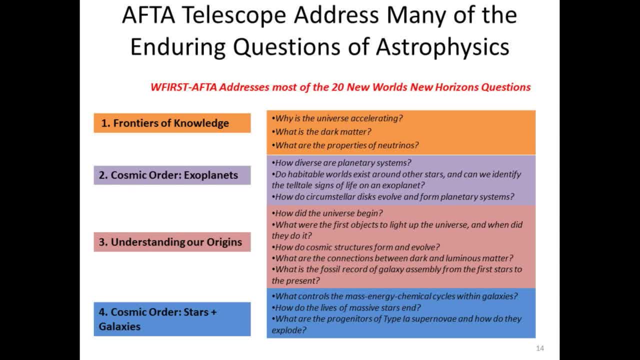 The decadal survey came up with about 20 questions. I wonder if we did that intentionally. So it's like the game of 20 questions, 20 questions of science for this decade. This mission seems to address 14 or 17 of them. 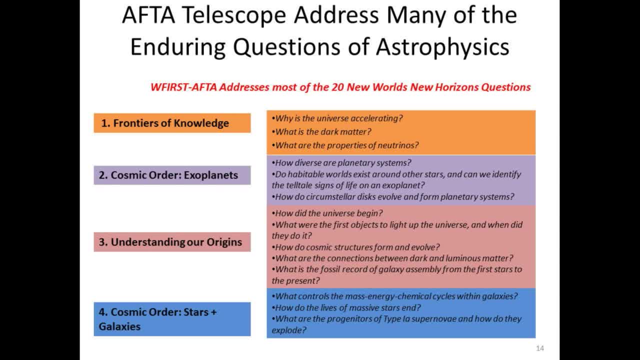 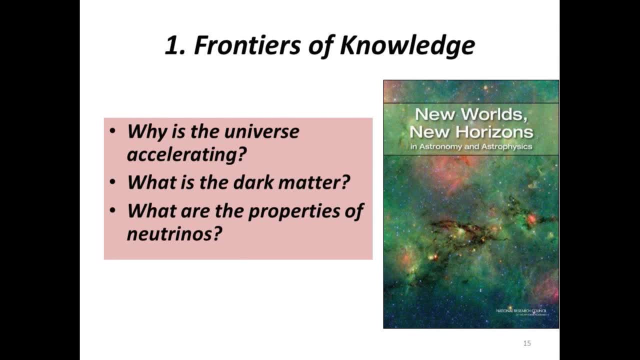 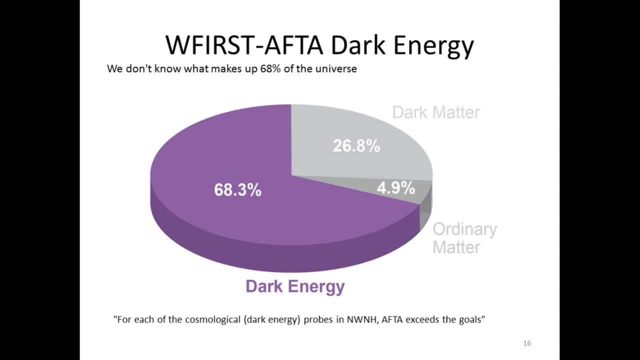 depending on how optimistic you are and how you do the counting. So we think that this observatory really will do the science that we hope for in this decade: Getting into the dark energy science. So you know one of the things we've learned. 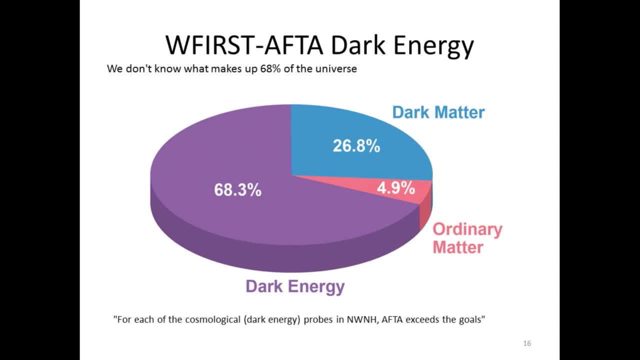 in the last decade is that the more. I guess one of the things we've known for a while is: the more we know, the less we know. right, And we've just learned it, in particular in this case with this dark energy, because now we know there's like 70%. 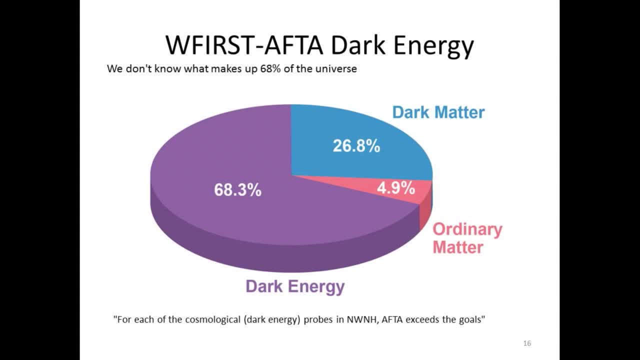 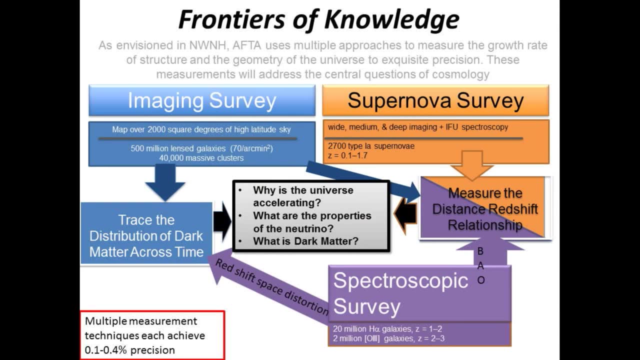 of the mass energy of the universe that we just don't understand at all, And so let's see how we can get at that. So there are going to be three surveys with AFTA that will get at this issue. So this is this imaging survey. 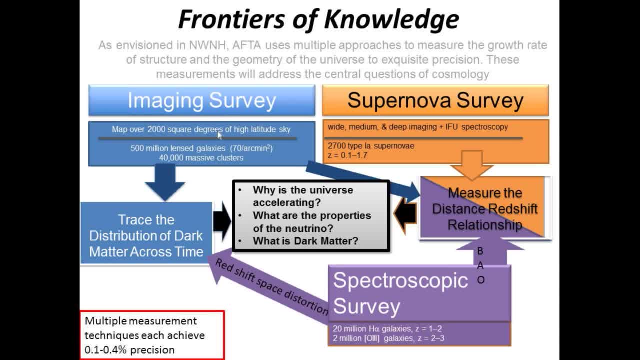 This is going to look at about 2,000 square degrees, which is about 5% of the sky. So it's going to spend, oh, something like over a year getting this survey And 500 million galaxies. So this is what's going to be: looking for perturbations. 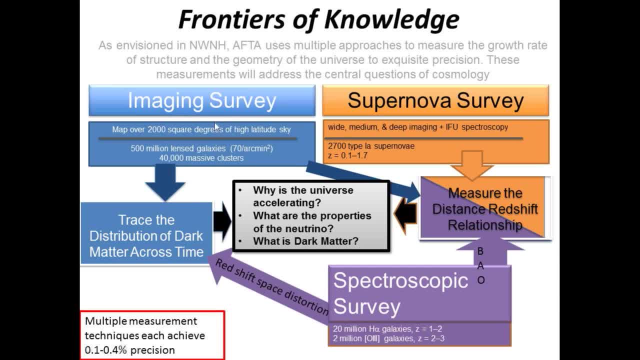 and shapes of galaxies due to matter in front of it. So this will map out the distribution of matter in the universe. Then supernovae- same technique again that won the Nobel Prize, being able to measure the velocities and brightnesses of supernovae. 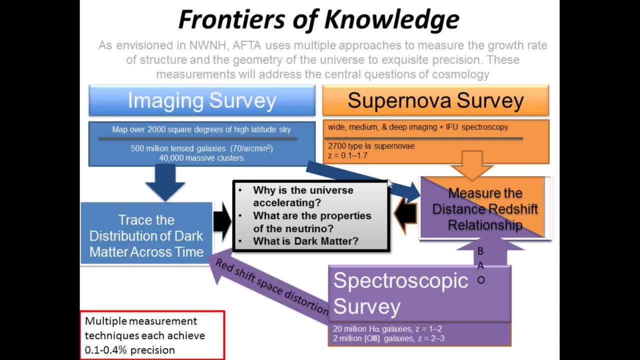 to look at how the universe is expanding. Then also the spectroscopic survey uses these baryon acoustic oscillations. This has a known size scale, so that it's actually sort of absolutely calibrated. These other ones are more this one's relatively calibrated. 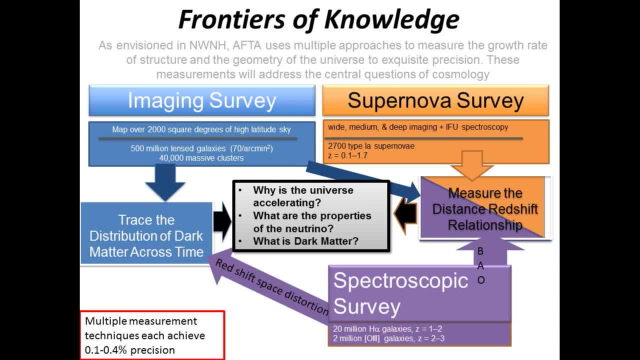 So these three tend to cross-calibrate each other and reduce systematic errors, So hopefully we can. we're going to hone in then on what the equation of state is of the dark energy. I'm not going to talk about that too much because I want to focus more on planets in this talk. 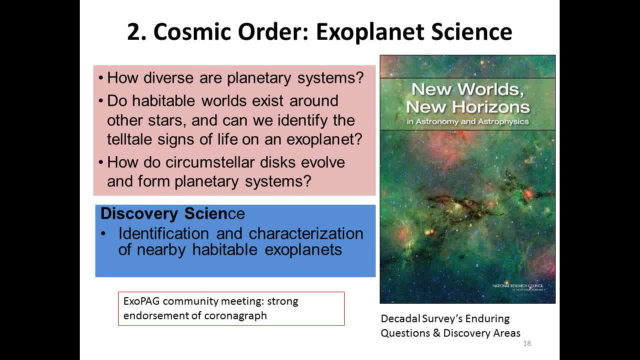 And that's also one of the big changes for this mission, So one of the big other big focus areas. you know, in astronomy for the last 15, 20 years the big things have been dark energy and planets. So we still don't know a lot. 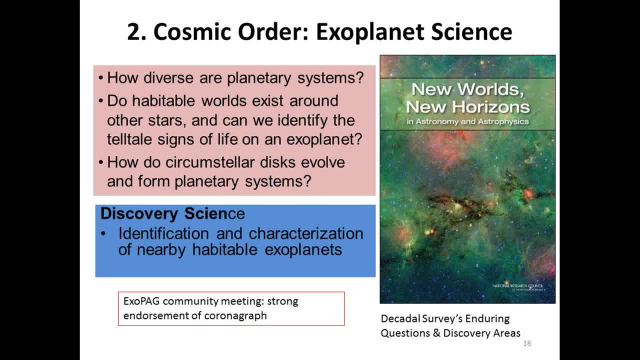 Kepler has really helped us understand diversity of planetary systems. There's this whole new class of planets I mentioned that we didn't know about. that we know is common. However, Kepler only probes planets pretty close to their stars just by the technique that it uses. 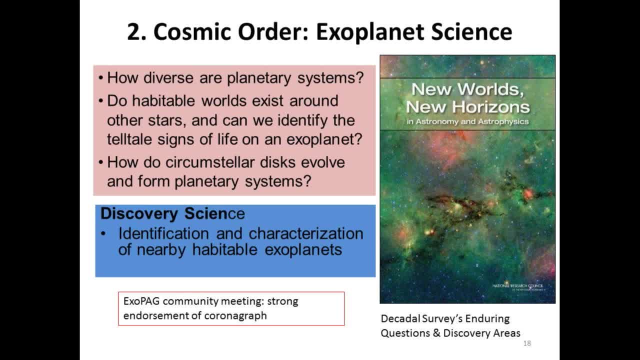 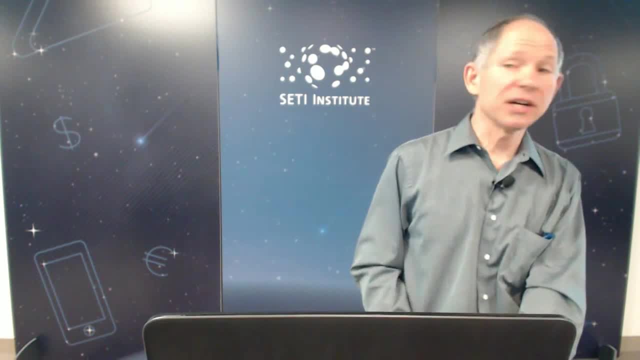 We also don't know much about circumstellar disks around planets. things like that's in our own solar system And we'll need to know more about those if we want to study and search for Earths in the future, because if the stars have a lot of dust around them, 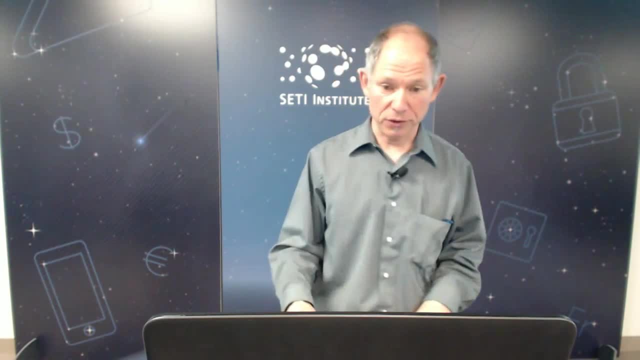 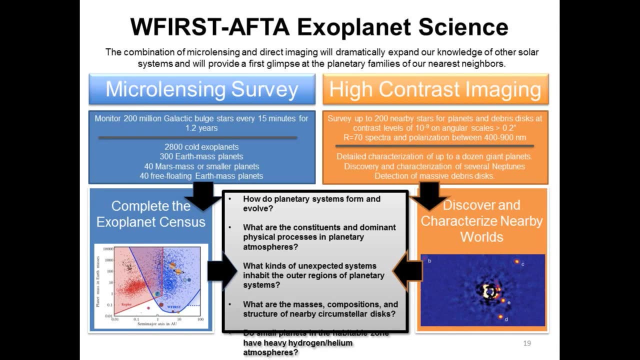 it could really blot out and obscure any kind of imaging of Earths. So we've got a survey- believe it or not- to do for the exoplanets and also some pointed observations as well. So for this microlensing survey we want to spend six periods of two months each. 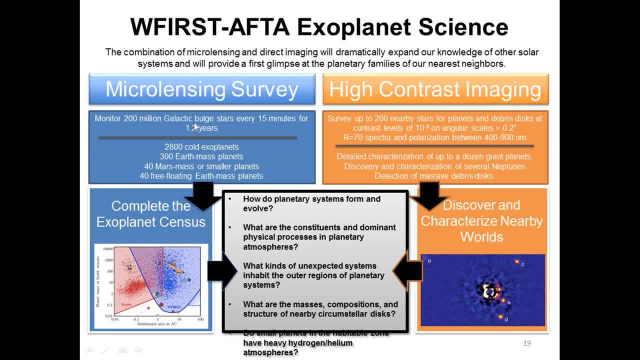 looking at these different fields towards the center of the galaxy And we think we'll be able to get about 3,000 new planet discoveries, very similar to the number of Kepler candidates. I think I've got another slide that shows the complementarity. 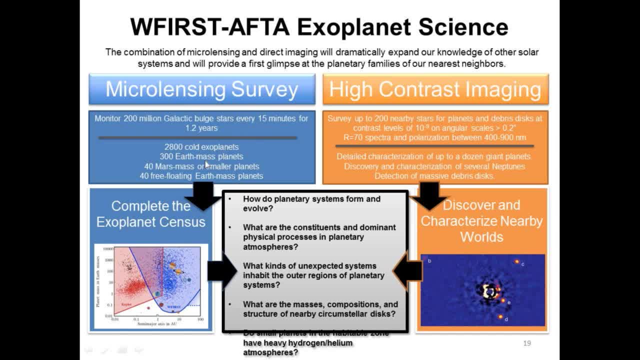 So this will be the statistical side. It'll be sensitive to low-mass planets and planets far from their stars. Those are two things that are orthogonal to Kepler, so it should be much more of a less-bias survey when you put them together. 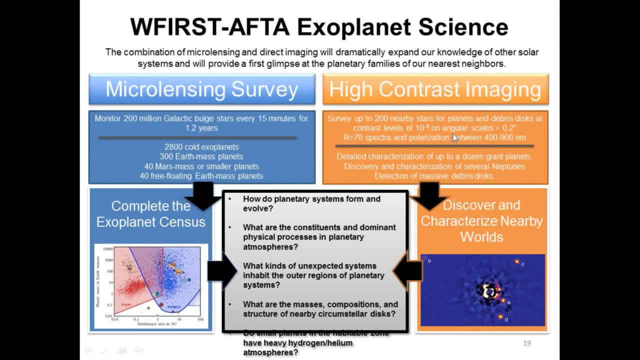 And then for the high-contrast imaging, we want to look at individual stars very nearby again. You've probably seen this picture of HR 8799.. This is a ground-based image, The stars blotted out here and you start to see the planets around there. 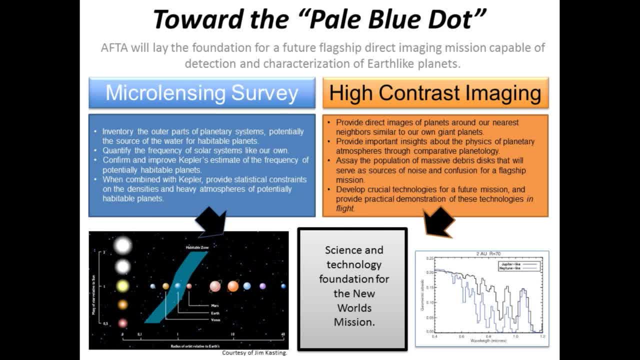 So the goal too is to take a step towards imaging Earths, And we'll need it scientifically and technologically, because we just haven't flown this kind of hardware before that can do this sort of active wavefront control, And also we haven't gotten any reflected light spectra. 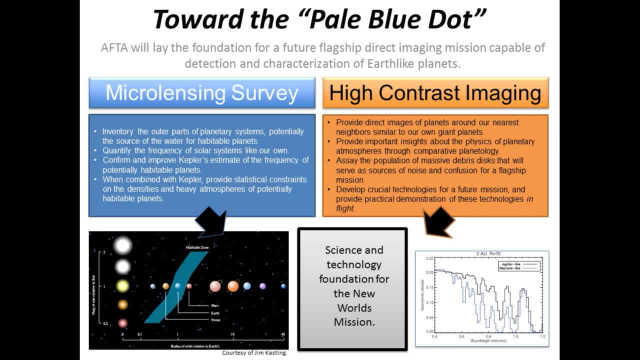 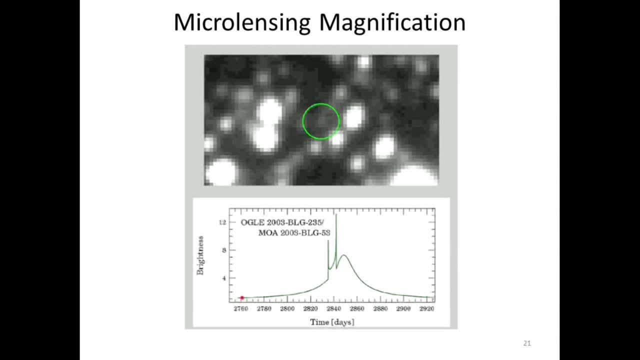 of any planets besides those in our solar system, So we will learn from both of those. The microlensing survey is the one that's going to be complementary to Kepler. It's going to net, hopefully, about 3,000 planets And the way microlensing works. 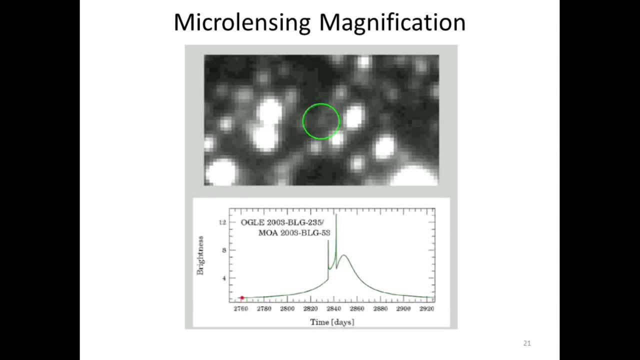 is that this is a ground-based image. You can see why we want a space image, because it'll be much sharper. So there's like a background star somewhere here, And then the idea is: is that if a star between us and the background? 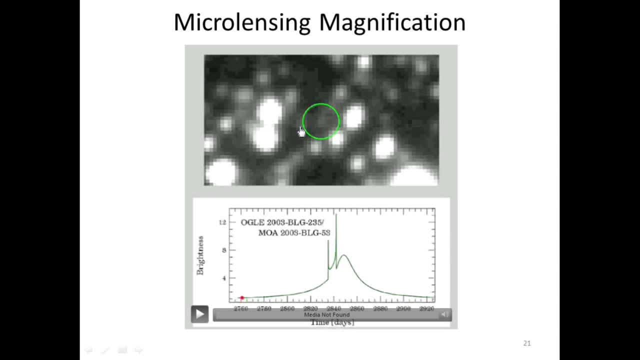 so this is the star in the background- is like at the center of our galaxy, then a star between us and this background star will move by it, causing this background star to brighten, because the gravity of the foreground star bends more light in our way. 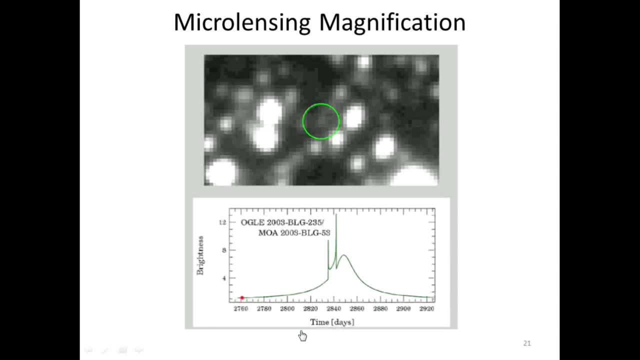 And then that's sort of what you're seeing down here. This is just a plot of time showing how the star will brighten, And you see these little narrow blips. Those are due to planets around the star, And it's a wild technique. 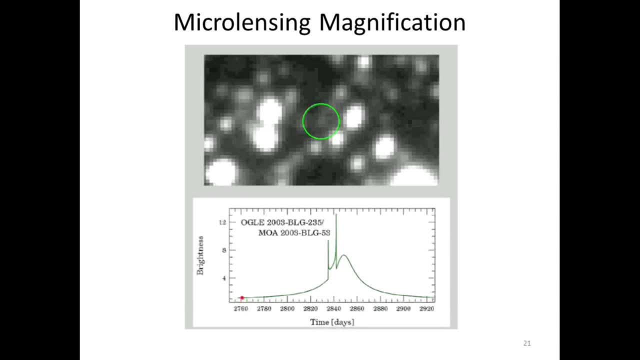 but it's already found about 20 planets or so on the Earth And we expect to find thousands, if we can do this in space, because we'll have much better spatial resolution, we'll have more depth, we'll be able to look continuously. 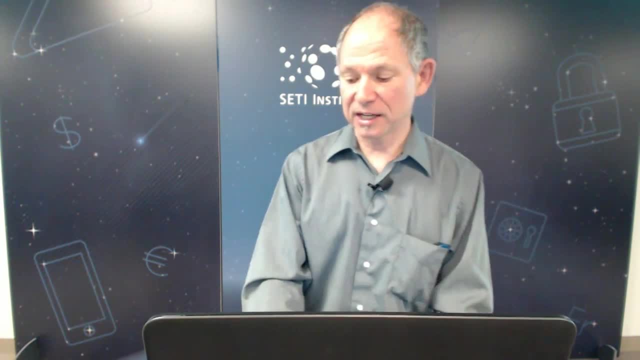 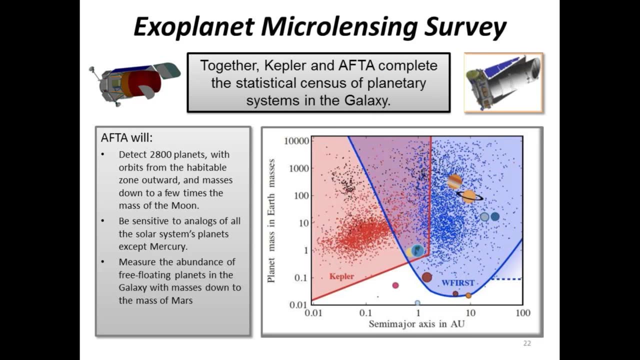 and it'll be the same kind of revolution that Kepler brought to transiting planets. And then this is a plot sort of showing the sample space. So Kepler sampled things pretty well out to about the distance between the Sun and the Earth, and this is where most of its discoveries. 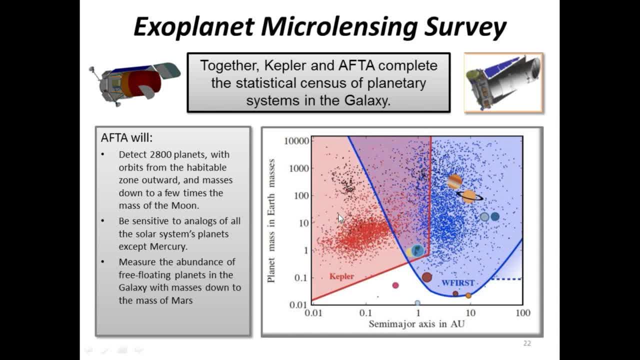 I guess have been. This is an old plot. It doesn't look like it's actual Kepler discoveries. And then W first is in blue here, and then it'll be sensitive to planets further away from their stars because they need to be separated enough. 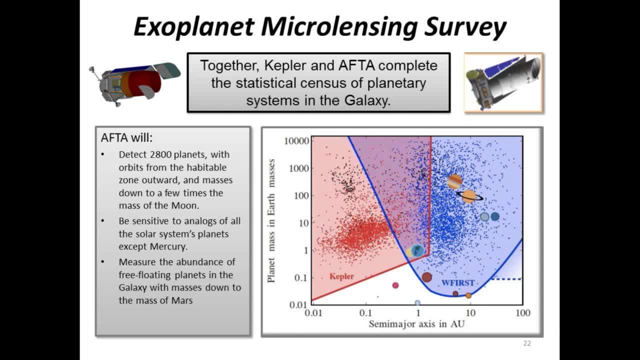 in that plot I showed you earlier so you can tell the difference between the brightening of a background star and the background star by the star and by the planet. So, Tom, what are the ones in blue? These are expected discoveries from W first. 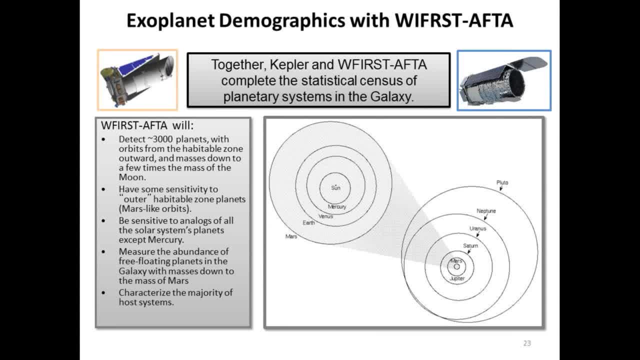 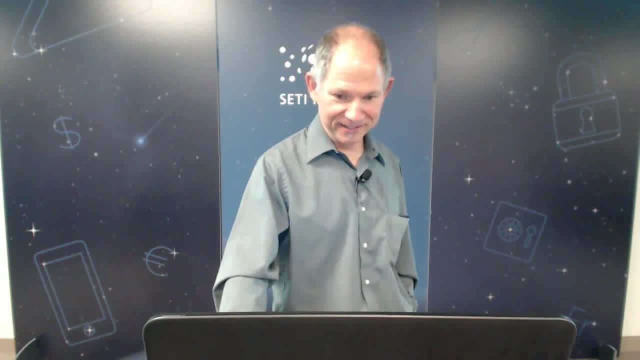 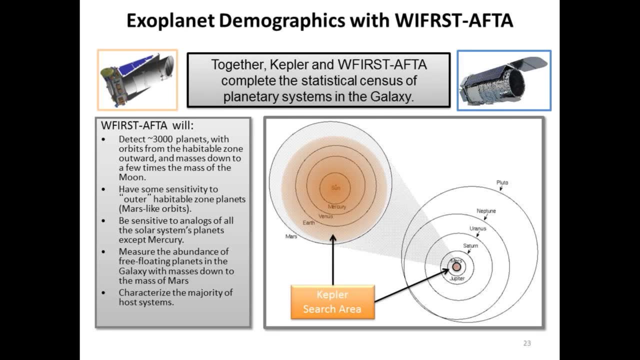 Yes, Yeah, I've gotten to a point where it's a very dangerous step for scientists to spend more time simulating data than actually getting data. So beware of simulation. So this sort of shows. also graphically the. It's a little unfair to Kepler. 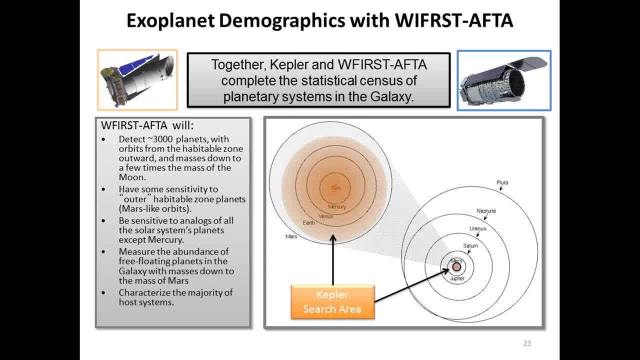 It really should be done in a log way, But where the Kepler search area is projected onto our solar system. Kepler is most sensitive to planets inside the Earth's orbit, and so that's what we have here. And then, however, W first is going to be. 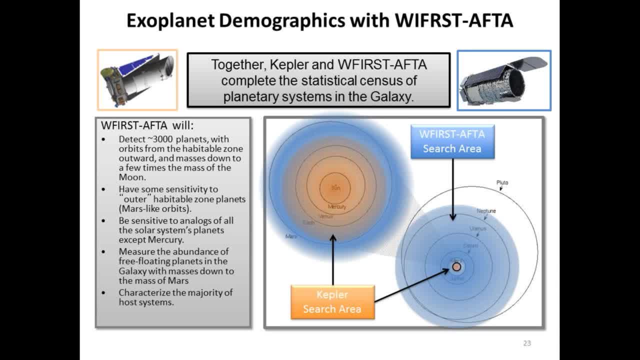 most sensitive to planets outside of the Earth's orbit. So it'll be sensing a much bigger area of the solar system. with Kepler down here and W first out here, It's maybe similar. It's a much bigger amounts of area in the logarithmic space. 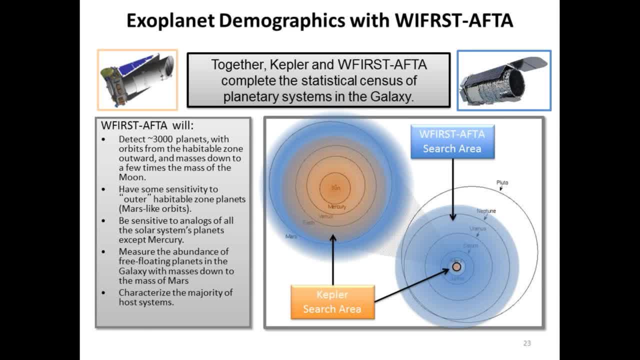 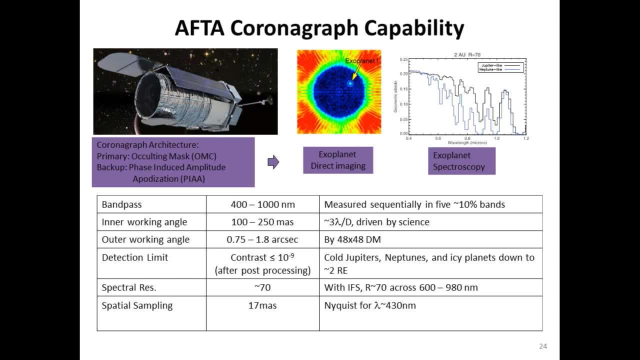 So the idea is the two together should be greater than either one and really give us a good idea about planets. So, in addition to knowing about them statistically, we want to know what we have nearby. You know where can we find oil or whatever. 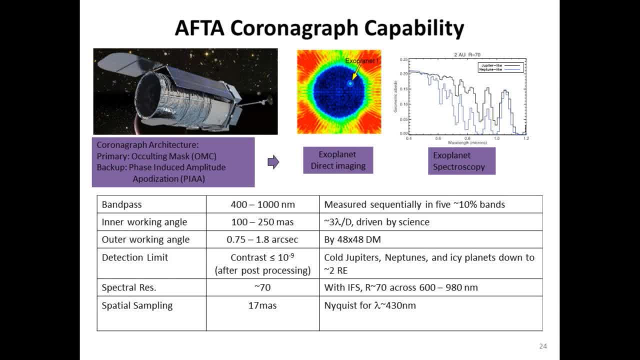 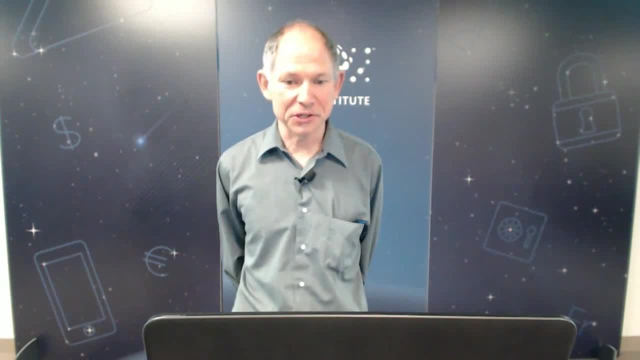 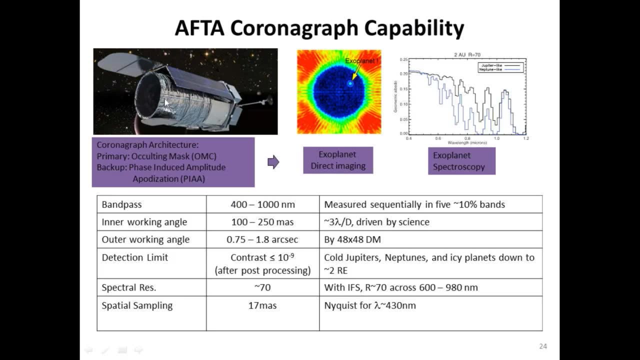 You know where. Something I thought that might resonate with SETI is searching what's going on in the Hubble zones and nearby stars, And we should be able to get pretty close to that The way these coronagraphs work. this is a concept of the aft emission. 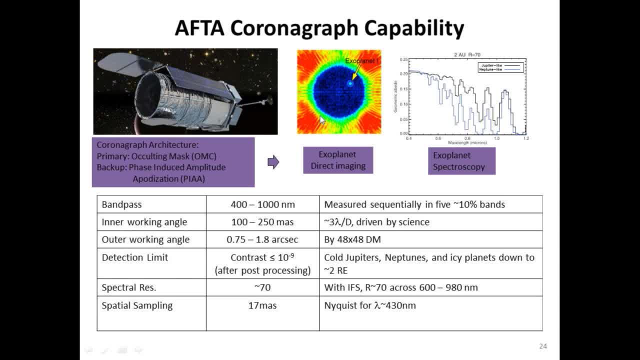 The star is blotted out. Then there's an area that's controlled here that's pretty small, It's like an arc second or so in size, And then we should be able to find an exoplanet here. that's only like. 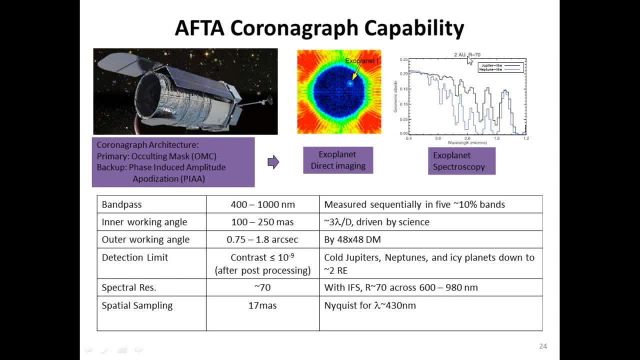 1, 1 billionth as bright as the star And we have instruments that'll take spectra. We should be able to differentiate between planets similar to Jupiter and similar to Neptune based on their compositions and temperatures. And it's a little bit about the technology. 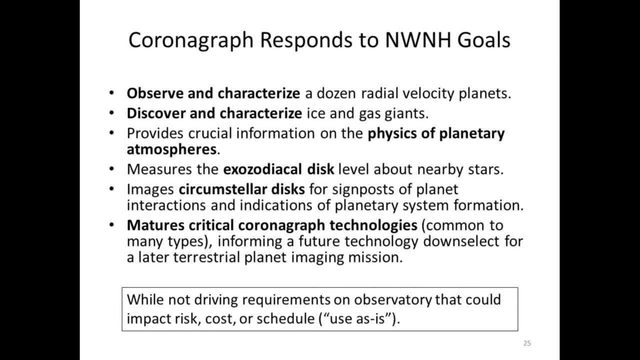 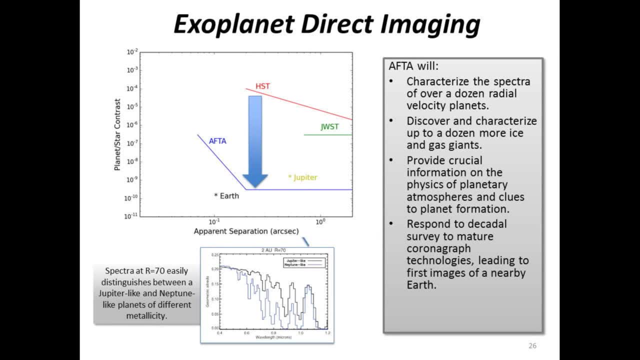 for the coronagraphs here. So in addition to finding planets, we're also going to measure this dust level around stars and mature these technologies for future imaging. This sort of shows where we are technically and where we need to be with this contrast thing. 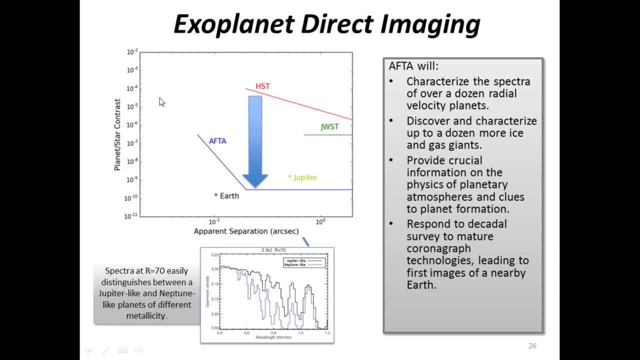 Hubble Space Telescope gives us contrasts of about 1 part in 10 to the 4. So we can see something that's about 10,000 times dimmer than a nearby star. So that's the y-axis is the contrast, The x-axis is the separation. 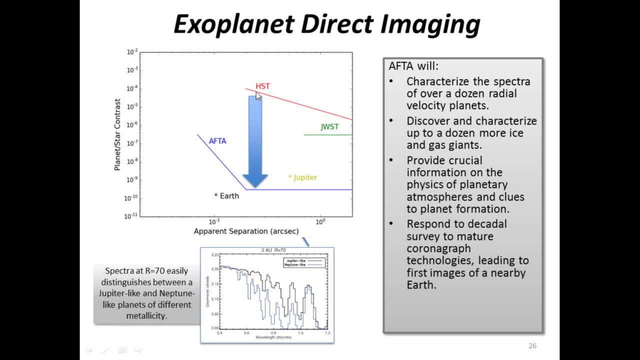 So a couple tenths, a few tenths of an arc. second away, you could see something 10,000 times dimmer than the star, However, something like Jupiter down here. you know, if you move our solar system away from us, 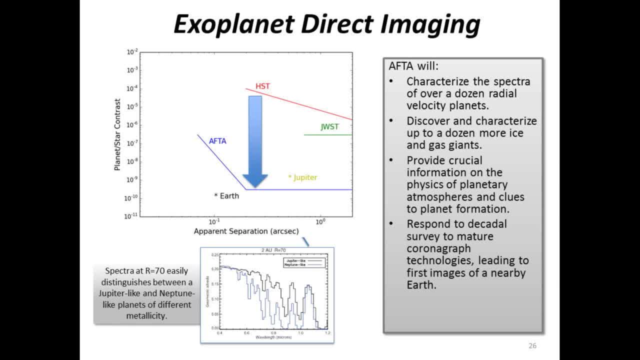 you'd see, it's about a billionth as bright as the sun. So you know we need to do a lot better than that, And Earth is 10 times harder still. So we need to follow this technology, And WFIRST will get us almost all the way there to an Earth. 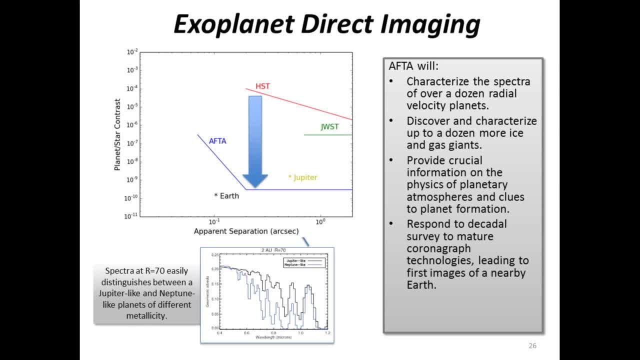 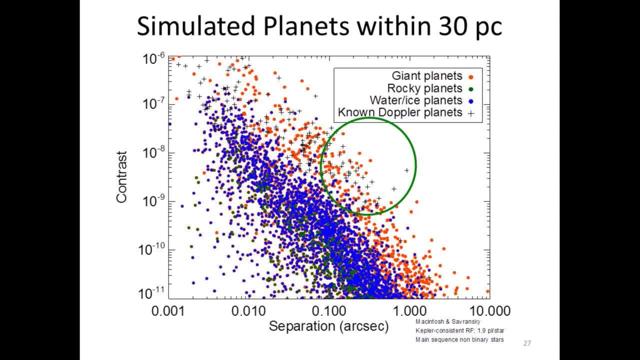 We should be able to get to Jupiter's, And it really is taking applying some advanced technology in space for the first time. This is more simulated data showing what we may expect to see around nearby stars. So if you look at stars within 100 light years, 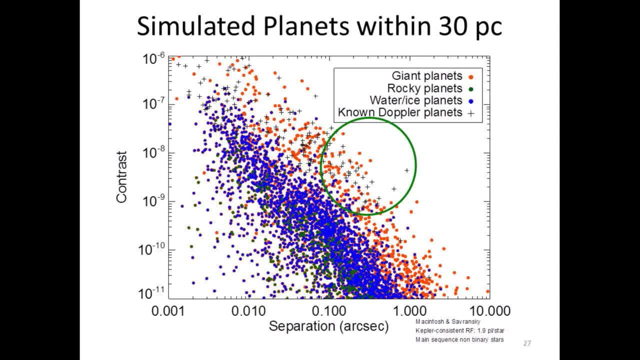 there's 30 parsecs. These are the, an estimated planet simulation using the Kepler statistics for how common planets are around stars- about two planets per star- And these are the sorts of planets that may exist there. Giant planets are the ones we're probably most sensitive to. 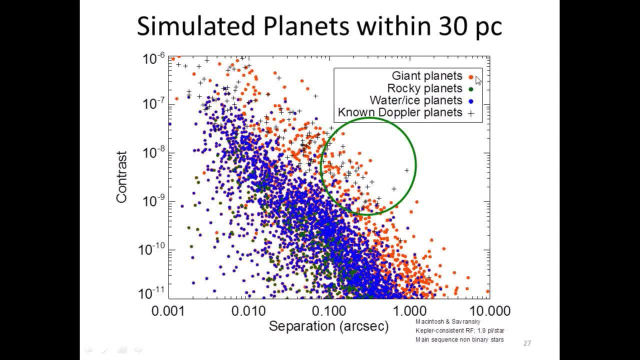 because things get easier in the top right, because then they get less, they get brighter And further away from their stars. So 10 to the minus 8 means that something is 10 one billionths the brightness of its star, And 10 to the minus 9 is one billionth of its star. 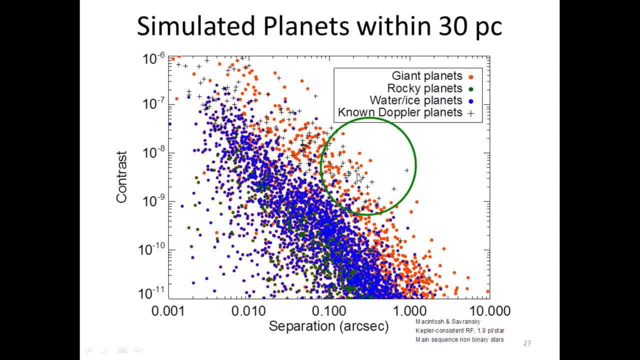 So we should be able to get some reasonable yield. The crosses. there are known planets. Those are known planets from Doppler radial velocity measurements, from like Jeff Marcy and others have been making for a couple decades now. We went to look and see how many of those known planets 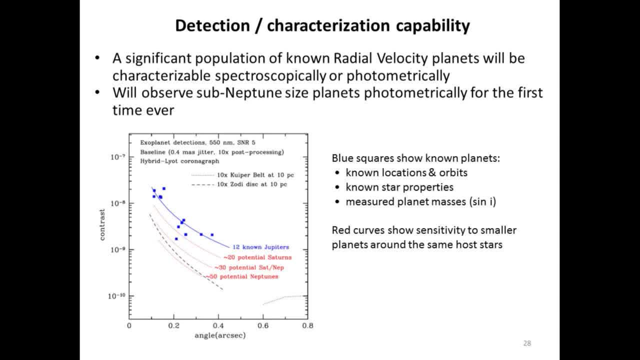 we could detect And characterize, And it turns out that we've done this for a few of the different chronograph technologies we've been studying And it looks like there are about a dozen known Jupiters that can be detected in each little over a day or two. 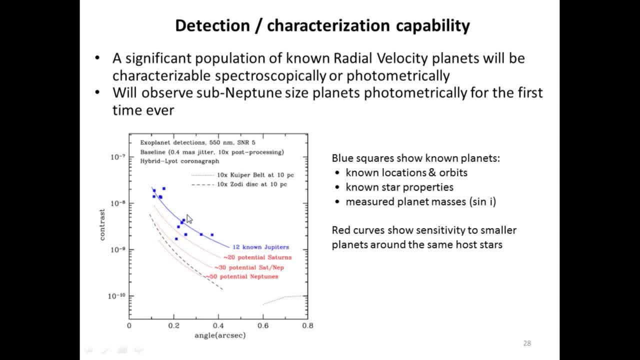 of time or less. And then, since we don't know about much lower mass ones, these sort of show potential lower mass ones, given Kepler's planet population statistics, If you just look at the same stars, there may be other planets there as well. 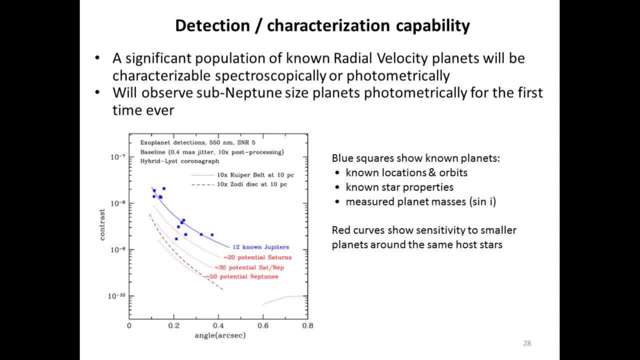 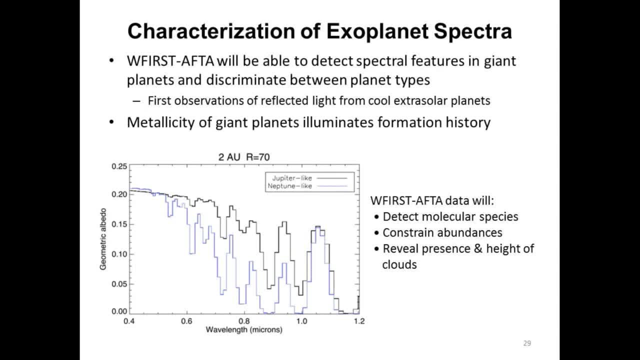 So we do have some good targets. It's good that we know their masses, because you can really understand what their spectra are telling you much better if you know their masses to understand their atmospheres. This is just a blowup of a curve I showed before. 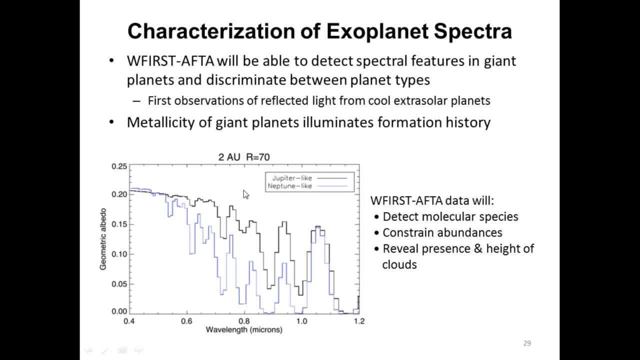 that sort of showed the quality of spectra we expect to get. So resolution about 70 is good enough to resolve these different bands of methane here. So those are the major features And be able to tell the difference if the two planets are the same distance from their star. 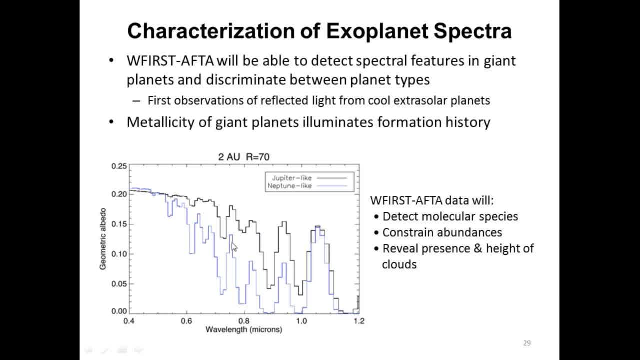 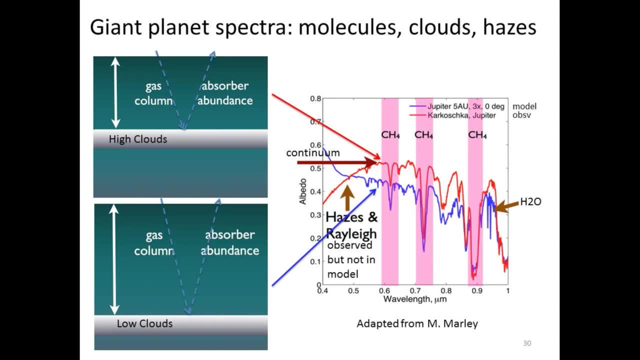 You see that this Neptune spectrum is much deeper because it's got a higher concentration of heavy elements, So there is more methane, more water in the atmosphere than compared to Jupiter, And by knowing these compositions relative to their star, we get an idea of how they may have formed. 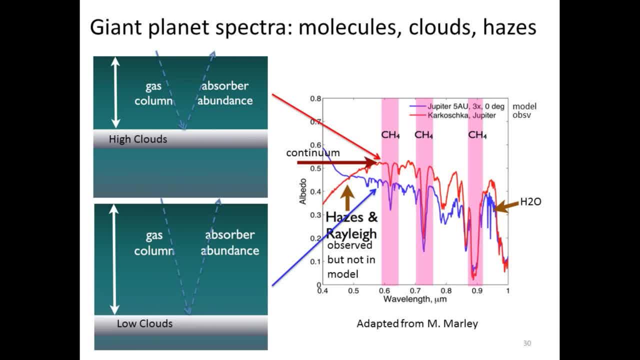 The technique that you use scientifically is actually very well developed, because this is what people use in our solar system. This is just reflected light from planets. We've been studying reflected light from planets through telescopes for 400 years, since Galileo looked at Jupiter in 1609.. 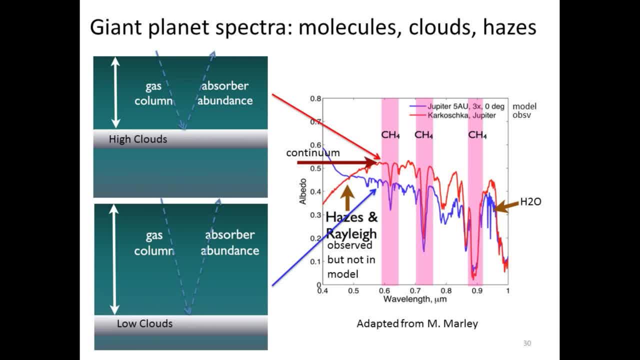 And it really evolved into a science of spectroscopy in the 1960s. What happens is that light comes in from the nearby star, goes into the planet's atmosphere, into the cloud. the cloud reflects it back out to us, to the Earth. 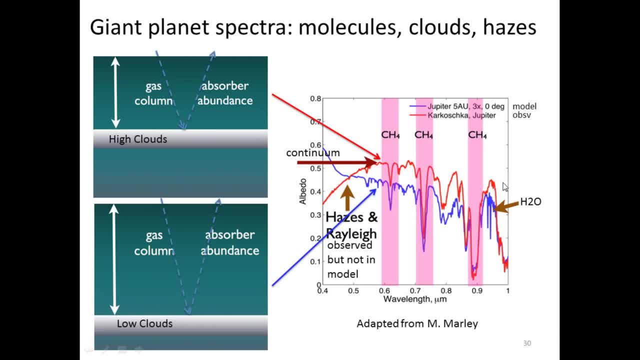 And then by looking at how much absorption there is at different wavelengths, then we can kind of figure out what's here and how high those clouds are. So there's a good bit of information that you can get from these spectra And a lot of the details have been worked out. 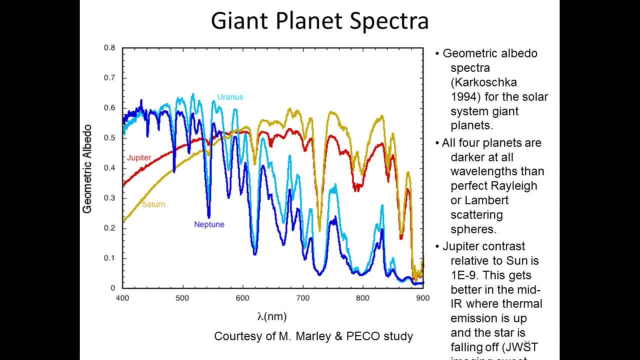 We kind of know what the limits are, what we might get. This sort of shows the differences of the giant planet spectra in our own solar system That hopefully we could observe. So Jupiter and Saturn look pretty similar here. However, Saturn is a little deeper in its methane here. 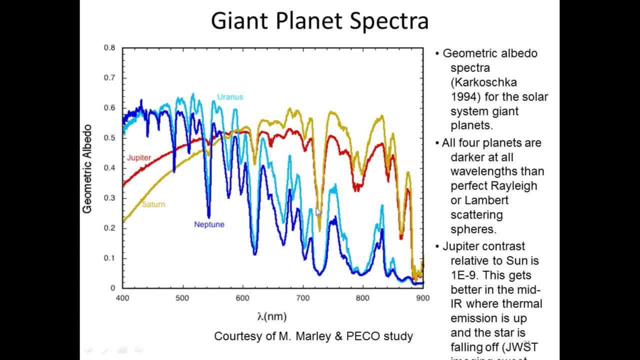 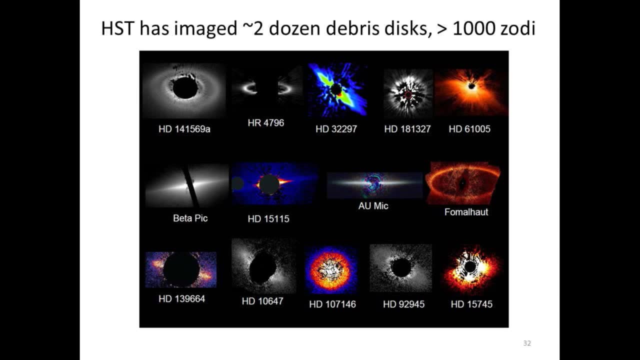 again because it's got a higher concentration of metals, of heavy elements. And then the clouds are lower because they're colder in Uranus and in Neptune. In addition to planets, we know that there are disks around nearby stars. This is disks of planetary debris. 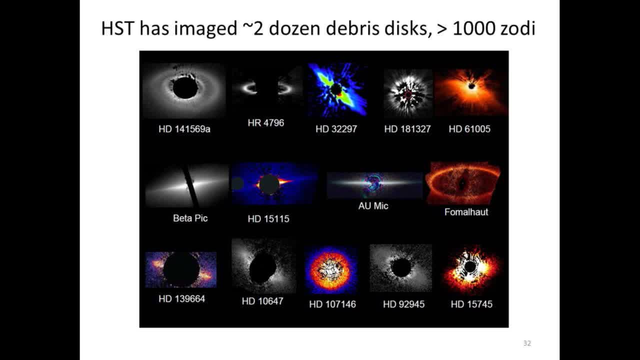 From things crashing into each other. Okay, And so the ones that are really bright have a lot of activity, So they must have planets, And indeed a number of these systems have found to have planets, Like Fomalhaut and Beta Pic. 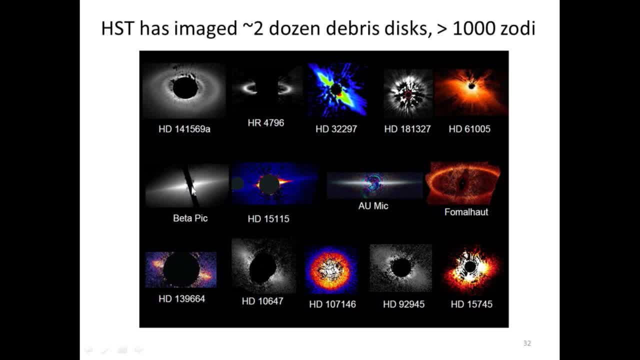 have thought to be planets there, And some of these other systems as well. 8799 is another one that's not on here, So, however, we've only really been able to look at the very brightest ones with the Hubble Space Telescope at the ground. 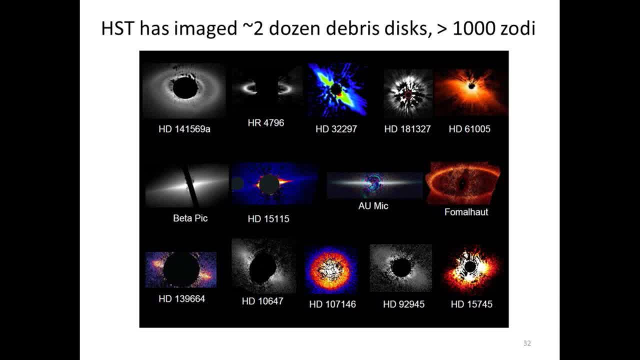 This unit here is a thousand. zodiac means a thousand times our own zodiacal cloud, So the level of dust in our solar system. We hope to do much better than that. We also will be able to image pretty close in to their stars. 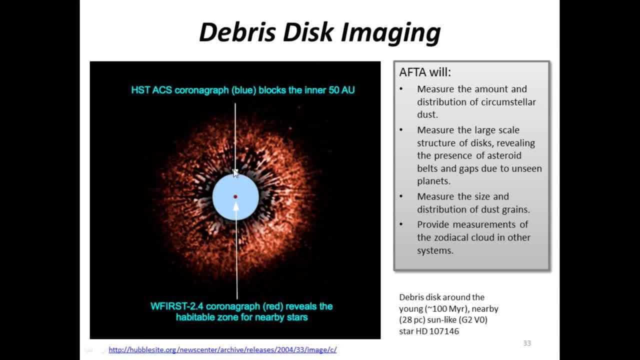 This shows the mask that's masked out in this Hubble image of a nearby star. This is a. This is a sun-like star that's about 100 light years away And, however, we can't see in to this inner region here. 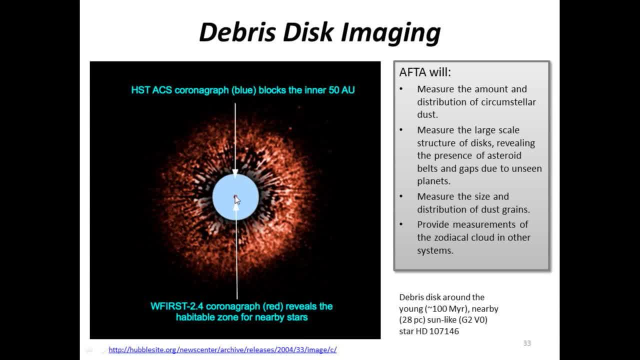 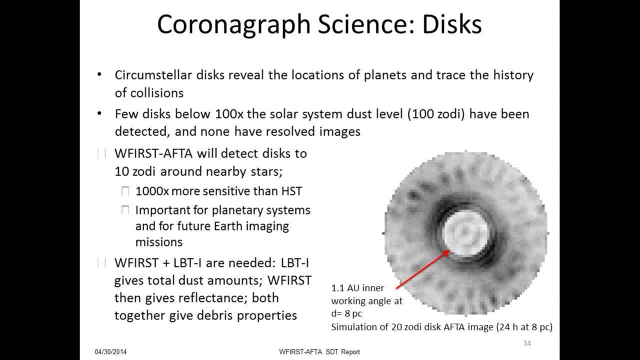 However, with this Hubble instrument, then it has almost a 2 arc second inner working angle. However, WFIRST is going to have a much smaller inner working angle, just the size of that red dot. This is, Beware, more simulated data here. 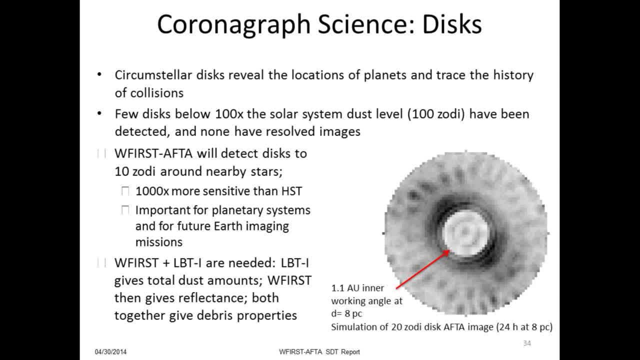 This is using the simulations of the coronagraphs with the wavefront error of this telescope and putting in different kinds of disks. This disk here is about 20 times the level of our sun. You can see the detections there. That's black there. 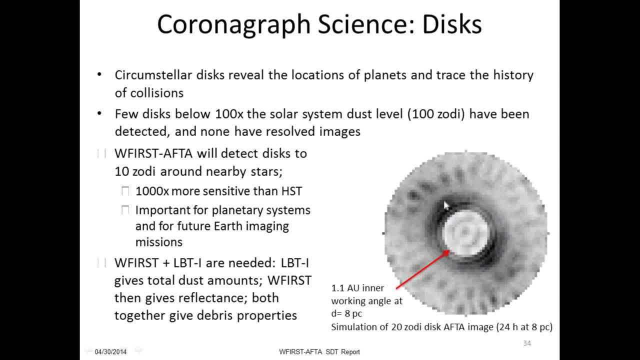 Black, some airy rings left over from the telescope, And it's inclined at an angle this way, So we can definitely detect things. Instead of being 1,000 or 10,000 zodis, we can image them at 10 zodis. 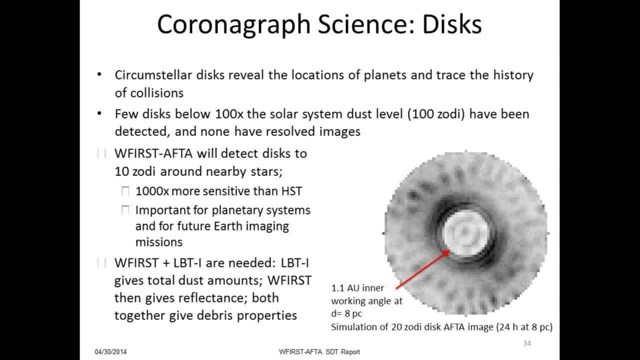 is going to be our limit. So 10 times the level of our solar system Should be a big jump there. Also, the distribution of material tells where planets are. if anything is being shepherded around, The stuff out here is all like leftover artifacts. 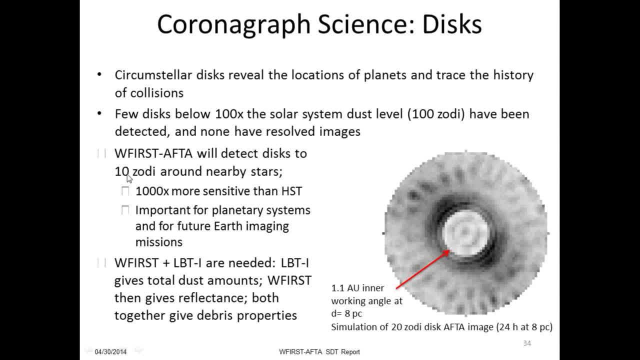 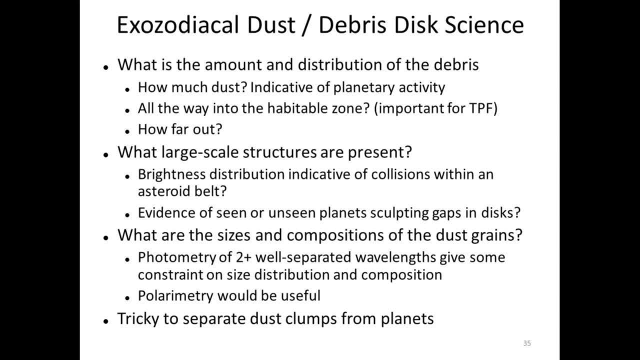 from the coronagraph and wavefront control. So the Again, the major questions of the debris disk is: how much dust is there? Where is it? That gives an idea of how much planetary activity. The other question is: what are the sizes and compositions of the grains? 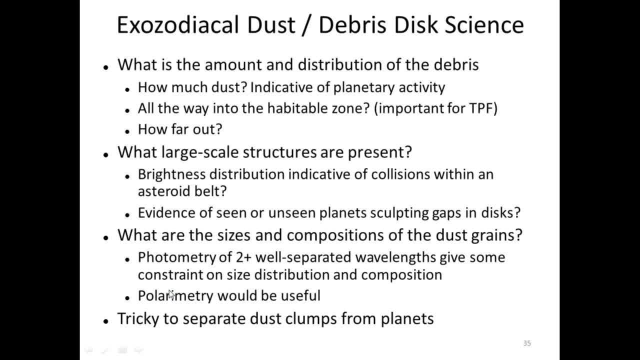 We should have a polarimeter on here so we can actually look at different polarizations coming off the grains in reflected light, which should hopefully help us separate dust from planets, because, you can imagine, a dust clump might look a lot like a planet. 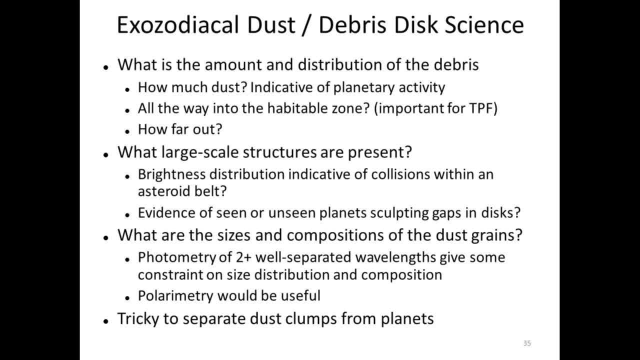 particularly if they're at similar orbits. Another thing this does is it helps us just figure out how dusty our neighbors are and how this could interfere with imaging for Earth, Because even though dust isn't very bright on a given area, but if you look within a resolution element. 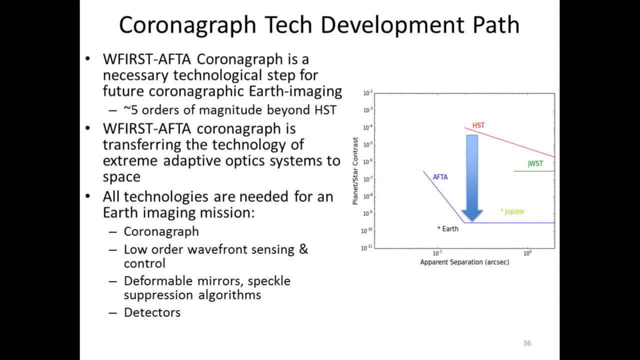 a lot of light could be there and it could be actually more than an Earth for a reasonable-sized telescope. So I'd just like to, I guess, maybe reiterate a couple points I made on this first planet graph. We want to go five orders of magnitude beyond Hubble. 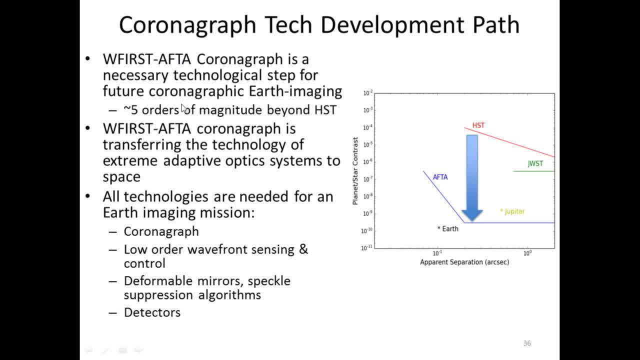 in terms of how well we do this contrast, suppression, And that's this big jump in contrast from 10 to the 4 to 10 to the 9, so we can suppress the starlight by a billion times. And the technology we're using. 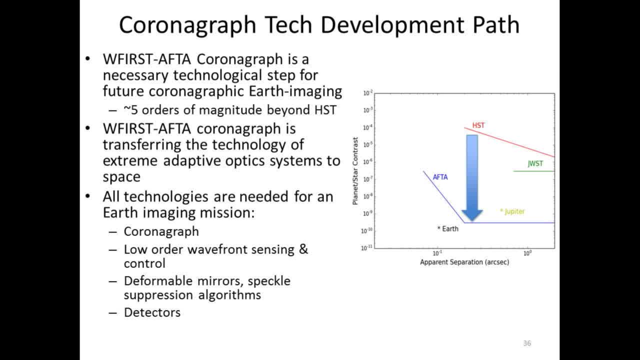 is a lot of the same technology that's been developed from the ground. It's been applied in space. The algorithms are pretty different because you have different kinds of disturbances. Here it dominates on the ground. It's a very fast thing. In space we have much slower disturbances. 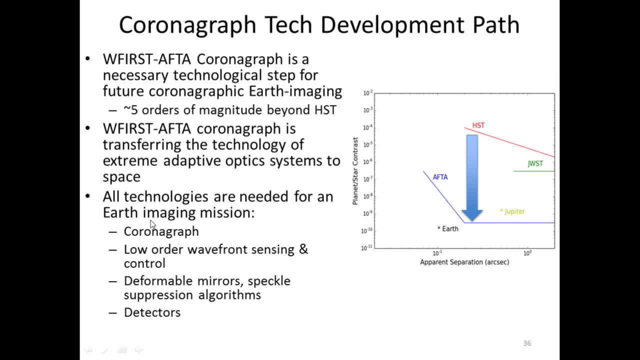 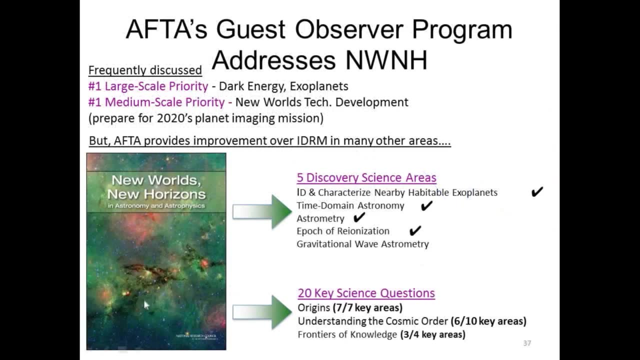 But all these individual items are needed in future Earth imaging missions, So it should be very useful to advance the technology. This is these chronographs pointing control. that's what this lower stuff is: deformable mirrors. speckle suppression detectors. 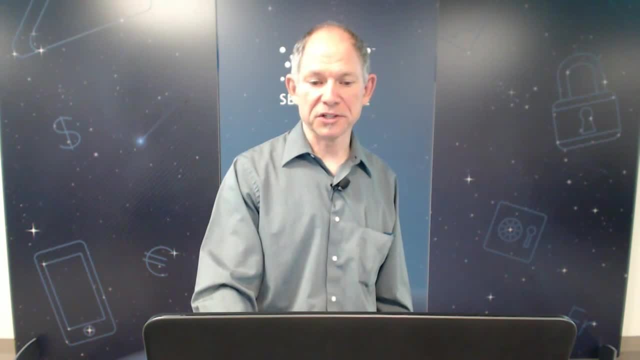 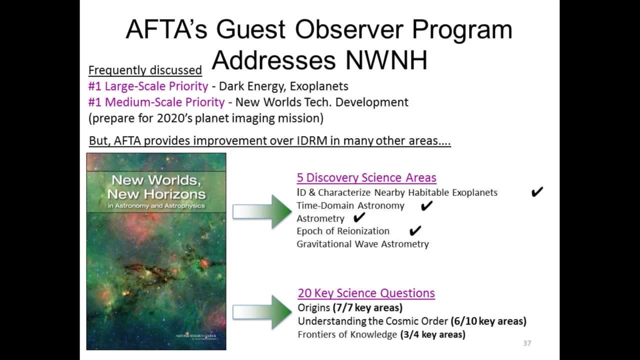 No, no, there's a performance. The question is, what is extreme? AO? Yeah, we can maybe handle that in the questions at the end. Okay, so in addition to doing this dark energy and doing planets, there are a lot of smart people. 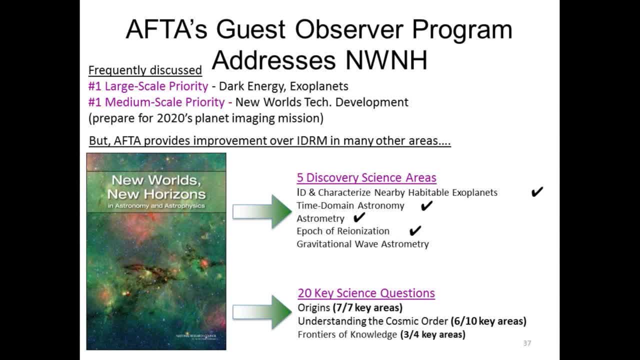 When you have a telescope that's capable with an imager like this, there's going to be a lot of other science people who want to do. We actually solicited white papers from the community last year and we got over 50 responses for some great ideas. 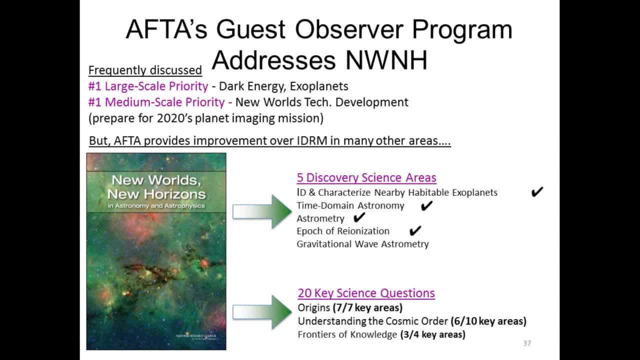 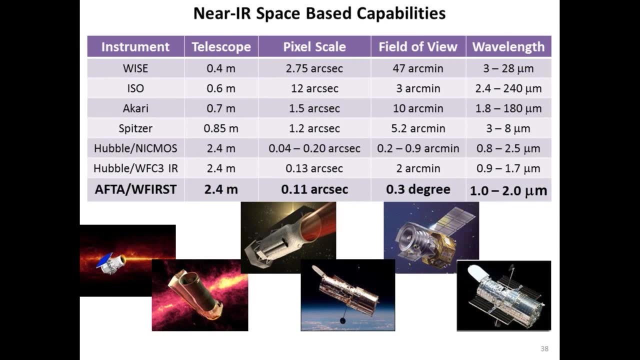 I'll try to illustrate a few of these. And there's just a lot of discovery from near to far, from looking for the closest stars- M dwarfs and brown dwarf stars- out to the most distant galaxies in the universe. This is a little bit of a comparison. 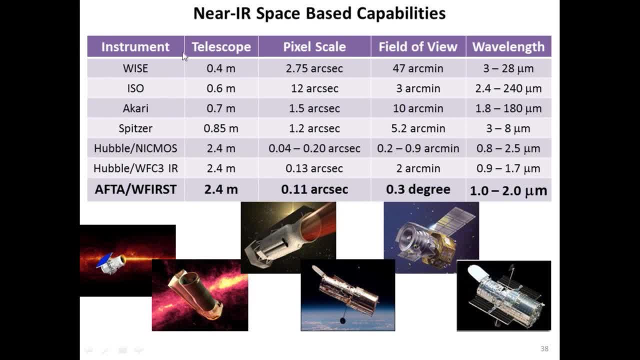 of different current and recent, somewhat recent observatories. So from the WISE Explorer at 0.4 meters up to Hubble at 2.4, now AFTA. So you see we've got about the same spatial resolution in this column as a Hubble Space Telescope. 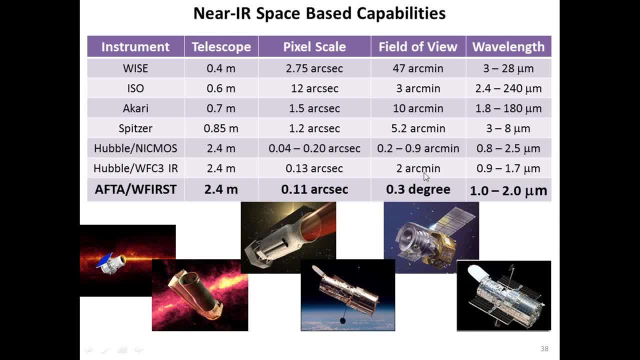 maybe a little bit bigger, but again this much bigger field of view and the similar wavelength coverage. Then Spitzer is still flying, It goes to longer wavelengths, but it has nowhere near this kind of field of view or just the light-gathering power. 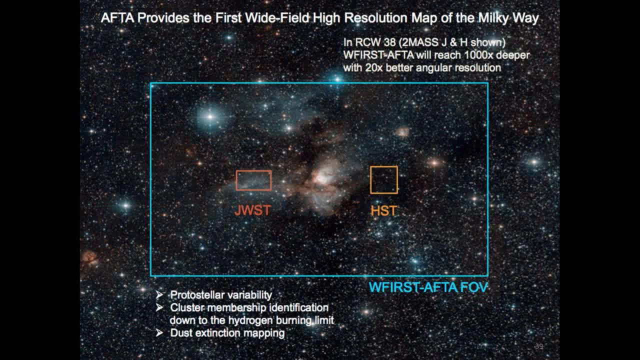 This is going to be tremendous for doing imaging in the Milky Way. This is a star formation region in the Milky Way. Right now, the only really wide field surveys we have have been done from the ground because we just haven't had the time and an instrument in space. 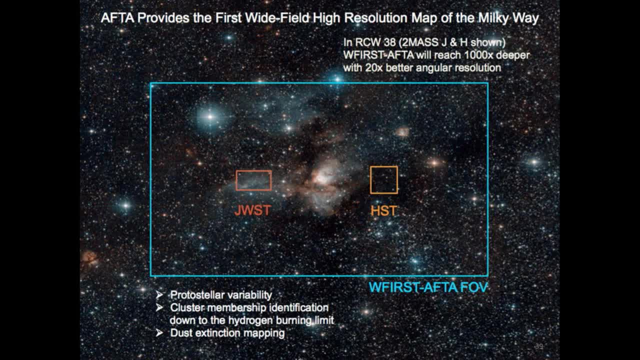 with a big enough field that could do everything. You know that Larry here was instrumental in 2MASS and this should be something like a thousand times deeper than this 2MASS survey here. This again shows the W-first field and what Hubble sees in there. 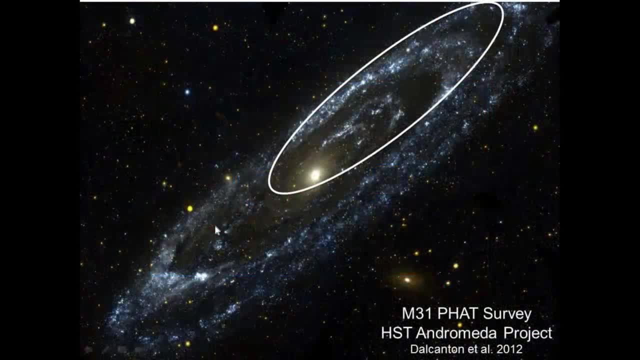 and what James Webb sees in there, So be able to do some great surveys. This is an example of our nearest grand spiral neighbor galaxy, Andromeda Galaxy and M31. This is a region about over a third of the galaxy that's being surveyed now. 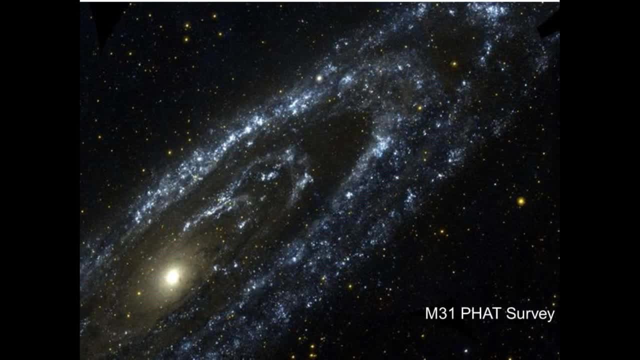 with the Hubble. That's a close-up of it. You can get multiple spiral arms in there. understand about populations of stars in here And you need to look at a big region to understand gradients in compositions as you go out and also any kind of changes in ages. 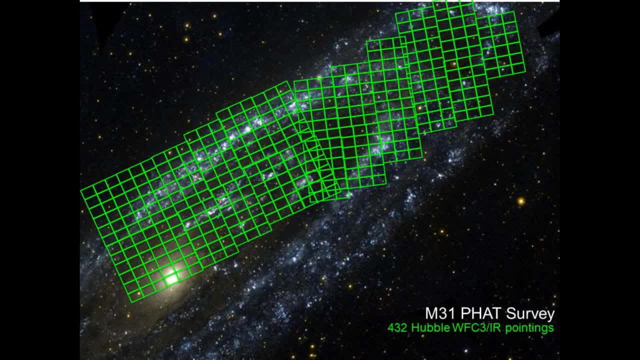 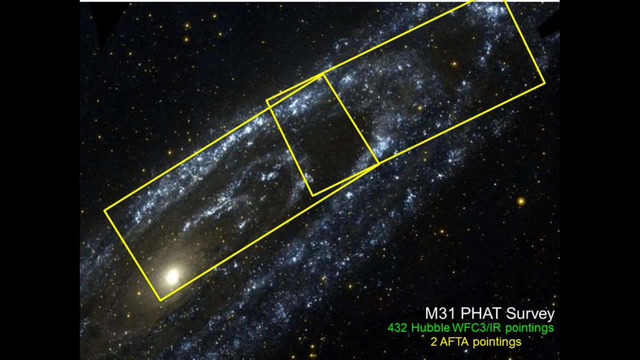 And so this is what some poor people are doing on the Hubble 432 fields okay to do this, But if you had W-first, it's two fields- okay, with some overlap. So you know it really enables science. 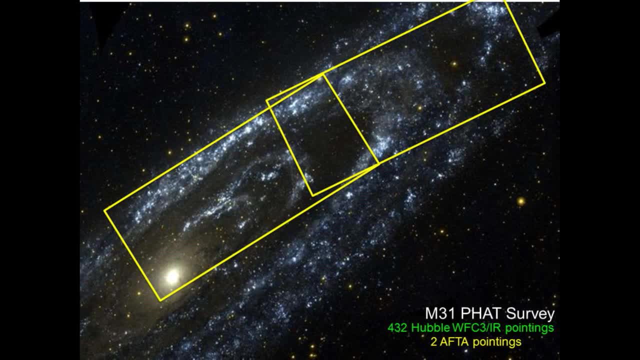 on a different scale. You really enter the statistical realm when you've got a field like this. Now the ground's been doing this for a while. The Sloan telescope is probably the first one to do this. The LSST is coming online. 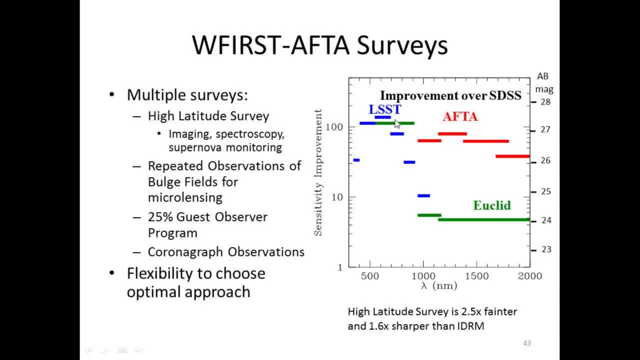 And this sort of shows that we're going to be very complementary to this LSST. This is a 6.5-meter telescope. It's being built now. It'll be located in Chile And it only really works out into the visible. 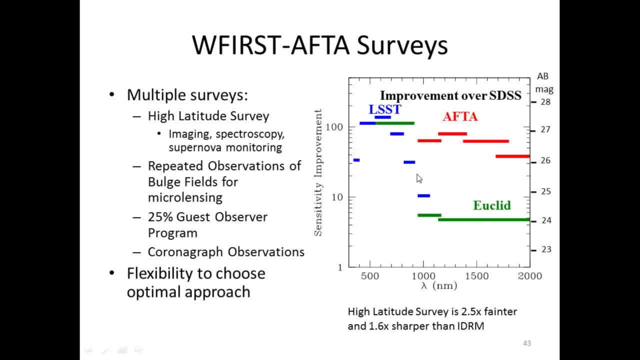 You see its sensitivity. This is the y-axis. It falls off a lot down here, But we pick up in the once you get to a micron. So it'll be very similar sensitivities to what the LSST is going to see. 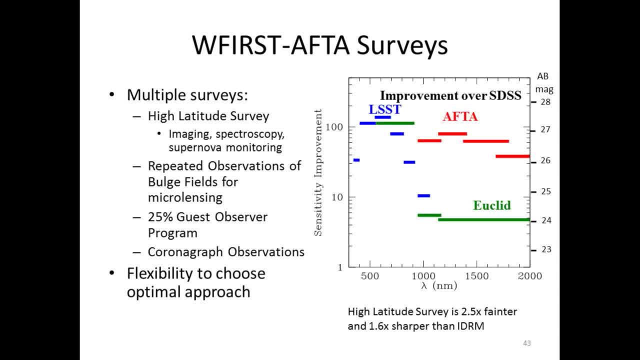 So it'll be able to actually look at some of the same objects over this really broad wavelength range. Europeans are building another mission for dark energy. They're building another telescope, It's Euclid- And you see, in the infrared it's really not going to have. 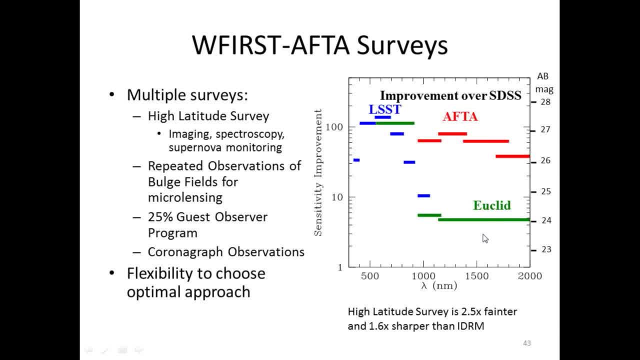 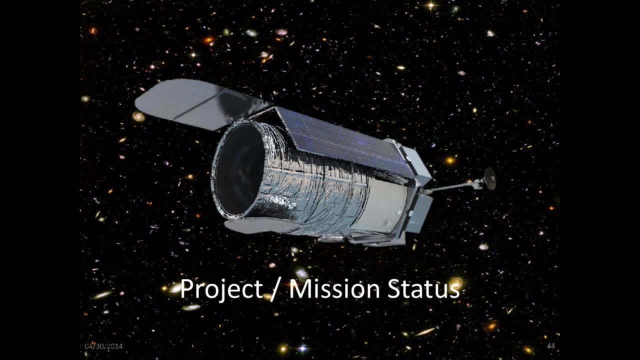 the same kind of capabilities, The orders of magnitude: an order of magnitude less sensitive, So it could be a factor of 100, different in time. All right, Just a few words on what's going on with the project status. This is a rendering of what 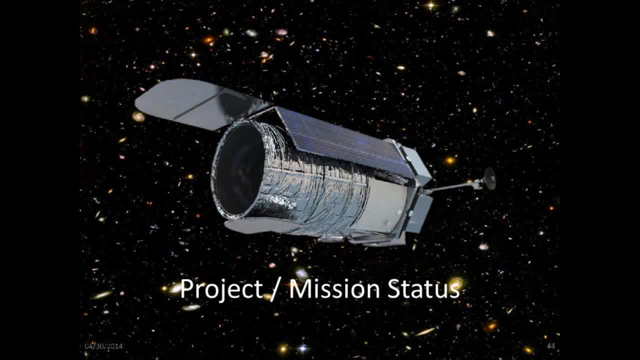 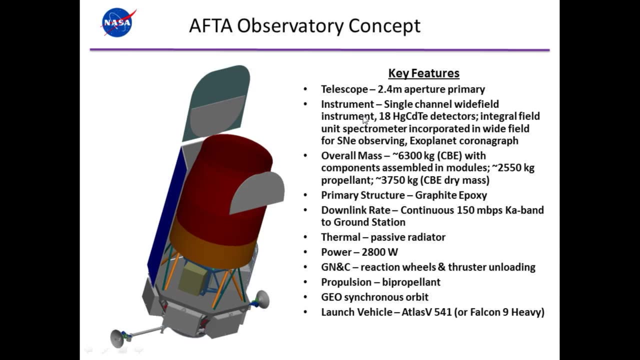 the observatory would look like It's based on a solar dynamics observatory bus, which is a similar size telescope, Also in geostationary- no geosynchronous orbit, not geostationary orbit, which is where this is going to be. 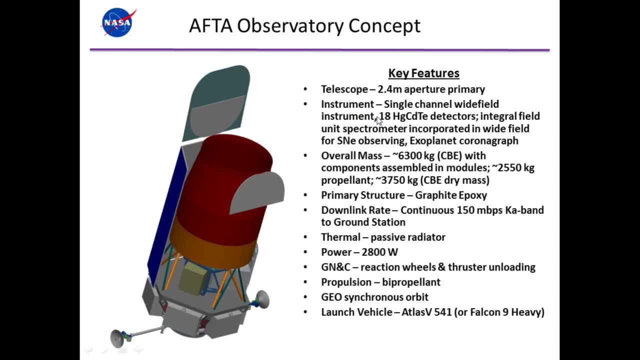 2.4 meter mirror. We've got this wide field instrument, 18 detectors that I've been blathering about. We'll have the chronograph and supernova spectrograph. It's going to be heavy Over six tons. This is about the weight. 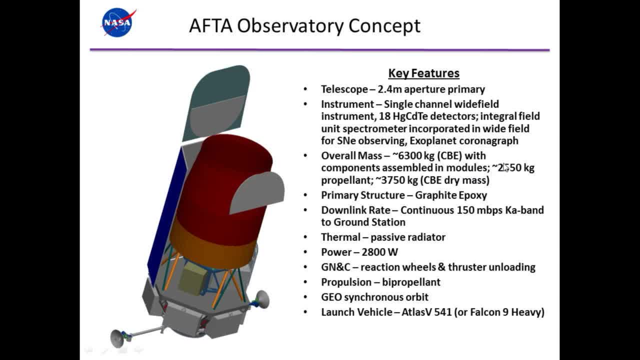 of the James Webb Space Telescope And a lot of this you see is going to be fuel. You look at the difference between propellant. Look at two and a half tons of propellant. This will allow it to maybe move around in its orbit. 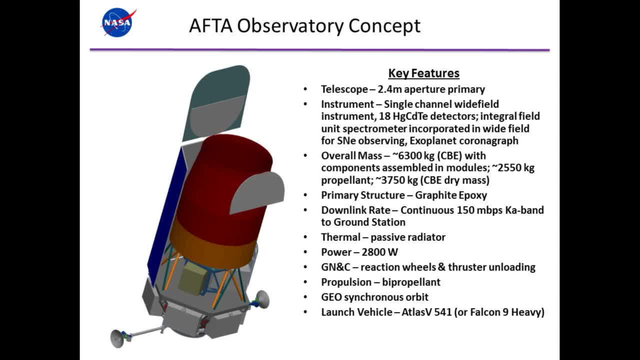 And one of the goals is to have this thing robotically serviced. So actually it's sort of a constraint for us. People think that there's going to be a market for doing servicing of the spacecraft in geosynchronous orbit. There are dead communication satellites there. 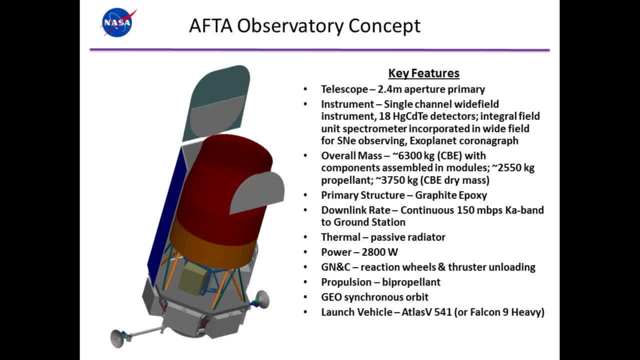 only because they've run out of fuel. And there are people right now that are working on these kinds of things And we've got a standard interface bus that they may be able to swap instruments out. Are you talking robotic servicing? Robotic servicing: yes. 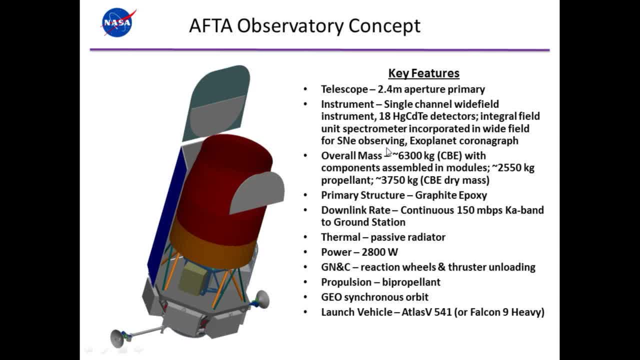 No, this is geosynchronous orbit, But we may need to get to geostationary, depending on where the robotic servicing is. That's why it has a lot of fuel there. Anything else compatible with Atlas V or Falcon 9 Heavy? 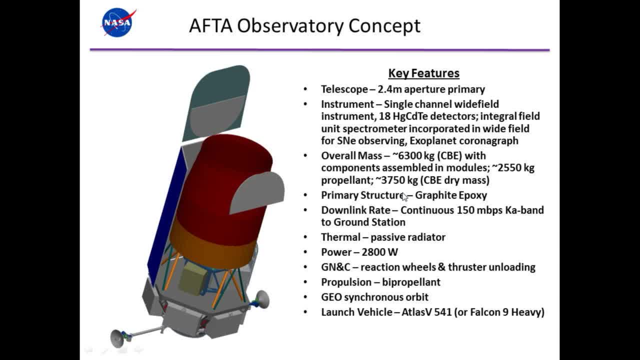 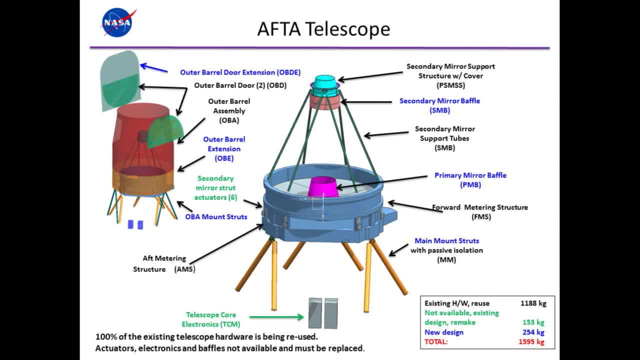 It's probably a little big for a regular Falcon 9.. Hopefully those will become available. That could help keep the cost down. This shows the We're going to keep the same basic telescope structure. Unfortunately it has these six struts that are rather large. 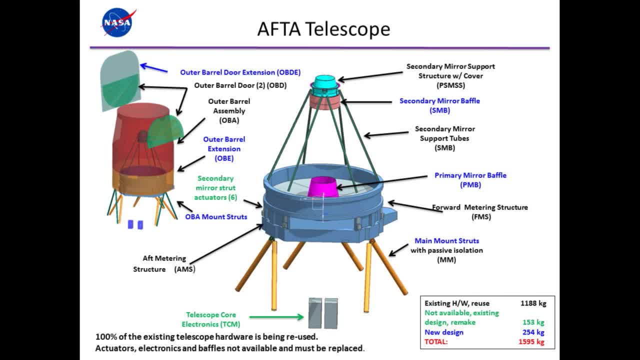 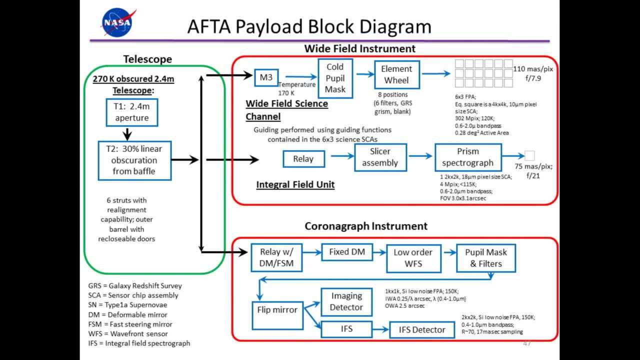 And that's what's really hindering performance the most for this planet imaging. It's just diffracting a lot of light out. But, as you saw, the chronograph should be able to still image large planets around nearby stars. Let's see if there's anything useful down there. 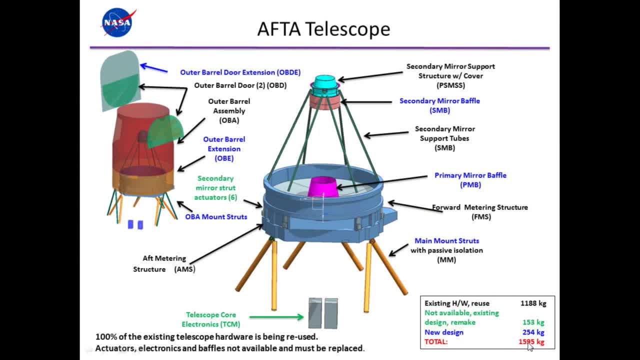 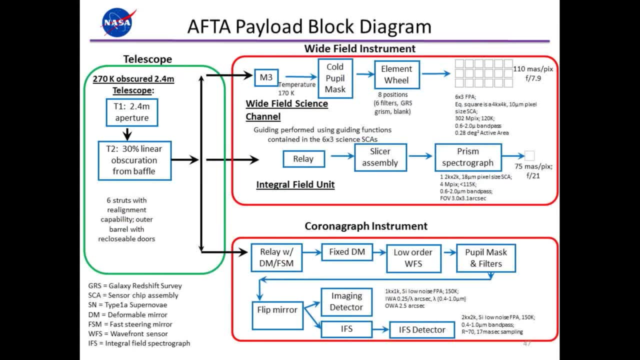 Oh yeah, so the telescope is about 1,600 kilograms, So 1.6 tons of the six tons total. So it's quite the most substantial element there. Just a schematic: The telescope right now is a two-mirror telescope. 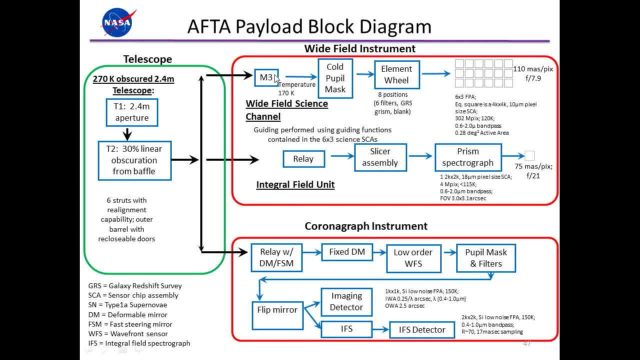 However, what we're going to do is add a third mirror And we're going to resurface this first mirror, that 2.4 meter, And it turns it into a three-mirror telescope, And that's how you get the huge field. 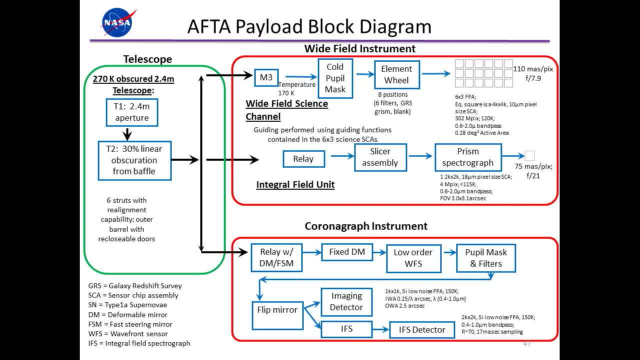 Something like the Hubble optics alone isn't going to give you a huge field, But if you turn it in, you make a three-mirror and a stigmat And you get a big field of view which enables it to use this big focal plane. 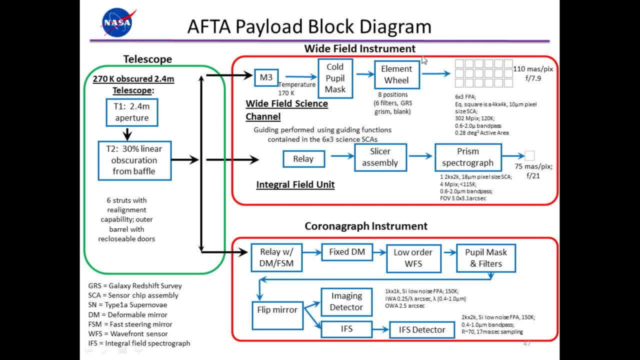 of detectors that we saw, And then there's a. We'll have different filters that could image here. There's also a grism here that will actually give a spectrum of every field point on here And that's going to be used in the Baryon Acoustical Oscillation Survey. 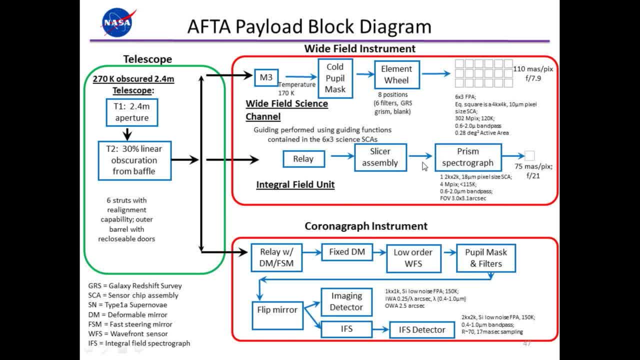 A separate little spectrograph just to look at individual supernovae. And then the coronagraph has got all the GWIS parts here from ground-based adaptive optics. There's informal mirrors, There's a low-order wavefront sensor that looks for things. 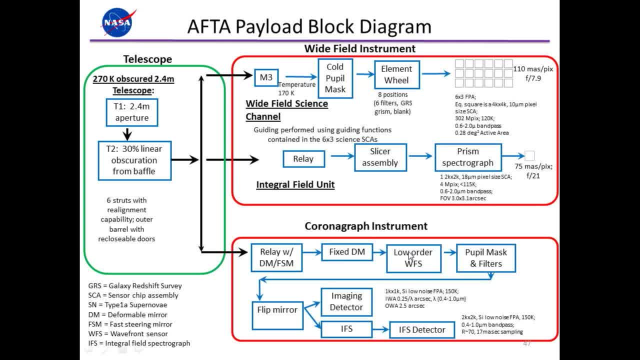 like on the order of, you know, 100 times a second and slower. And then we'll stabilize the wavefront with these formal mirrors. And then there's also There's a camera- We'll be able to take the pictures- And a spectrograph. 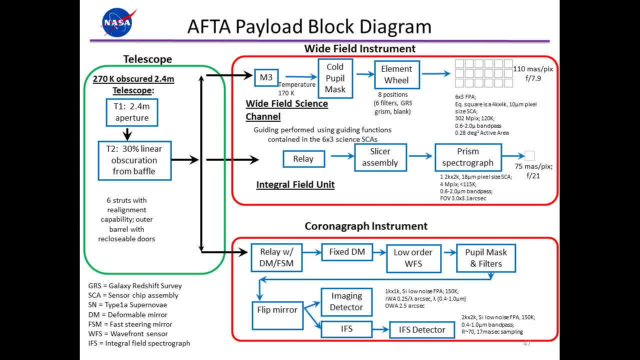 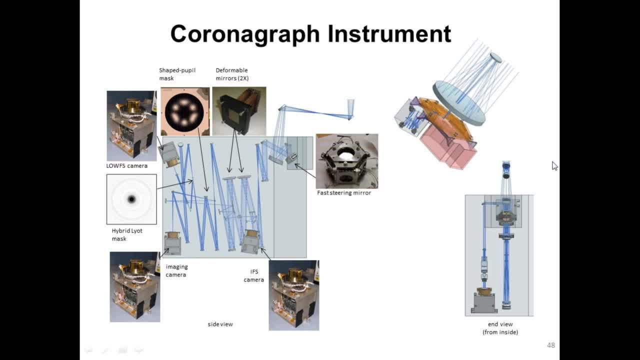 will give the sort of spectra that I was trying to show for what the planets may look like. This hardware exists for the coronagraph. This is the telescope here and sort of shows the light coming into the coronagraphic instrument and goes through a bunch of full mirrors. 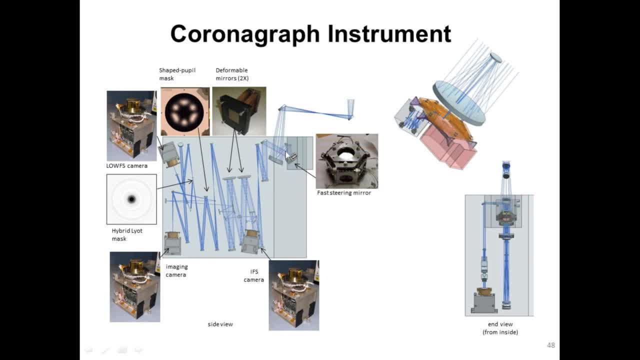 and the steering mirror here that takes Corrects any kind of fast steering that, any jitter the telescope has. Then these are the deformable mirrors that the telescope has remapped onto them And they kind of touch up any kind of optical problems across the surface. 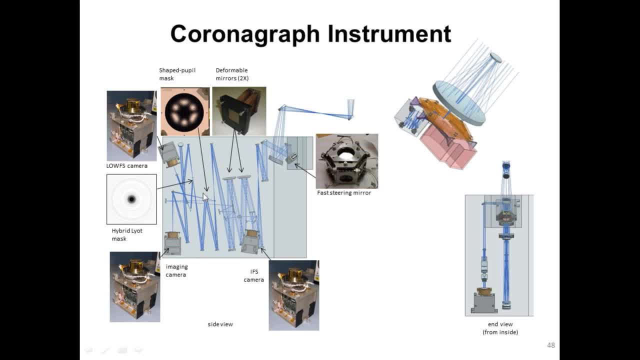 And then the coronagraph guts themselves, or here, And that's what suppresses the star, And then we get imaging onto the camera here or spectra into this camera. So good news, All this stuff exists. We just need to make a system and fly it in space. 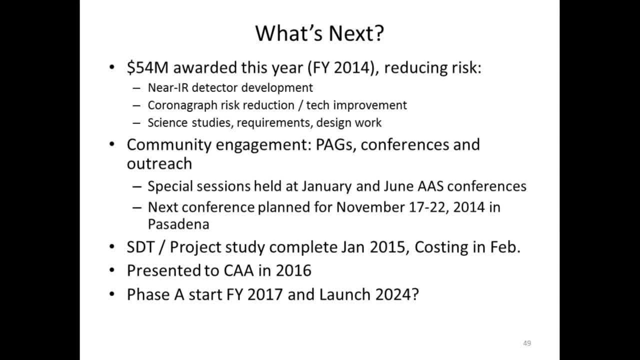 Easy. So just a wrap-up here as to what's coming next. So we're lucky. this year, The Senate wrote in $54 million for this. This is a lot of money for a project that hasn't even started yet, And so we're using it to reduce risk. A lot of this is going into developing these near-infrared detectors. The ones we need don't exist yet. What we want to do is take the ones like they're on James Webb and make them smaller. So that's really where this development is going. 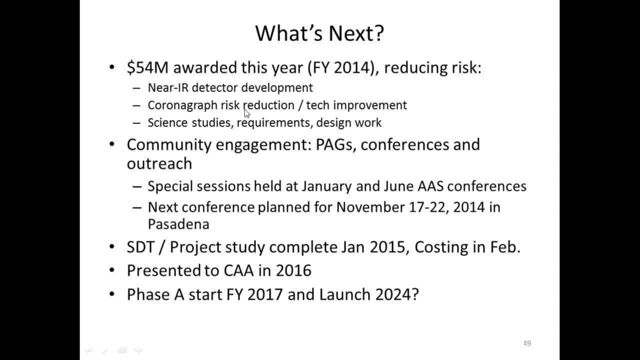 A lot's going into this coronagraph, A lot of work being done at JPL, along with funding some of the people that came up with the coronagraph designs. Also some science studies And like, for example, I'm doing disk simulations. 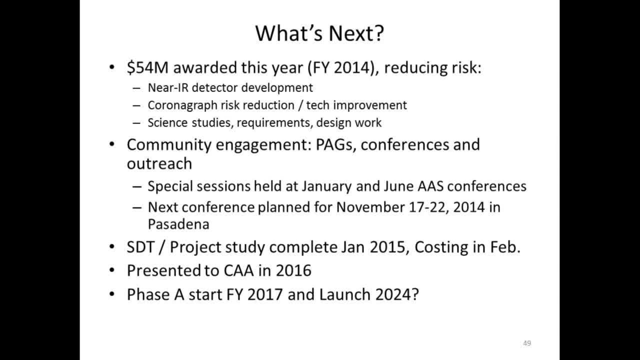 Other people are doing dark energy simulations And a lot of design work trying to figure out how cold can we take this telescope? Can we operate it at longer wavelengths into the infrared And also flowing down capturing requirements and flowing them down now? Really want to reduce risk. 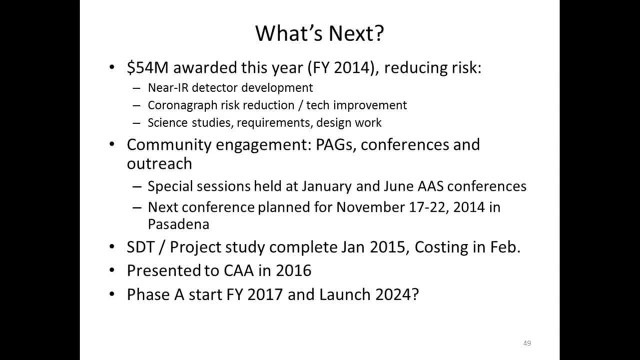 so that when we do get the OK to start- hopefully around 2017 or so- then we can just have a plan all mapped out, Trying to engage the community. Have talks- I have this talk here- Been having sessions at the American Astronomical Society meetings. 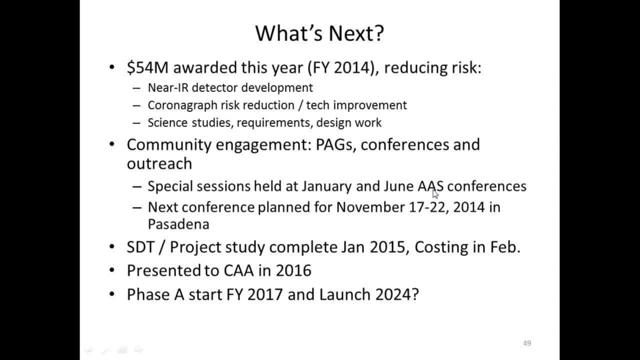 Going to actually have a cold planets meeting in the Boston meeting in June. Then there's going to be a surveys meeting this fall in Pasadena. So for probably the dark energy survey and the microlensing survey We're going to complete the science studies. 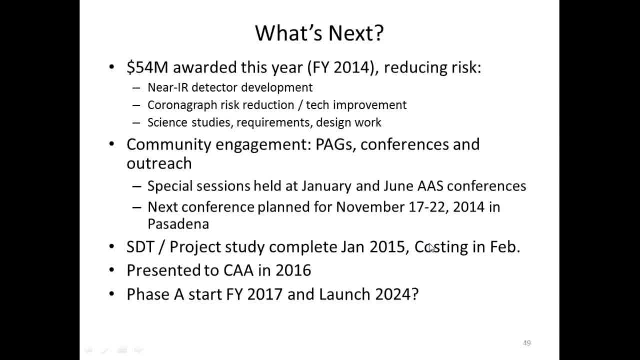 and the math team is going to complete its report in next January, And then the whole mission is going to be costed again by a third party, by the Aerospace Corporation, And then there's going to be a mid-decadal review as just part of the whole. 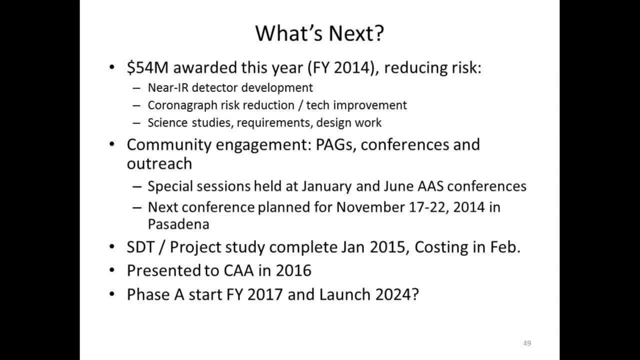 decadal survey process in 2016.. We're going to present this and say: this is what we want to do for WFIRST, And then hopefully we'll get a thumbs up And then hopefully the administration and Congress will see it fitting to fund this. 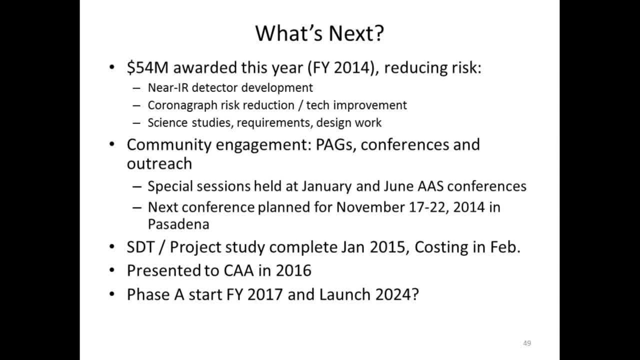 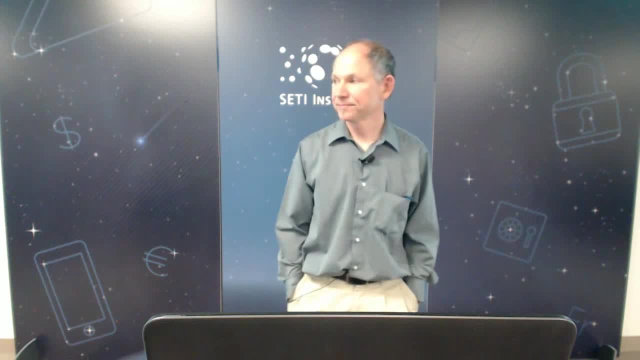 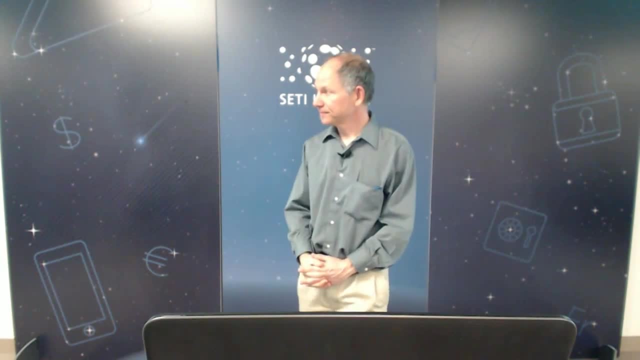 so that we can make it happen And maybe by 2024 we'll be getting data. So thank you very much, Tom. what? this is a little bit off topic, but what else is competing for the 2.4 meter darkly sourced telescopes? 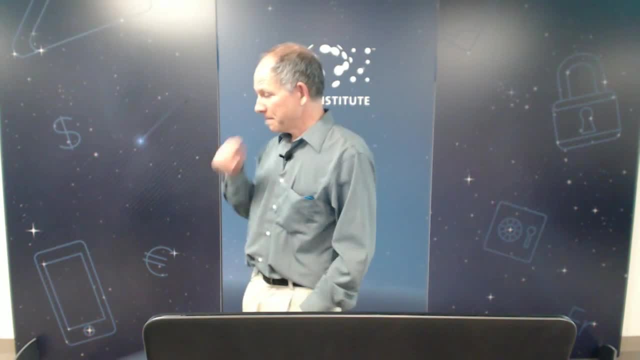 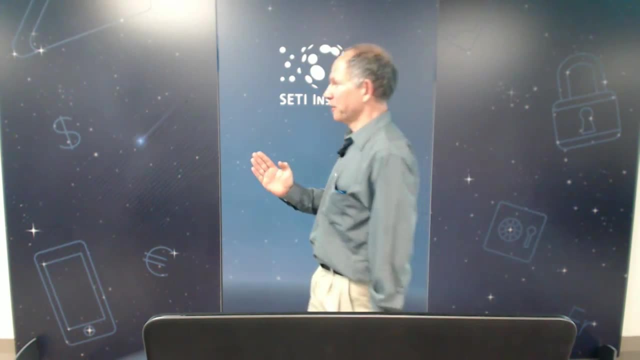 or telescopes. How many other plans are in the mix? It has been decided by the NASA administrator that one of them is going to be used for this mission, So there are no. there's no- other competition for this one Now. two were given to NASA. 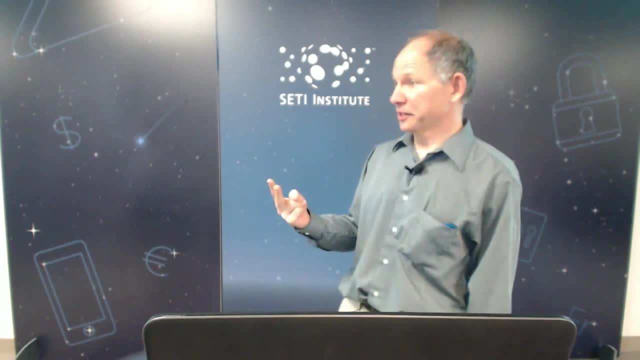 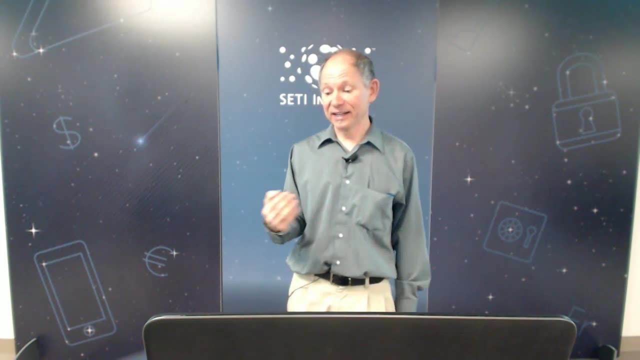 And there were some studies done, solicited for what would you do if you had a 2.4 meter telescope- in astrophysics and other fields as well, And I think NASA decided not to act on those. So I don't think. 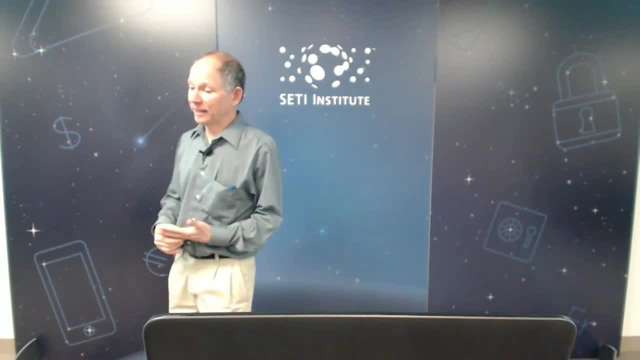 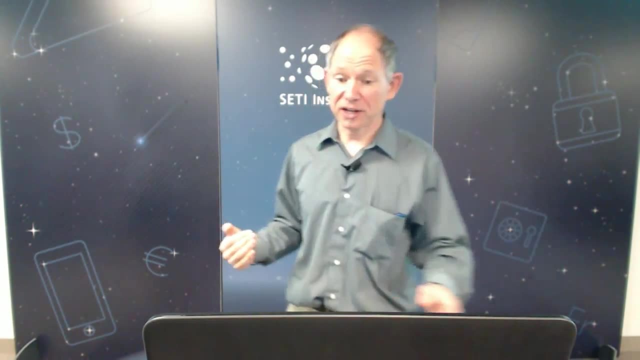 they're even really categorized, The. I think that in general NASA goes by these decadal surveys for big bucks. So if somebody were to show that you could address different science in the decadal laid out with another one of these, then I think NASA's ears. 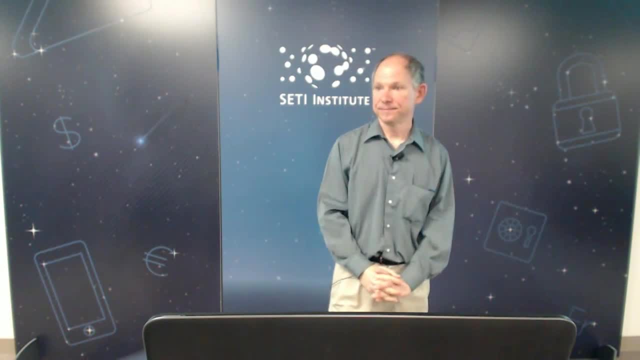 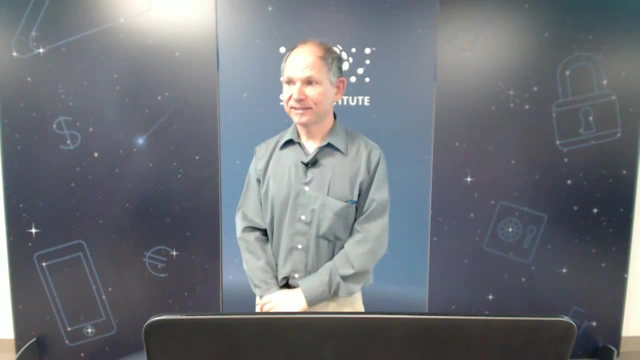 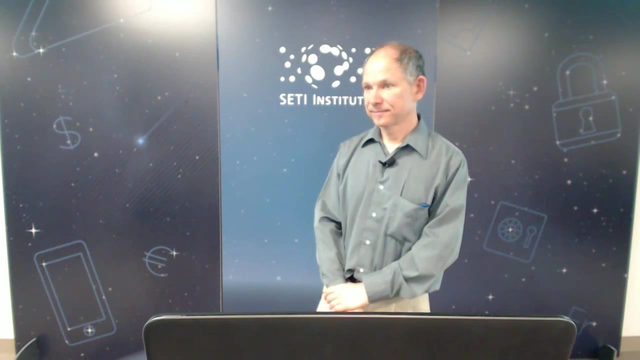 would perk up. Okay, We had a question in the back. Hey, Tom, interesting talk On the latter part of the Kepler mission. a lot of the work went into characterizing false positives and catalog completeness And my understanding is with microlensing. 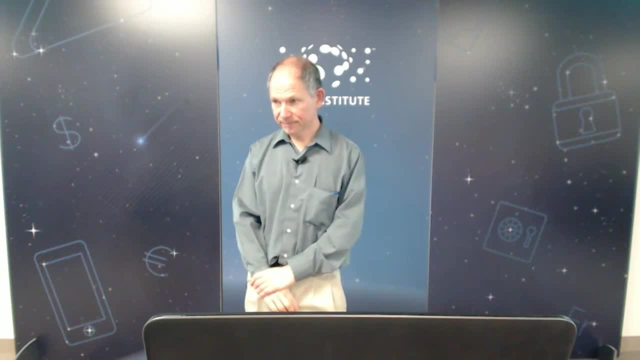 there's no follow up or repeat events, So I'm wondering what your approach is to these issues when it comes time to publish your statistics. Yeah, I'm not a real expert on microlensing, but I would think that the images themselves and the distortions. 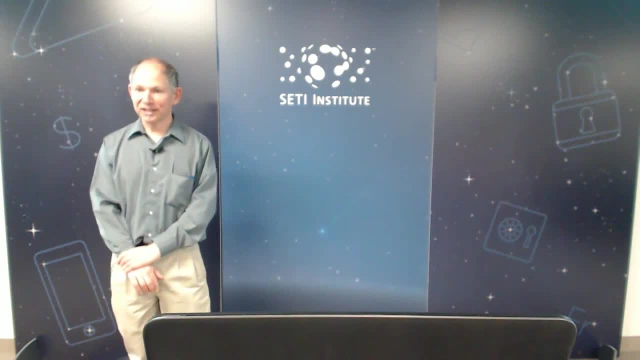 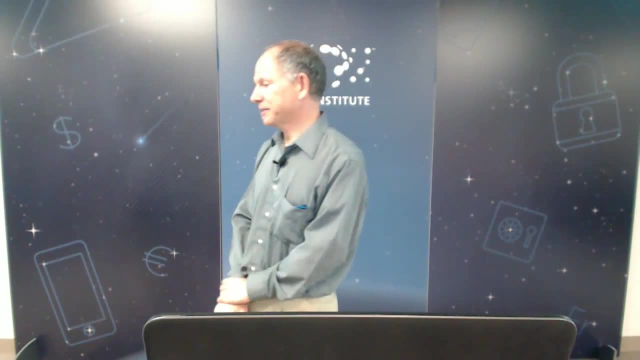 that you get are going to probably identify it as really a lensing experiment, As really a lensing event and not like a flare or something like that. And I just don't know enough about the shape profiles as to what are likely false positives and what can be ruled out. 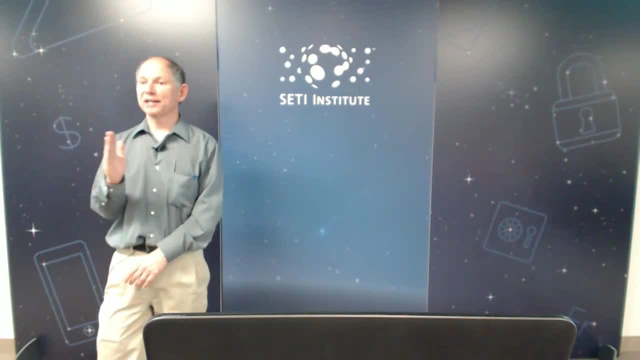 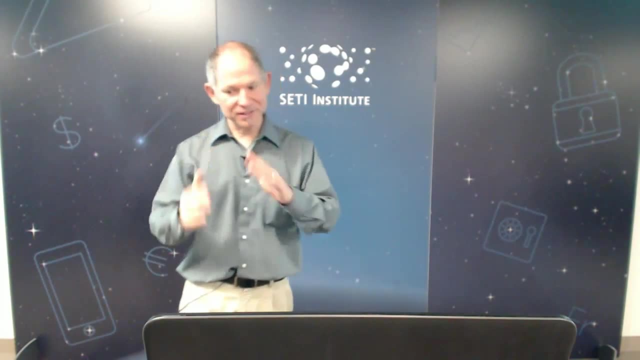 Now you know, things like binaries are probably not. that wouldn't give a false positive right, because we're sensitive to mass And so it would be different false positives from Kepler, But should probably. actually we've been thinking about having a microlensing. 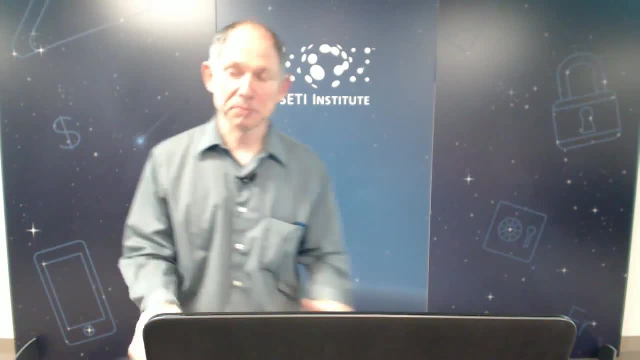 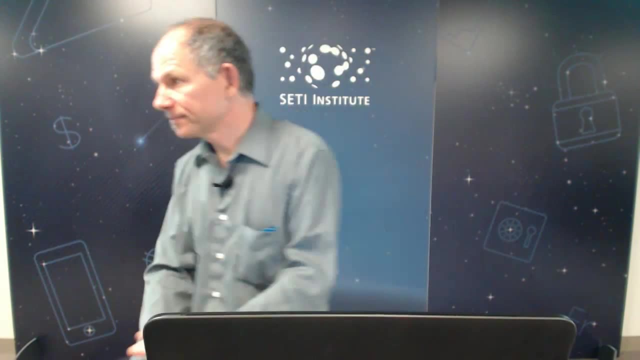 expert come and give a talk to our Bay Area exoplanet meetings to address questions like that. So just following up, if you could just say a little bit more about what you meant by extreme adaptive optics? And then a different question: is there any value? 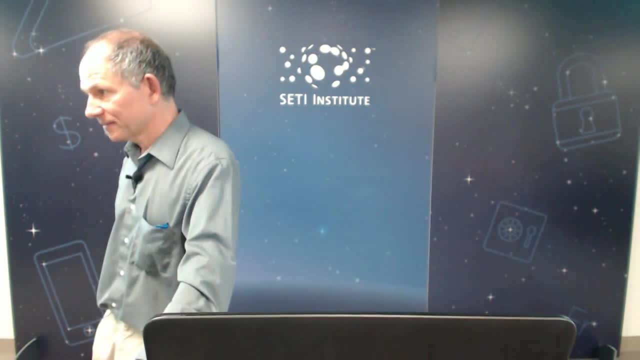 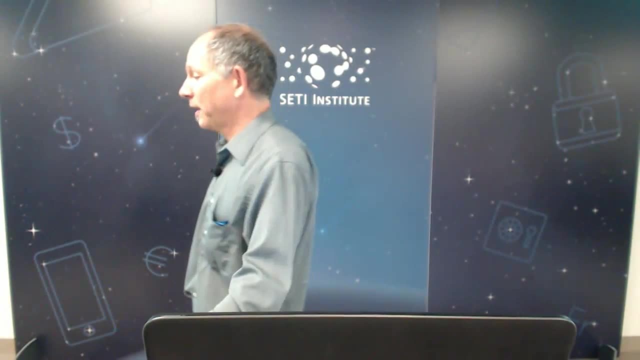 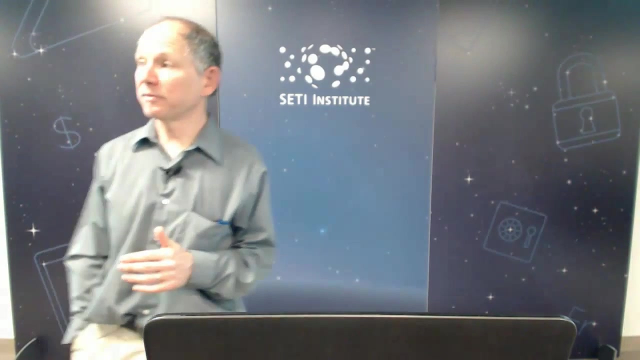 in that star shade concept flying out in front of this W first or not? Okay, extreme adaptive optics is a technique that's been developed on the ground. The first instrument that probably really uses extreme AO has just been deployed to the Gemini Observatory. This is the GPI instrument. 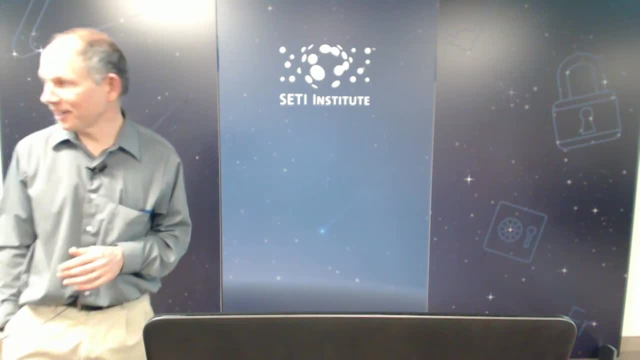 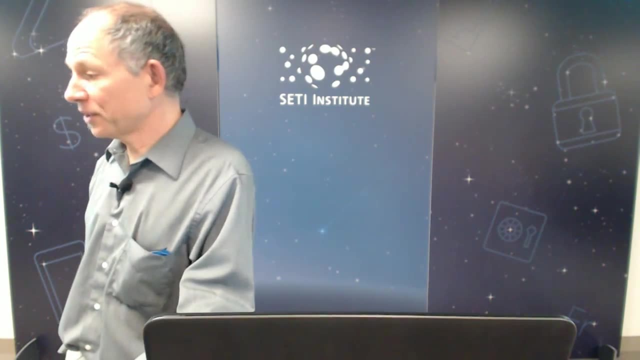 Okay And then. yeah, so people, definitely people in this community, have been working on it And you know that's where you're really trying to correct wave fronts. you know you're trying to correct faster than the atmosphere can do. 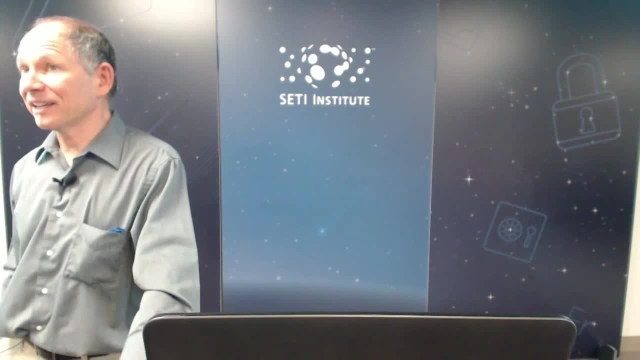 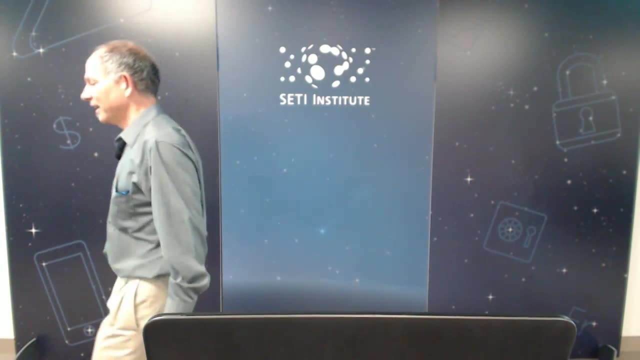 And you're not just doing a. I guess I don't technically know. I've forgotten the distinctions between, like regular AO, like on the Keck Observatory now, and a lot of the GPI stuff. But it's when you dig a specific dark hole around an object. 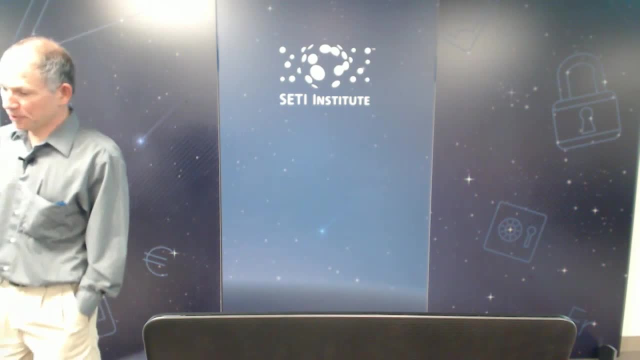 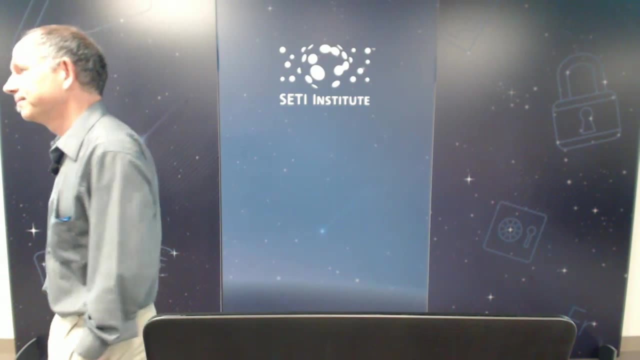 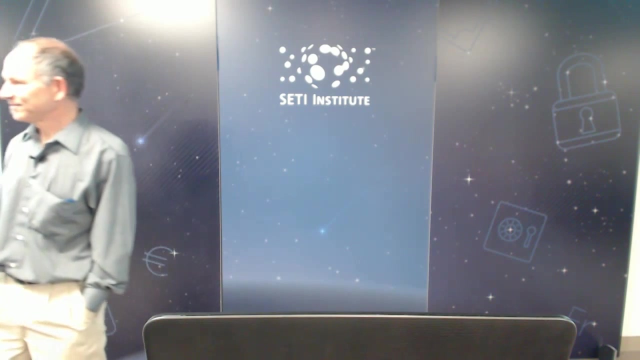 and you're trying to correct over a limited radius as opposed to just, you know, removing seeing as best as possible. Sorry, that's a terrible explanation, but yeah, yeah, What about the star shade? Oh, star shade, Yeah. 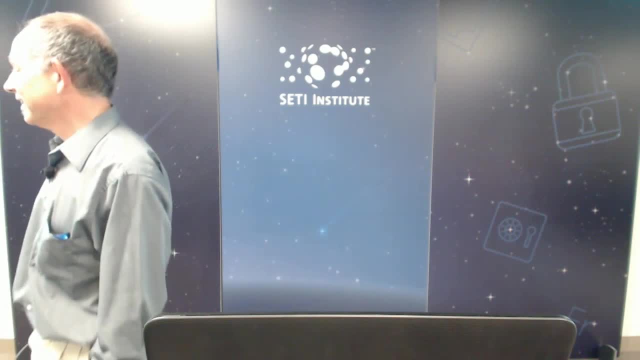 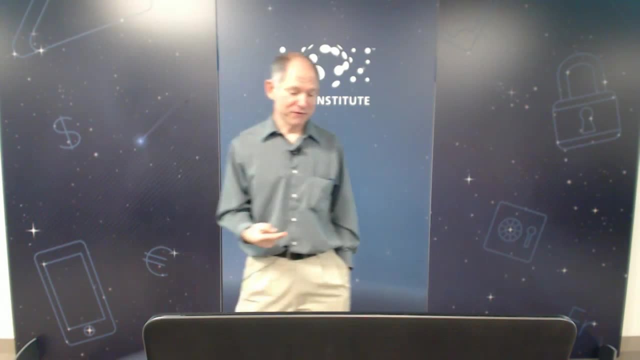 A star shade would be really great. You know it's like for people. it's an alternative to the coronagraph, very different technology. What you do is you have two spacecraft. you fly a thumb 100,000 kilometers away from your telescope. 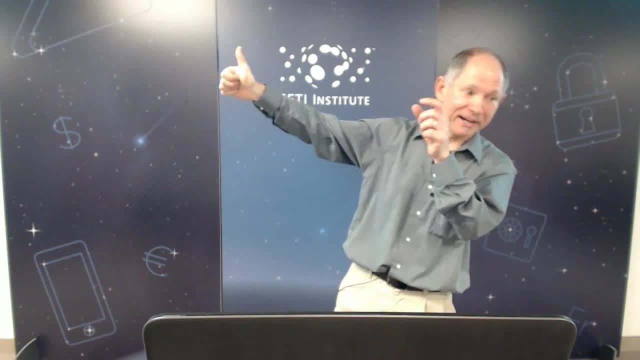 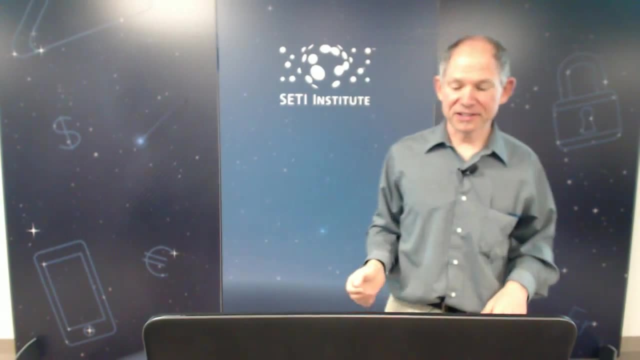 You put your thumb over the star and then you just kind of look next to it for the planet. Great, I mean, because it really breaks the degeneracies, because with the coronagraphs it's like always, that angle that you have is proportional. 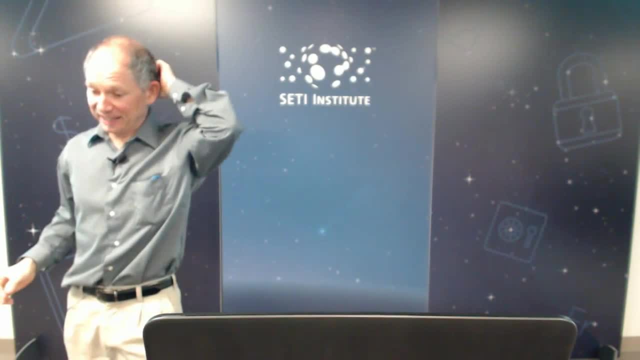 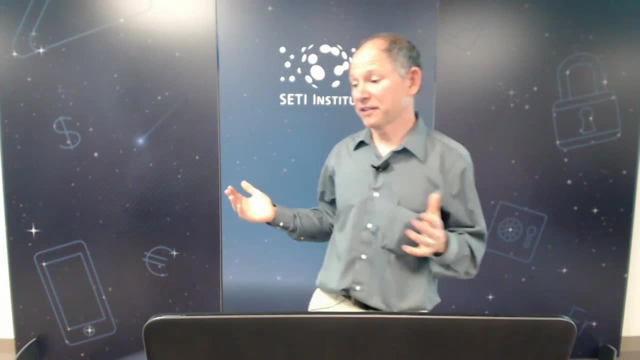 to the diameter of the telescope and there are some other things in there and you break that degeneracy. The problem is is that it just hasn't been demonstrated. You know it's like and no one's gonna. I think you're gonna need. 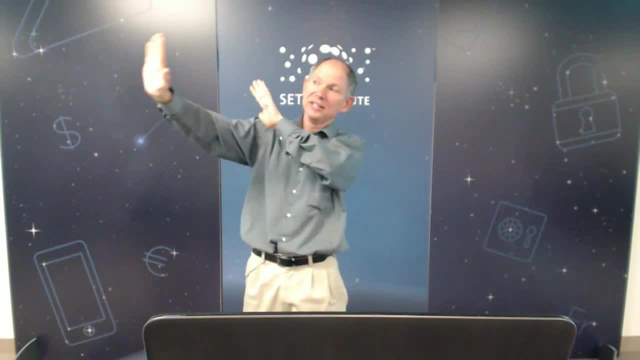 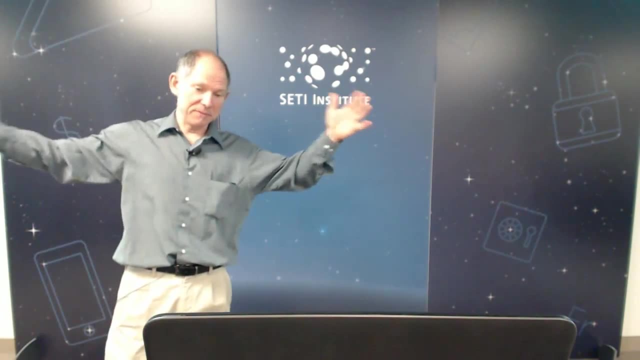 a flight demonstration, because the tolerances are just incredible. that you need to do, because you need to be able to fly these things 100,000 kilometers apart. you need to control them within you know, meters left and right. The pedals of these things. 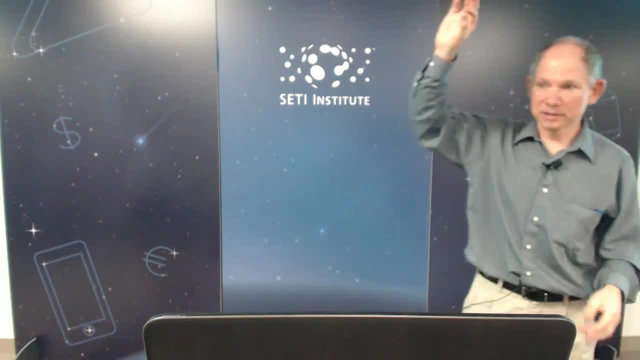 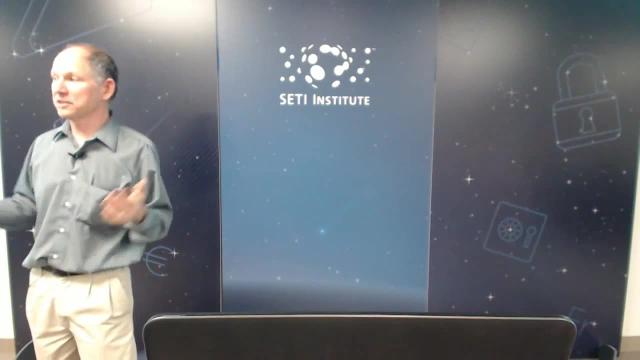 are 50 meters, They have to deploy to within, you know, and all that sort of stuff. There are a lot of studies going on, but I mean, if you get one of these things to work, yeah, yeah, that's really the way to go. 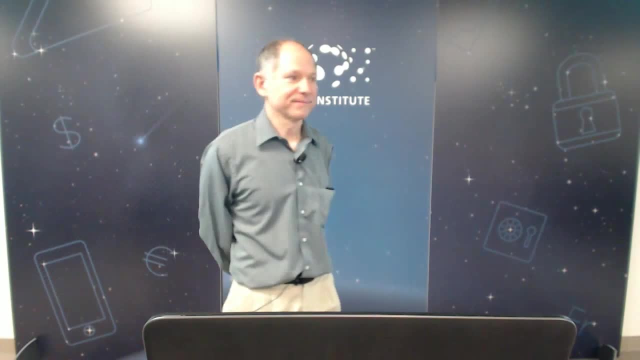 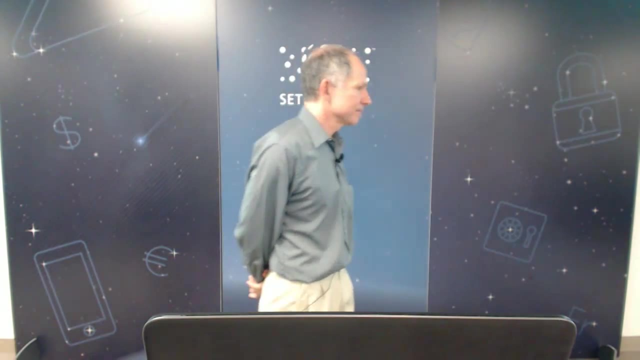 and then you can use any telescope. It doesn't have to be any kind of fancy telescope. You don't need to have this coronagraph. The microlensing over here, the microlensing survey sounds very similar to the LSST microlensing survey. 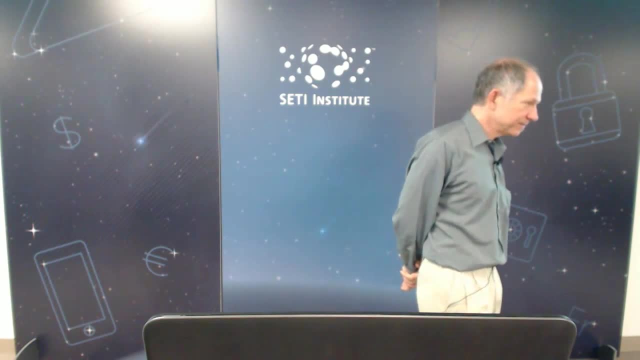 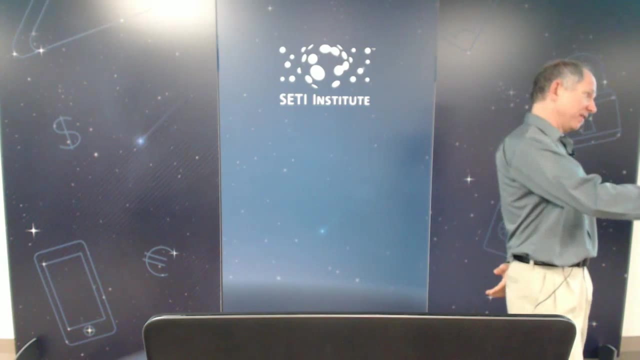 sorry, weak lensing survey. Okay, How is it complementary and how is it similar? Well, we're going to get much deeper in redshift, so be able to sample a much, a bigger volume. I think We'll be able to look. 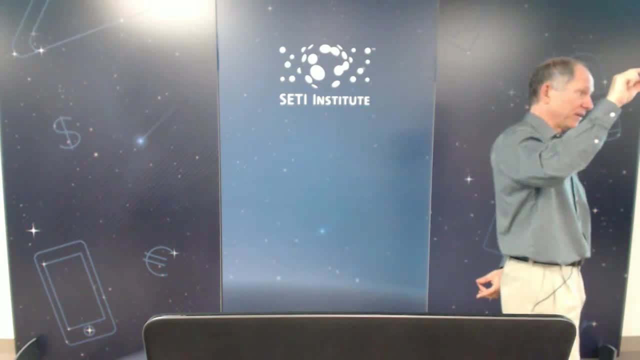 for much. we have much finer spatial resolution. You know, the native spatial resolution is like 110 milli-arc seconds here and it's seeing limited on LSST, so that's going to be like half an arc second. so I think you'll be. 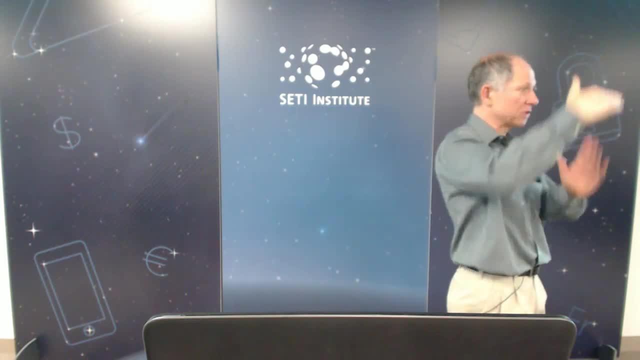 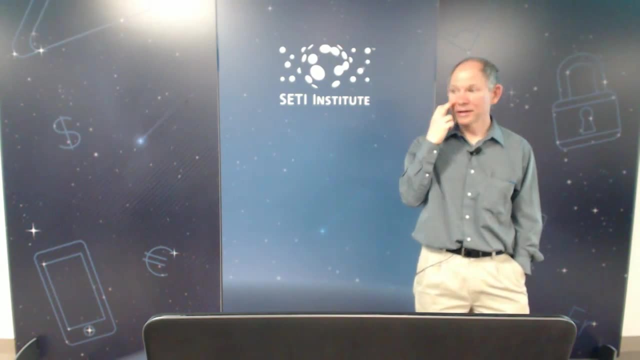 sensitive to much smaller amounts of mass. you know from distortions. I think Ken had your hand up. if you want, Hold on, hold on, Okay, Okay, yeah. well, the detectors need to be cooled or they're going to be. 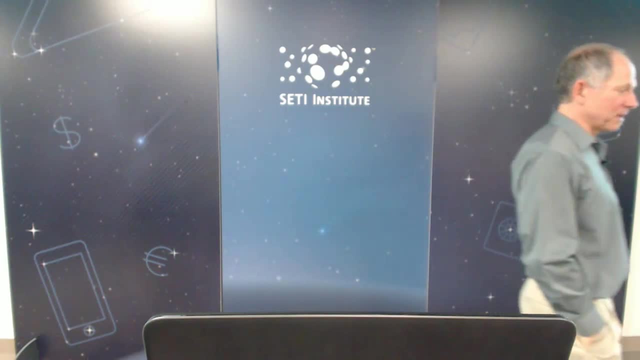 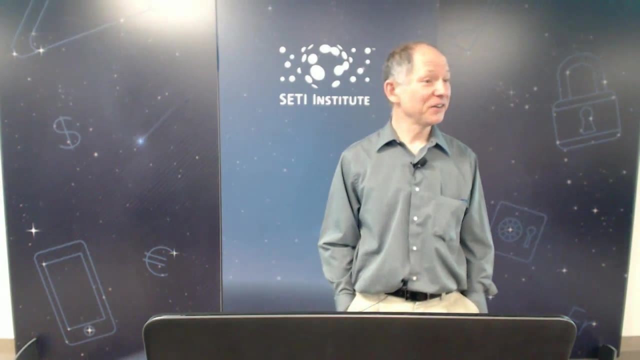 in ambient temperature. They need to be cooled, but it's going to be done passively with a radiator, so probably on the order of 110, 120 Kelvin, that sort of thing, which would be no problem. Actually, we have to heat. 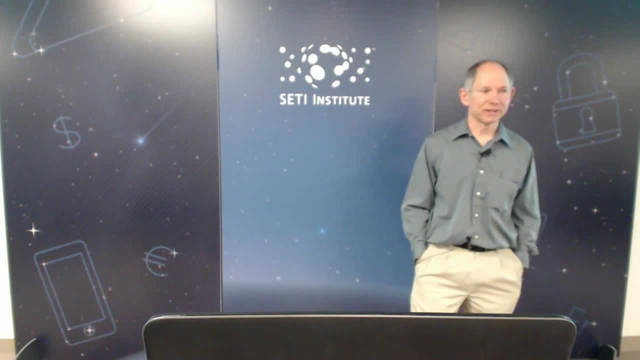 the telescope a lot and it should be no problem to keep the detectors cool. A technical question about your coronagraph optics. I mean, given this 10 to the minus ninth contrast ratio and all of those mirrors that I saw these days. 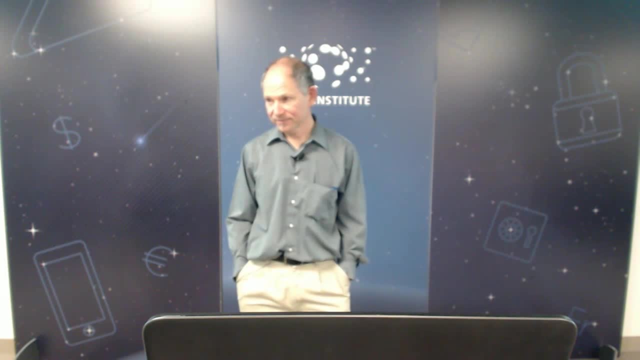 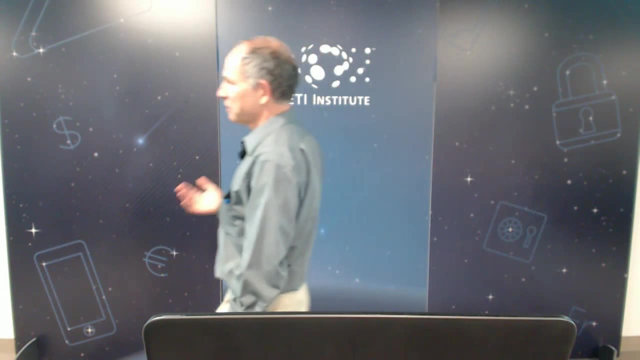 what sort of surface figures does it take to get the suppression of scattering from that and how does that compare to Hubble, for example? Yeah, well, the surface figure of these mirrors, it's okay. I think the wave front is about 50 nanometers RMS. 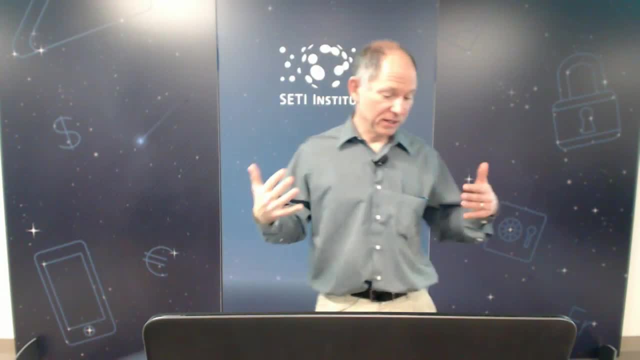 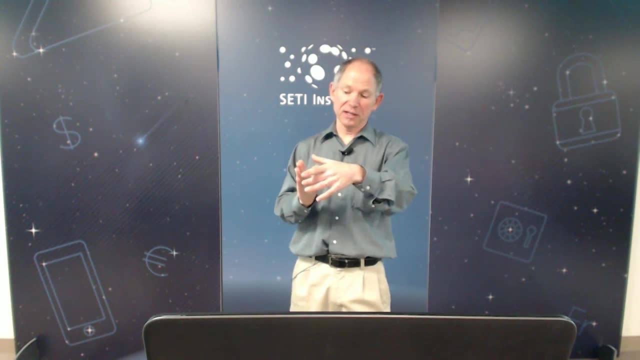 and we can live with that. but the thing is is that the key thing is having these formal mirrors where we can touch up. So what you do is you image the pupil on these formal mirrors and then each one you're pistoning by very small amounts. 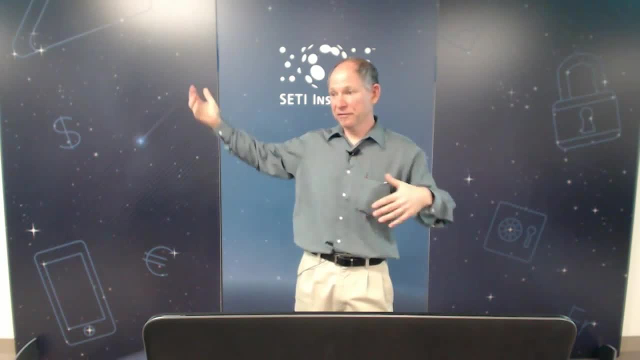 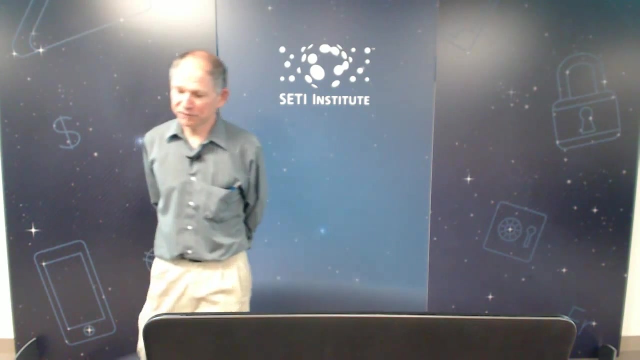 so you're correcting these moderate spatial frequency wave front errors. Surface roughness: Oh yeah, for scattered light, That's a good point. I don't think there are any particularly tough specs on surface roughness. Yeah, I don't think. 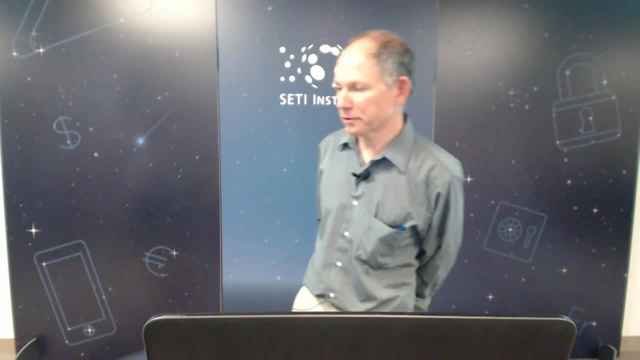 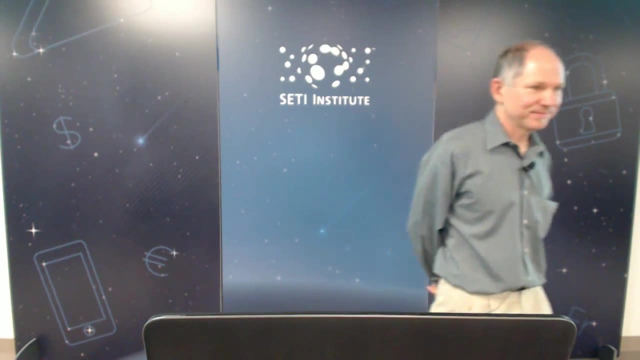 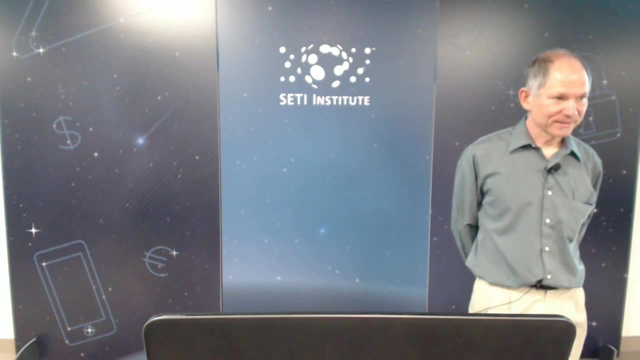 that's a big requirement. the way the chronographs work and I can hook you up with somebody in the audience who can tell you about that afterwards. Tom, it looks like that large format focal point array is going to require possibly a stretch in data transmission. 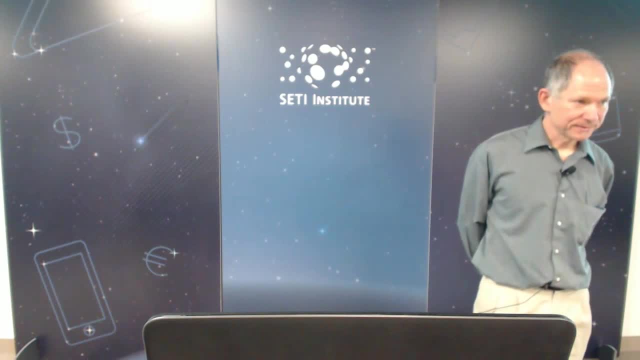 for NASA? and also, have you looked at the data analysis required for this thing? It looks huge. Yeah, it's going to take a lot of data, but it's we have to get that in place for the LSST, I mean. 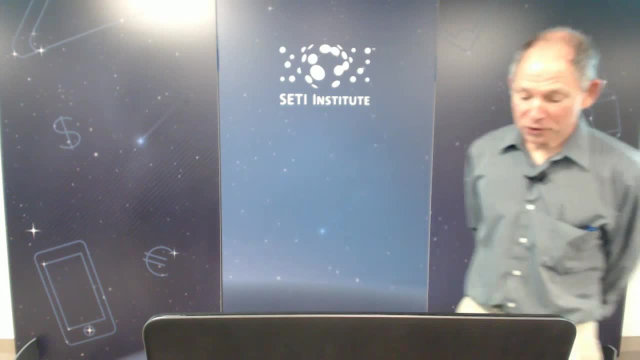 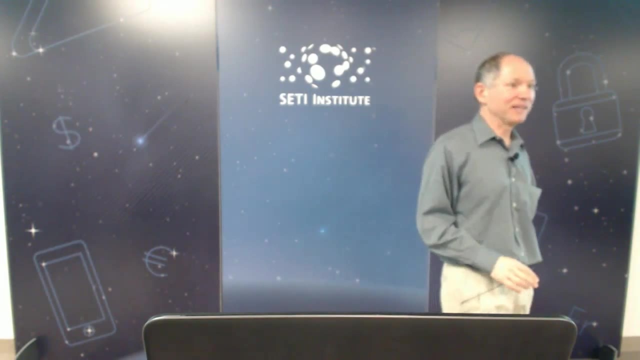 the LSST is going to observe its entire observable sky every three nights. You know it's got more. this is not a big focal plane for astronomy, you know, and Google is investing in LSST algorithms and whatnot, So you know. 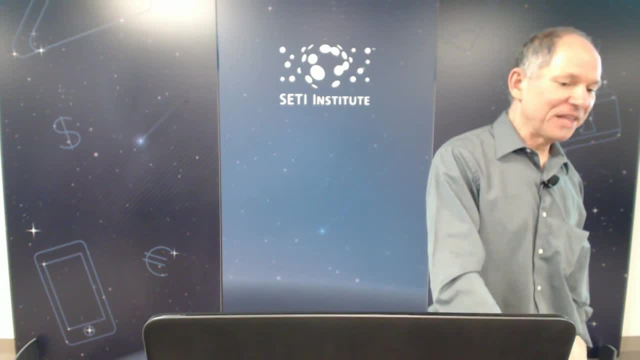 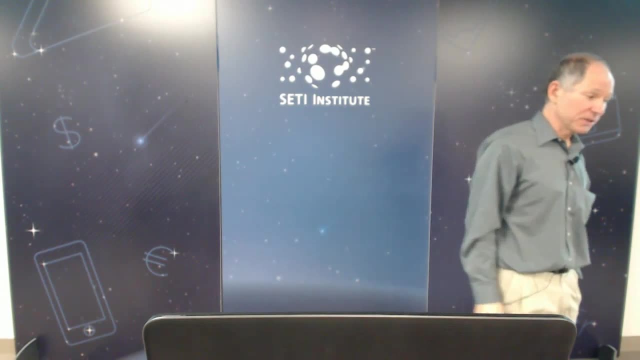 I think that that is a concern and you need to keep an eye on it, but hopefully we're not going to be able to be pushing the bleeding edge there. The comms available. we don't need to go to laser comm or anything like that. 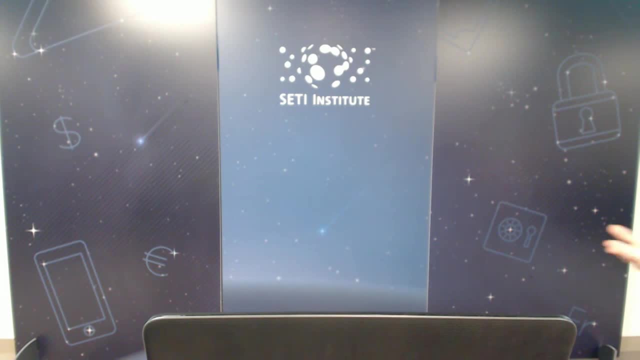 and there is commercial stuff available that fits within the budget and fits on the spacecraft and all that Going to geo orbit really helps. I mean, I think people know how to you know, get your cable signals down very, very quickly and take advantage. 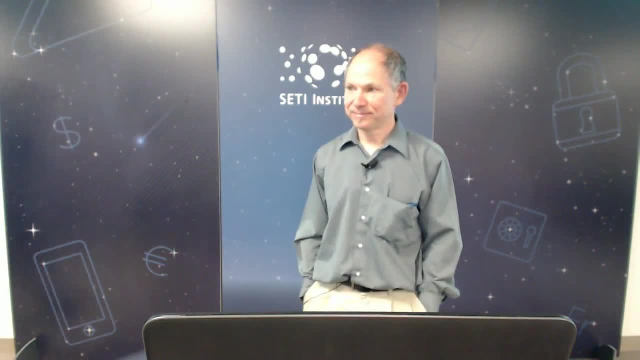 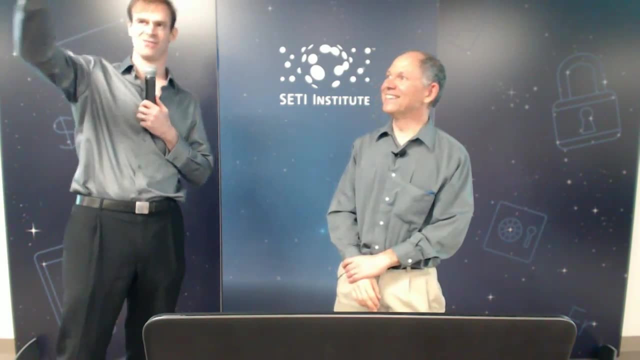 of some of that technology. Okay, no further questions, Tom. we have a special SETI mug. It's not a thumb, but maybe you can use it as a chronograph. Oh, great To block out some light at some stage. 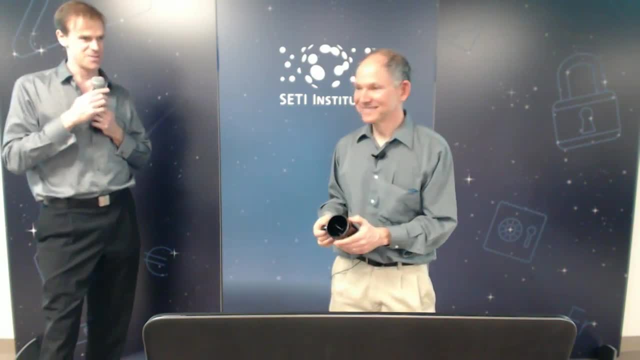 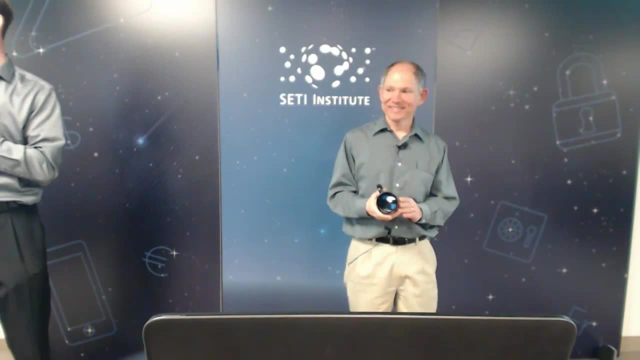 in the early of the morning when you're working on WFIRST. So please join me in thanking Tom for his great talk. Thank you, Adrian. Thank you SETI. I could probably actually accept this. This is probably less than $25. and don't tell me if it's not Great.